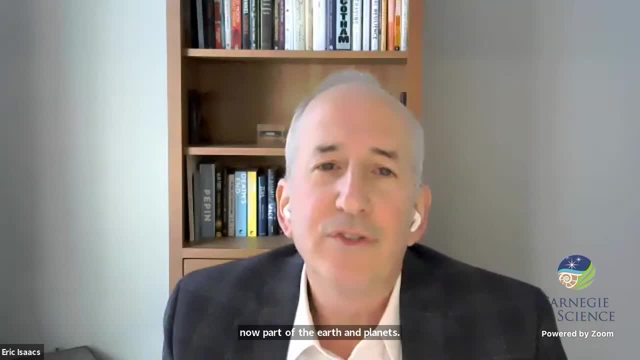 part of the Earth and Planets Laboratory. Professor Seeger is the class of 1941, Professor of Planetary Physics, Aeronautics and Astronautics at MIT. At MIT, she focuses on the discovery and characterization of exoplanets, with one of her hopes being finding an Earth-like planet. 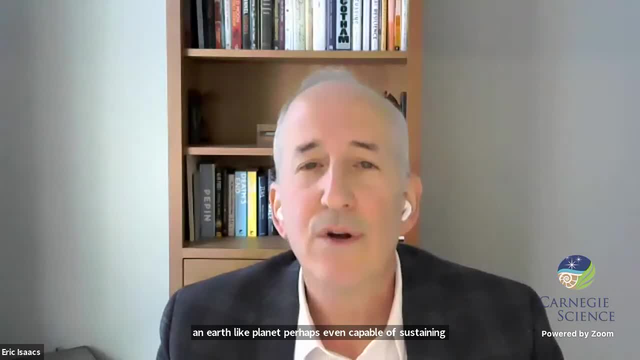 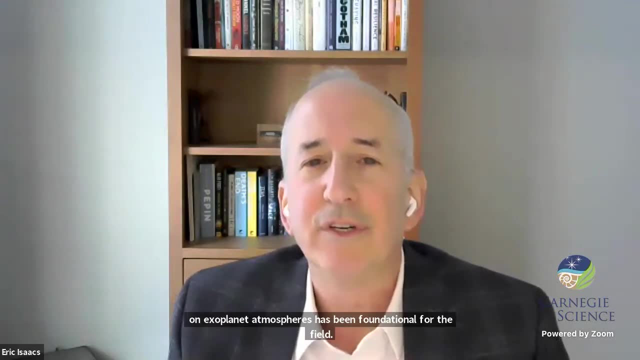 perhaps even capable of sustaining life. Her work on exoplanet atmospheres has been foundational for the field. Early in her career she posited that an exoplanet's atmosphere could be observed when that exoplanet eclipses its parent star. 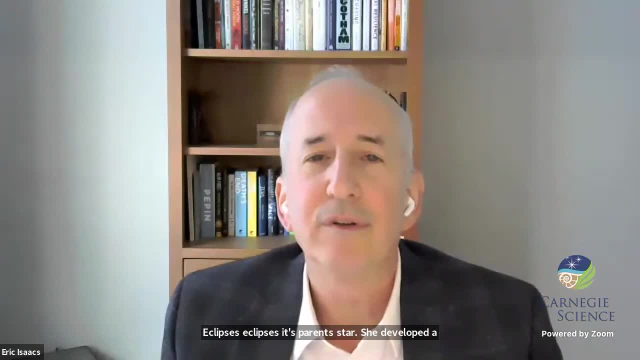 She developed a framework based on this principle that eventually enabled her to make the first detection of an exoplanet atmosphere using the Hubble Space Telescope. Now she's a leading expert in the search for signs of life on distant worlds by looking for biosignature. 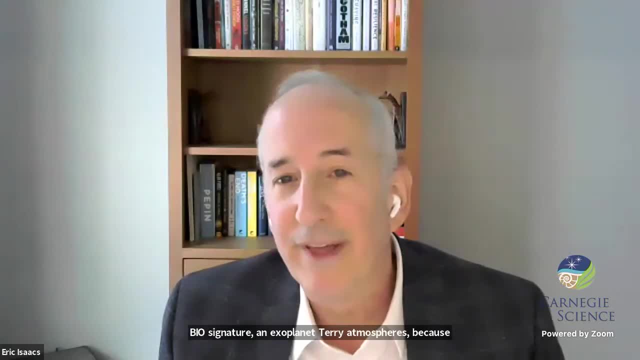 in exoplanetary atmospheres. As you know, there are thousands of planets that have been discovered orbiting distant stars- over 4,000, all of which, or many of which, have atmospheres. She is involved in several, if not many, important space experiments, including the discovery. 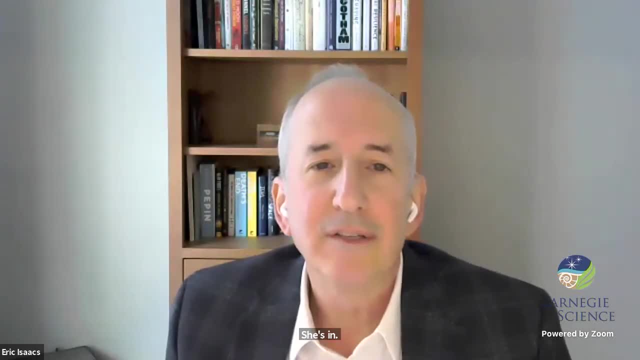 of exoplanet-based exoplanet endeavors, including leading a leading scientist for the Venus Life Binder mission. It's a concept study that's targeting signs of life on Venus and it's funded by the Breakthrough Initiatives. She serves as Deputy Science Director for NASA's Transiting. 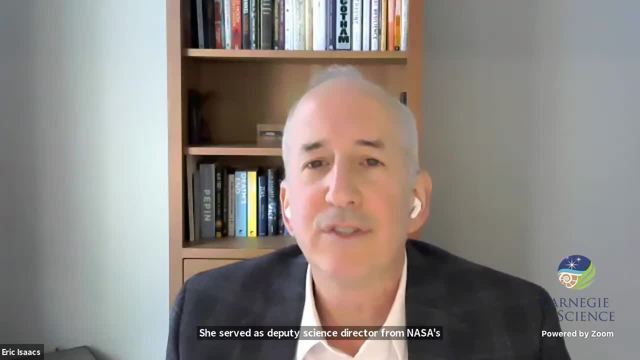 Exoplanet Survey Satellite known as TESS. It's a TESS mission satellite mission And she's the principal investigator for the JPL-MIT CubeSat Asteria, which is a prototype intended to be the first of a planned fleet of nanosatellites. 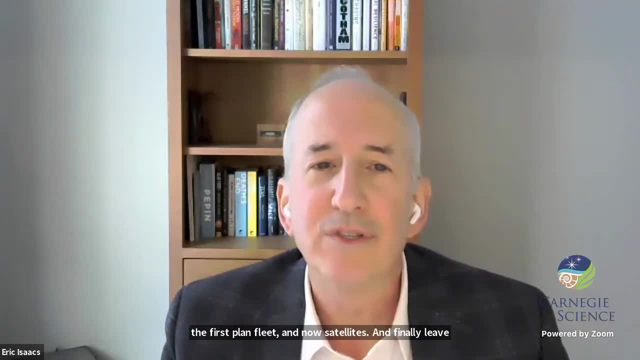 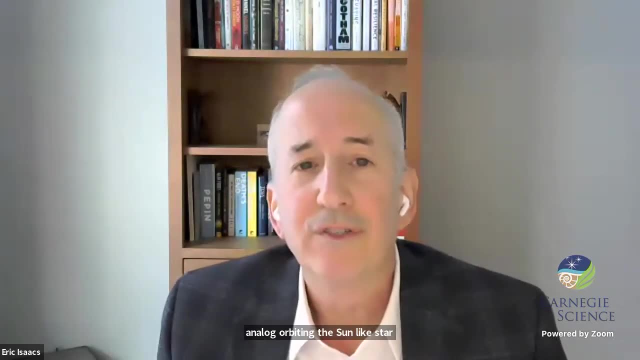 And finally, leading the Starshade Rendezvous Mission, which is under development to find a true Earth analog orbiting a sun-like star Prior to Seeger's time. at Carnegie, she spent three years at the Institute for Advanced Study in Princeton and received her PhD from Harvard University and her bachelor's degree. 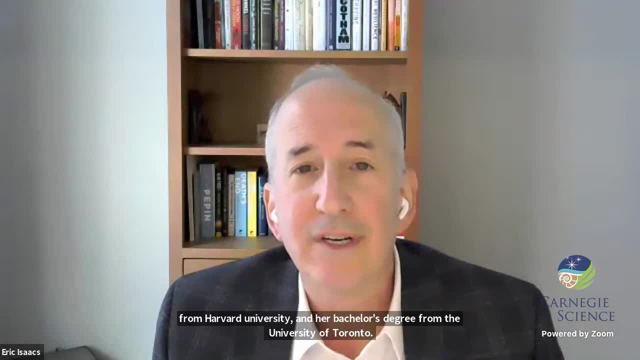 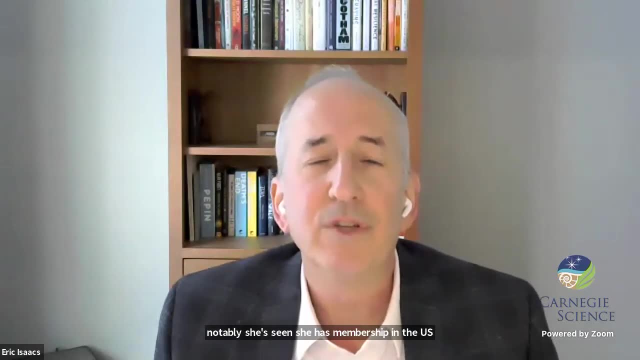 from the University of Toronto. She's received many honors. I can't mention them all here, but notably she has membership in the US National Academy of Science and membership in the 2013 US National Academy of Science and the 2013 US National Academy of Science. 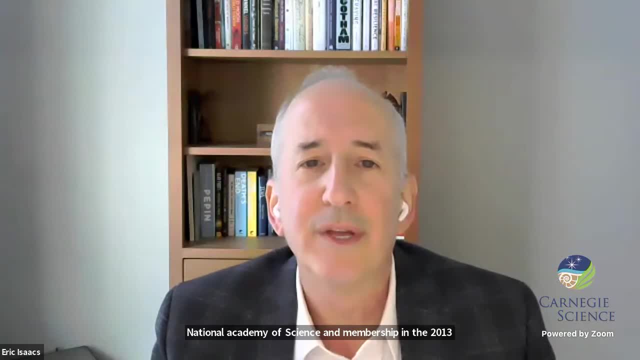 She's also a member of the US National Academy of Science and the 2013 class of MacArthur Fellows- the so-called Genius Award, So I'm very eager to hear from her today, and I'm sure you are as well, So please join. 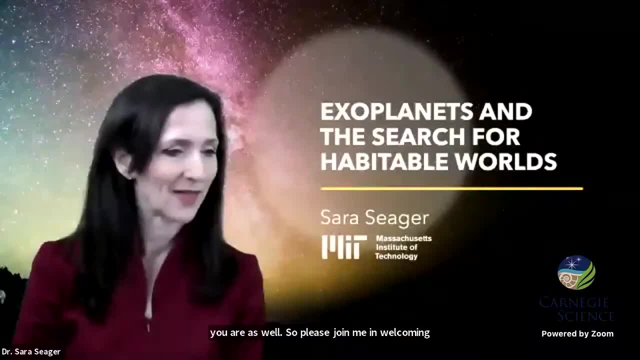 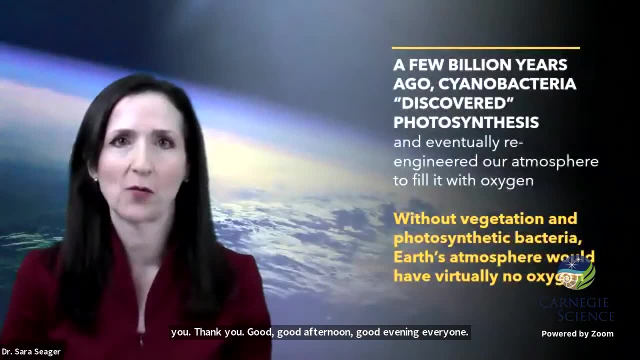 me in welcoming Professor Sarah Seeger. Sarah, Thank you, Thank you. Good afternoon, Good evening everyone. Well, to get started, I wanted to start out with the humble cyanobacteria that a few billion years ago, discovered photosynthesis: how to capture sunlight, to extract oxygen from the. 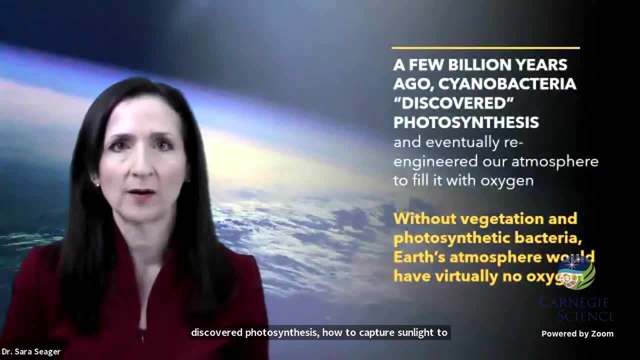 energy from the environment And a waste product. a byproduct of photosynthesis is oxygen, And these cyanobacteria unknowingly filled our atmosphere with oxygen, which eventually accumulated to 20% by volume. So today, without vegetation, without trees and plants, and 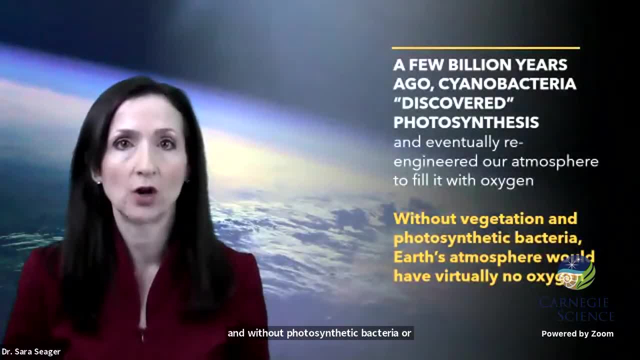 without photosynthetic bacteria, our Earth would have virtually no oxygen. So what I love to think about is intelligent aliens- unimplied aliens and intelligent aliens who are on a planet orbiting a nearby star, And if they have the kind of telescopes we're- 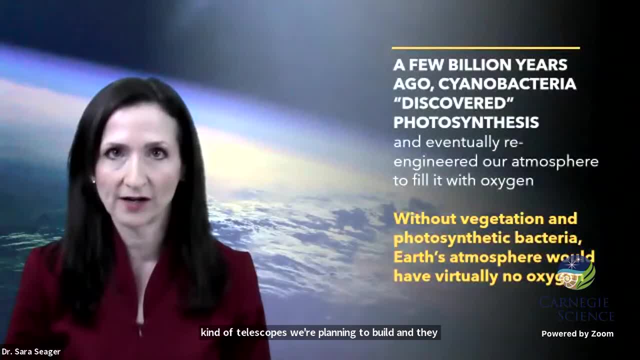 planning to build and they look back at Earth and they see oxygen in our atmosphere. they'll be highly suspicious because oxygen's a very reactive gas and shouldn't be in our atmosphere yet we have so much of it. So hopefully those aliens are out there. they're looking at us. and they suspect that there's life on our planet Earth, And that's what we're hoping to do. In the field of exoplanets, one main thread is to be able to study atmospheres of small planets and to look for gases, you know, like oxygen. 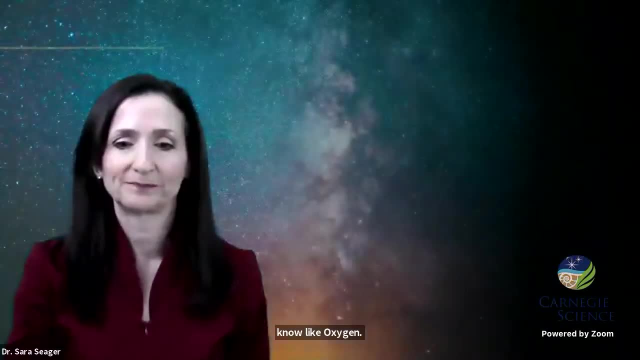 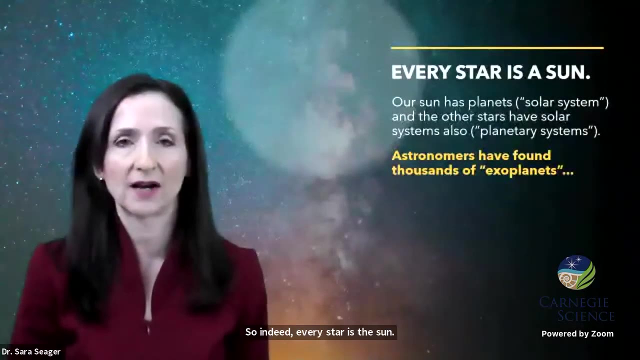 that shouldn't be in the atmosphere and to look for signs of life. So, indeed, every star is the sun, And if our sun has planets, it makes sense that other stars should have planets also, And we know of thousands of planets orbiting nearby stars and we think that pretty. 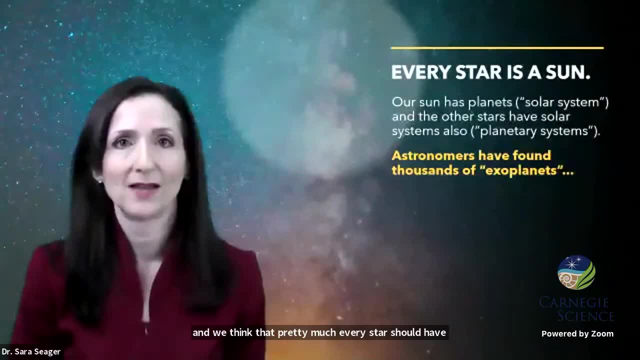 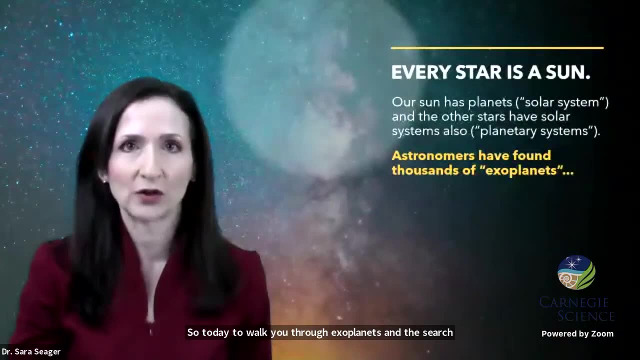 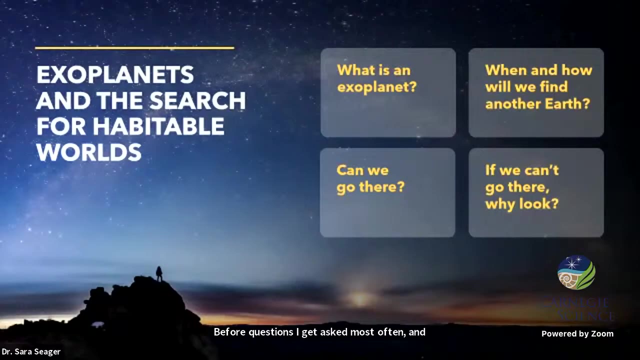 much every star should have a planetary system. So today, to walk you through exoplanets and the search for signs of life, I am going to answer for you the four questions I get asked most often. And these questions, you know, I get to ask them from people from all walks of life, not just from children or parents. 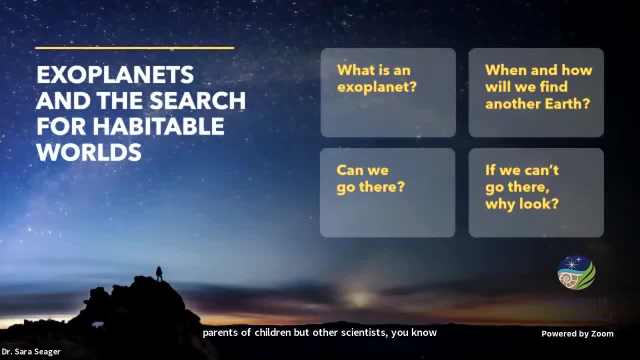 of children, but other scientists, you know, people I meet on the airplane or just anywhere. really, I mean, it's amazing how these questions come up over and over again. There's a lot of questions that I get asked, actually most often out of all these, and I'll let you think. 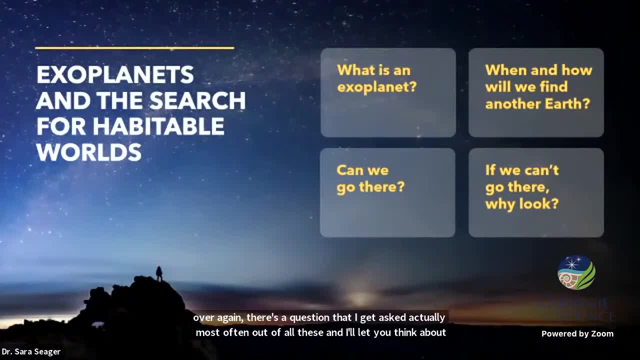 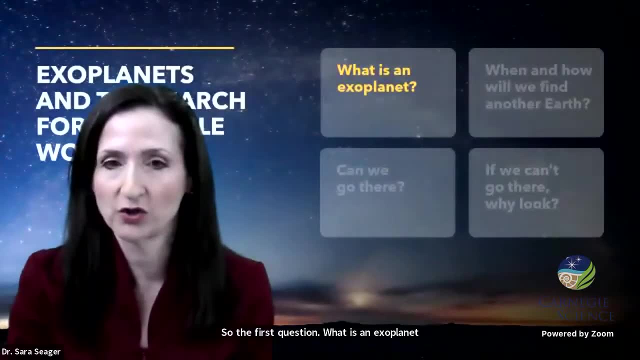 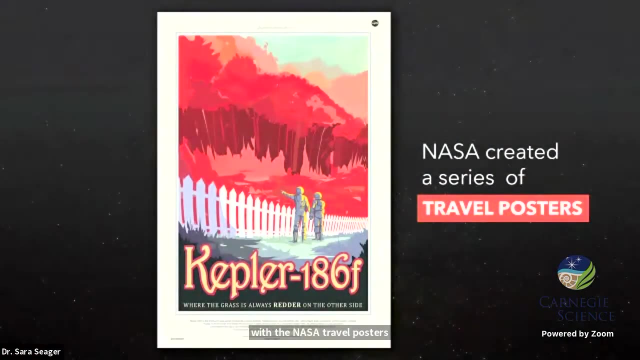 about which one that is, and I'll tell you when we get there. So the first question: what is an exoplanet? Well, a fun way to start to answer this question is with the NASA travel posters You can see. here's one of them. It says Kepler-186f. where. 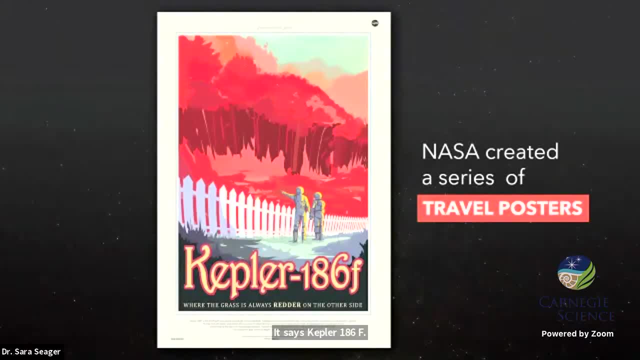 the grass is always redder on the other side. Now we can't travel to another exoplanet, but it's fun to try to imagine what these planets might be like. And here you see, the artist has made the trees red. Kepler-186, the host star, is a small red dwarf star. 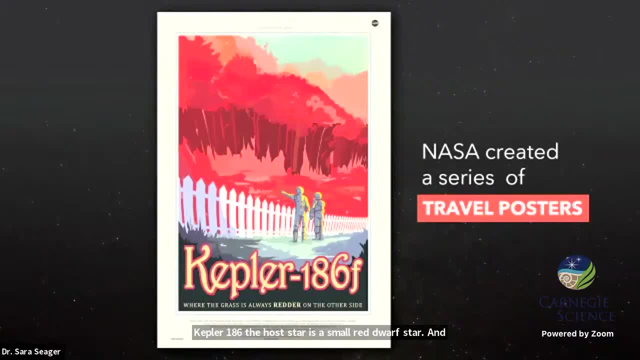 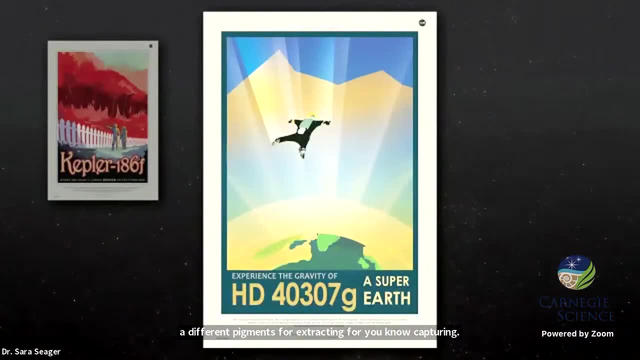 And so people are imagining that the life there might have different pigments for extracting, for capturing energy from the star Experience the gravity of HD40307g- super earth, And here the artist is imagining A person who's going to parachute on a planet with a higher gravity than we have here on. 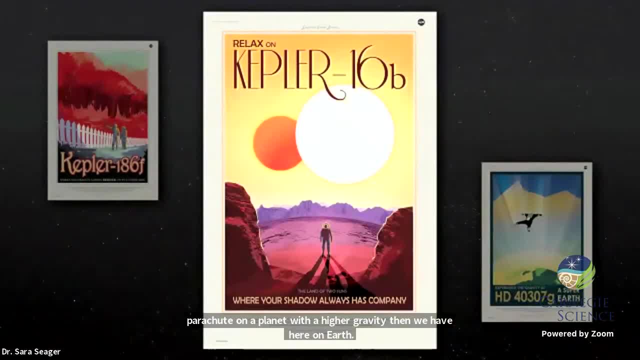 Earth. Relax on Kepler-16b, the land of two suns, where your shadow always has company, Because there are some planets that orbit two suns. We call them circumbinary planets. And yeah, it would be really different on a planet like that: There'd be two shadows. 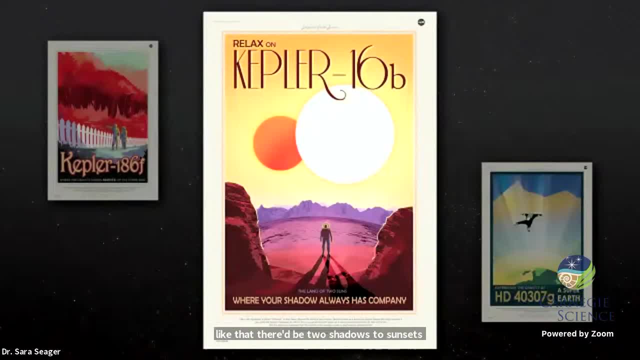 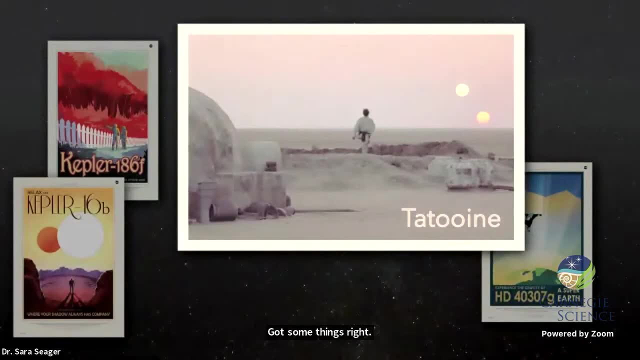 two sunsets, And I love to say that science fiction got some things right. Here's Tatooine, a planet from Star Wars, where there are two suns. So Tatooine was a circumbinary planet. Now we don't know much about the exoplanets. 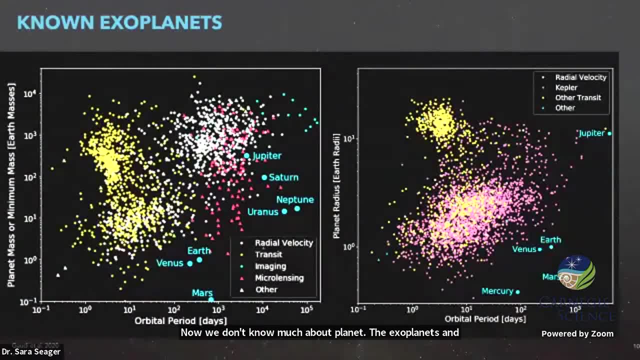 in detail, but we know that there are a lot of them and that the planets have incredible diversity in their mass and size and orbit. Now, you don't have to understand this plot to understand the rest of the talk, But I wanted to put a few quantitative things out. 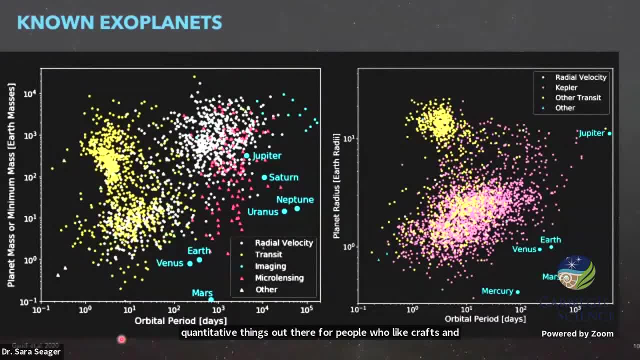 there for people who like gravity. Let's talk about this plot on the left side. It's showing you a planet mass as a function of planet orbital period or year in days, And each one of these points on the plot is a different planet. So you know, your first takeaway can be: wow, there are a lot of planets. 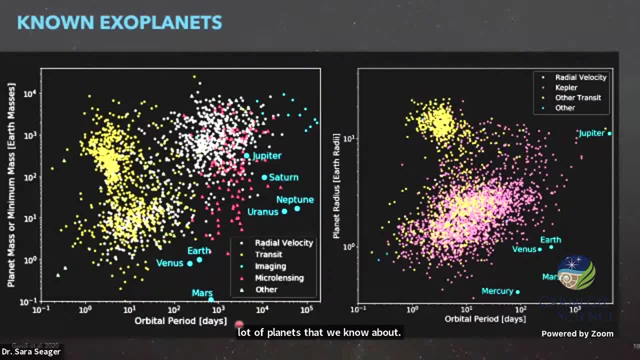 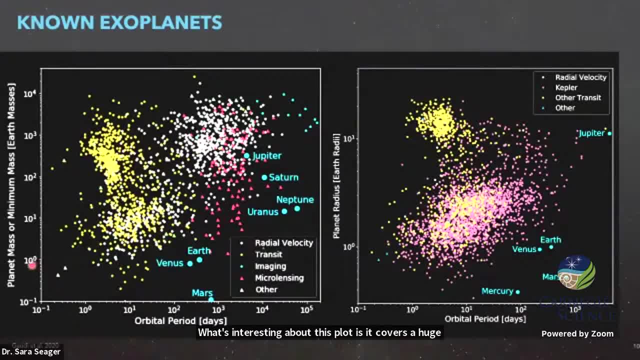 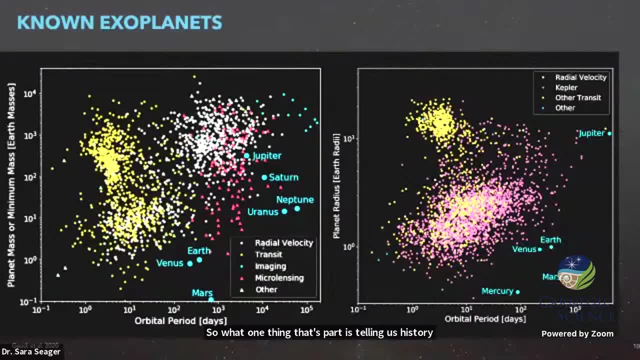 one thing this plot is telling us: it's trying to capture all of the really interesting planets out there. There are some planets, for example, that are our Earth size, are smaller than Earth mass, or smaller than Earth mass whose years- the time that it takes the planet to go around. 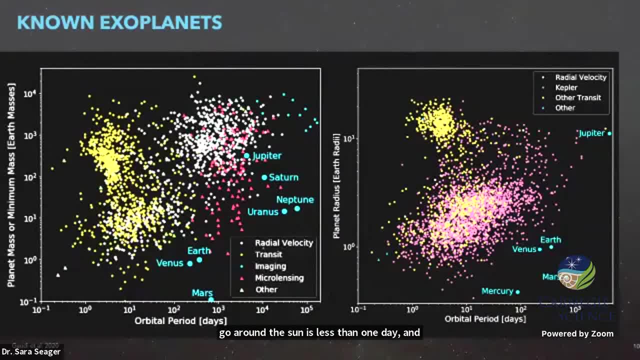 is less than one day, And these planets are so close to their star, based on Kepler's third law, that their surfaces are hot enough to melt rock And we think they have lava lakes just from heating from the host star. There are some planets that are so big- they're far too big- for us to. 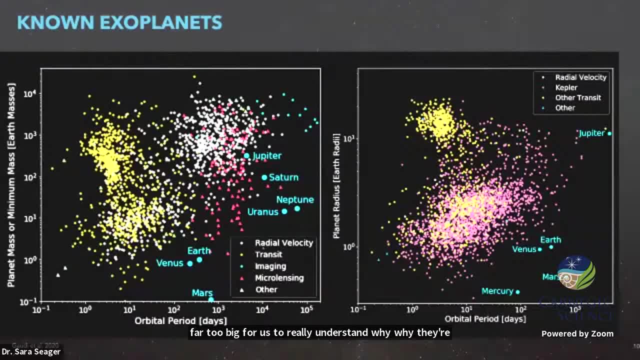 really understand why they're so big. There's actually a whole bunch of planets. They're two to three times the size of Earth And we call them mini Neptunes because they're smaller than Neptune, which is about four times the size of Earth, And these planets have no solar system. 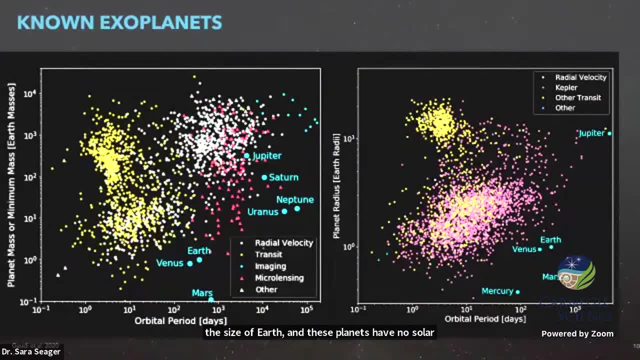 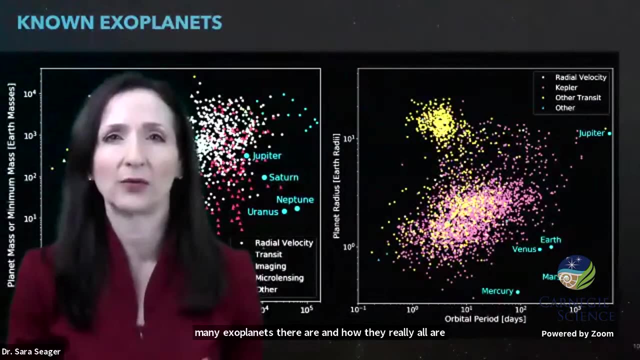 counterpart, yet they appear to be the most common type of planet in our galaxy. So I haven't done this justice in any way. I just wanted to show you this slide so you could just see how many exoplanets there are and how they really all are very spread out when we think about their mass. 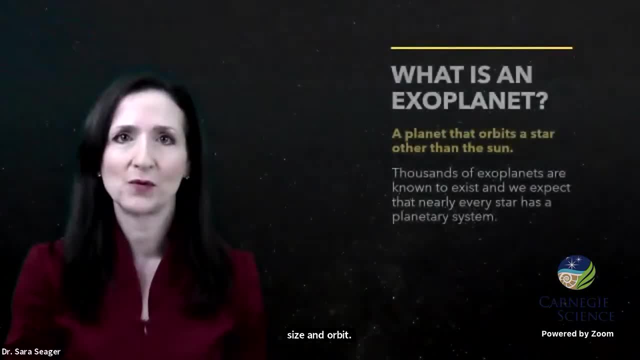 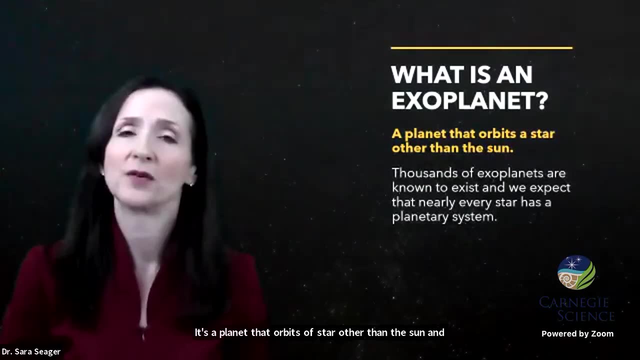 and size in orbit. So what is an exoplanet? It's a planet that orbits a star other than the sun And, as I already said, there are thousands of them that we know and we expect that every star has a planetary system. 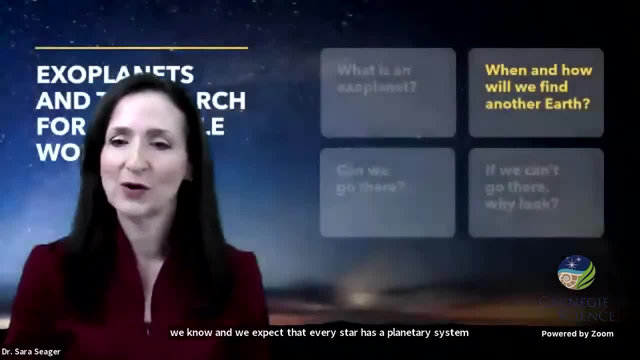 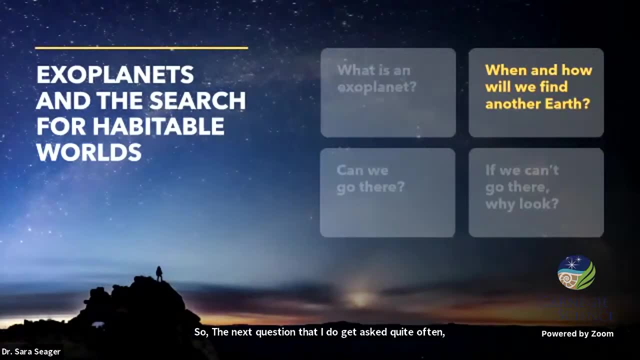 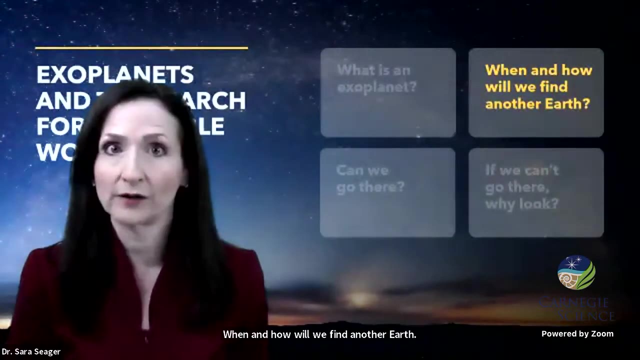 nearly every star. So the next question that I do get off quite often it's cuts to the chase: When and how will we find another Earth? Because there are all these interesting planets out there, but only some of them. And to answer that question, I just wanted to start by telling you that our own Earth at some 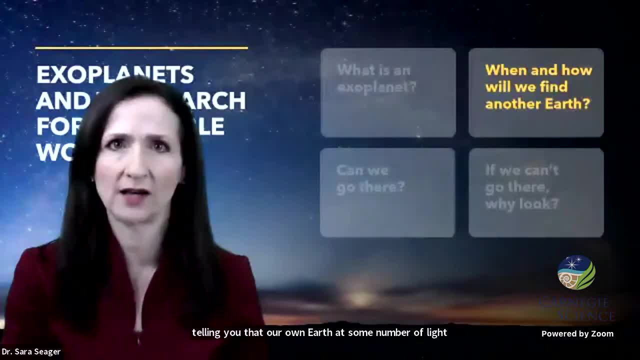 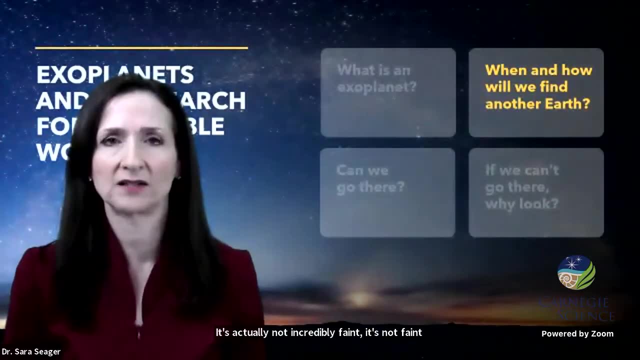 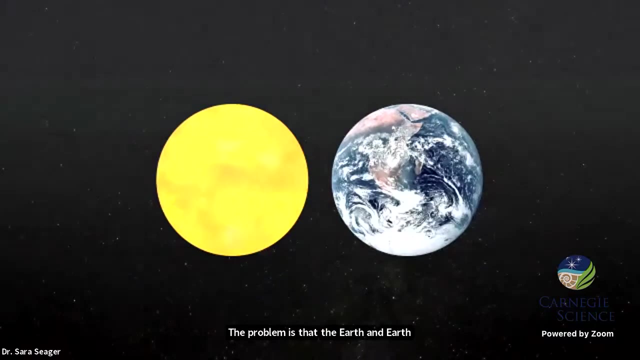 number of light years away, say 10 light years, 20 light years, 30 light years- a planet just like Earth. it's actually not incredibly faint. It's not fainter than, say, the faintest galaxies ever observed by the Hubble Space Telescope. The problem is that the Earth, an Earth-like planet, 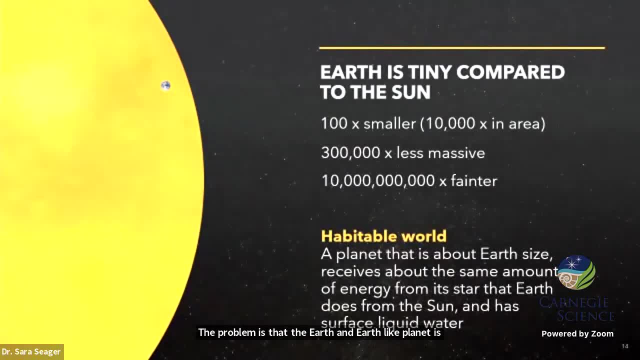 is next to a sun-like star And, at least for our Earth and sun, the comparison is just outrageous. Our Earth is really tiny. Our Earth is 100 times smaller than our sun And our Earth is 300,000 times less massive. Our Earth is also 10 billion times fainter than our sun. So if I was with you and I 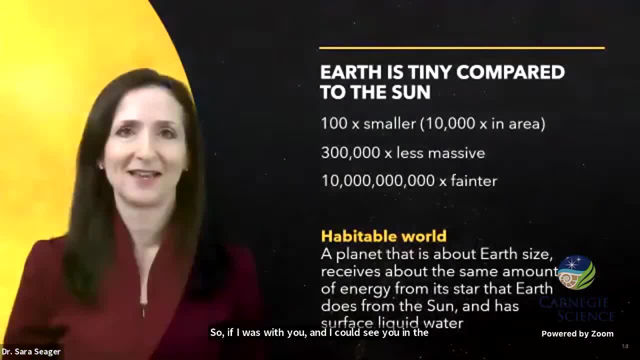 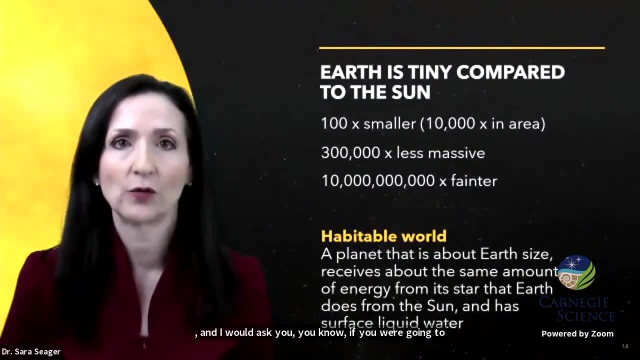 could see you in the audience, I would literally ask for a show of hands. And I would ask you- you know, if you were going to drop everything, take a sabbatical on exoplanets to find another Earth, which method would you choose? 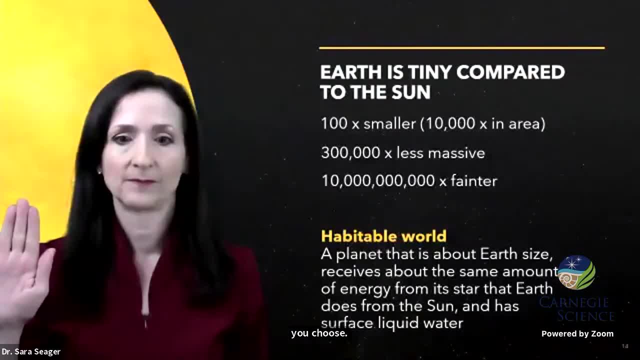 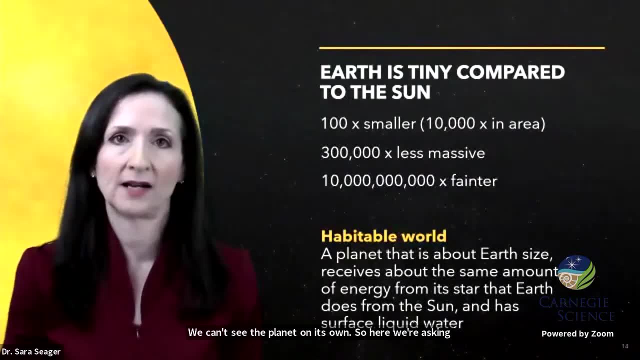 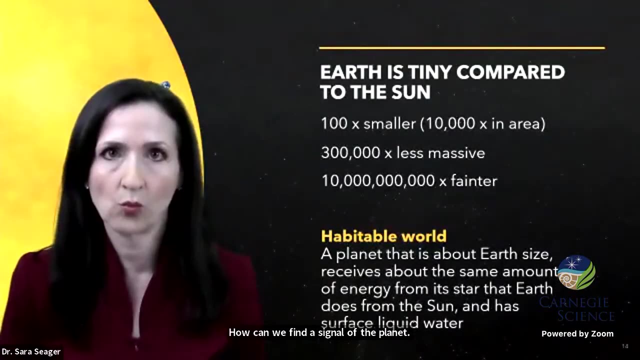 Would you choose a method that involves planet size? We can't see the planet on its own, So here we're asking: how can we find a signal of the planet right next to the big, bright, massive star? And in this case, you'd have to work on a technique. 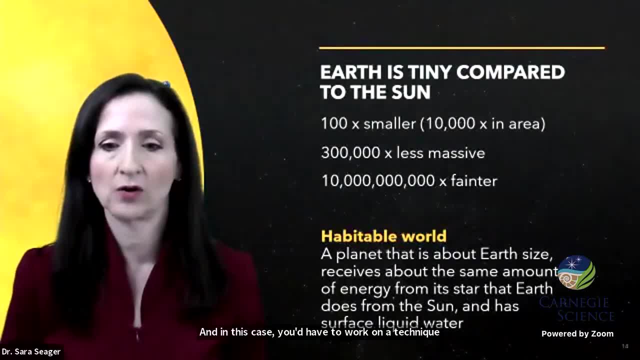 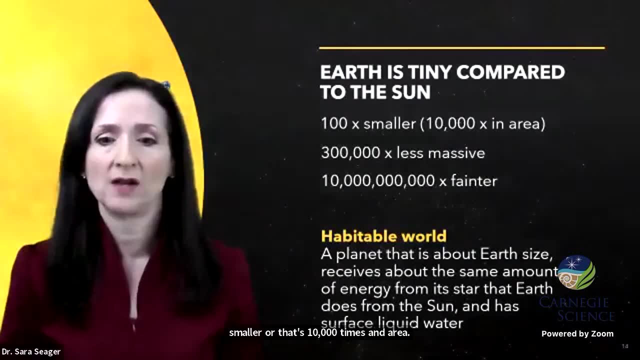 where you'd be able to find a planet that's 100 times smaller or that's 10,000 times an area. Or would you choose to work on planet mass? Here it looks like an even harder problem, because our Earth is 300,000 times less massive than our sun. Or would you choose to work on 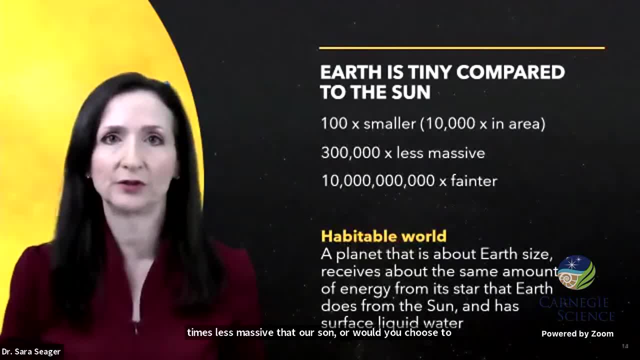 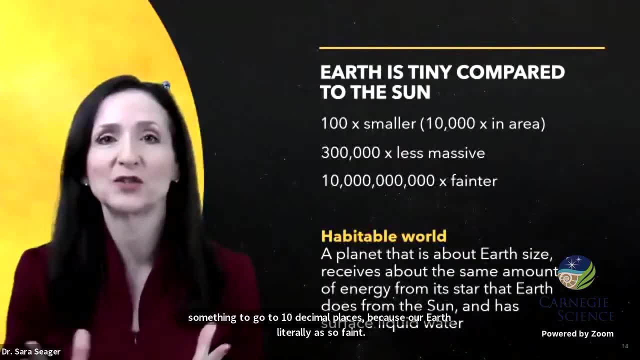 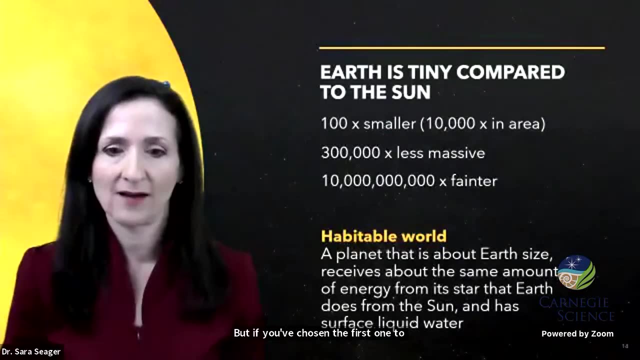 a method that requires you to be able to build something to go to 10 decimal places, Because our Earth literally is so faint. Well, I can't see you and I don't know which one you've chosen, But if you've chosen the first one to find a planet by its relative size, then you're. 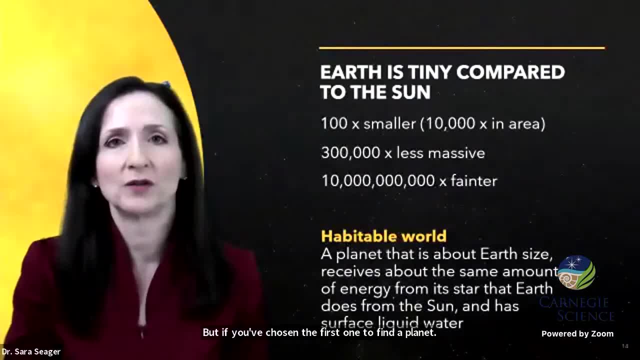 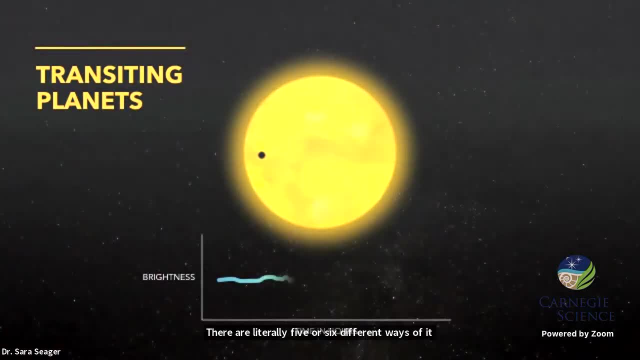 size compared to its star, then you have chosen the most common way that we find new exoplanets. today. There are literally five or six different ways to find planets, but here I'm focusing on what we call transiting planets. These are planets that go in front of the star, as seen from the 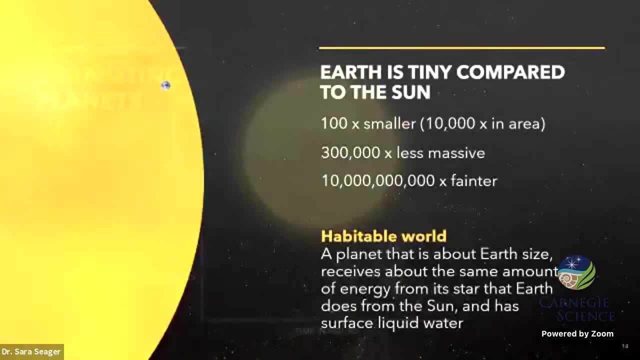 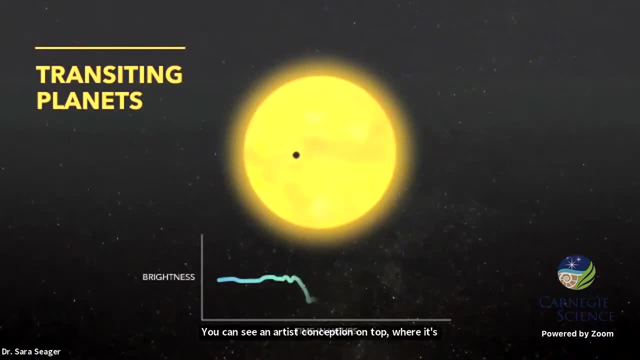 telescope, And I'm just going to run that animation one more time. You can see an artist's conception on top, where it's showing you a fake planet going in front of a fake star, And on the bottom you're seeing what we actually measure. We can measure the brightness of a star as a function. 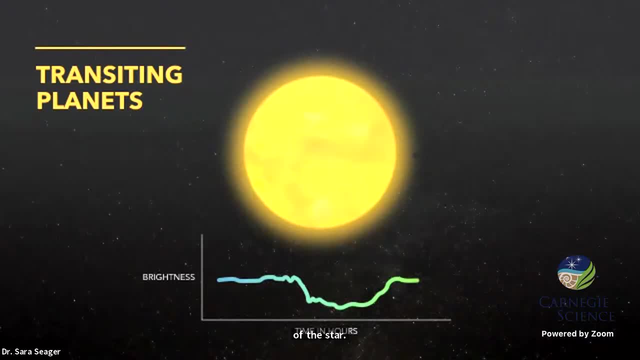 of time And we can look for a tiny drop in brightness if there just happens to be a planet going in front of the star. Now, a planet that transits is actually quite rare, because the planet might not be going in front of the star, Its orbit might not be aligned in such a way that transit. 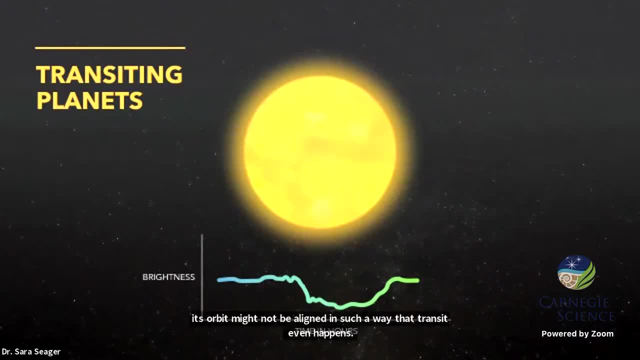 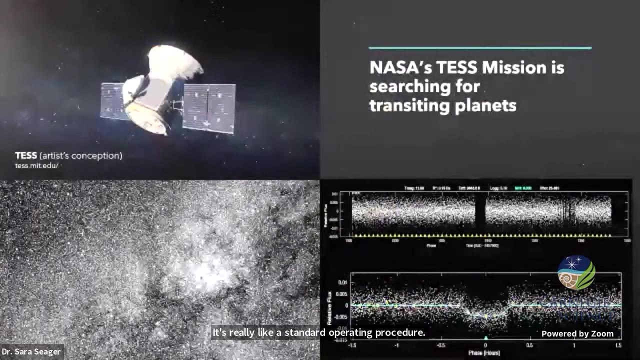 even happens. But I wanted you to know that this method of finding planets by the little drop in brightness, It's a very well-established technique. It's really like a standard operating procedure And one of our we have a mission. it's an MIT-led NASA mission called TESS, like the girl's name, TESS. 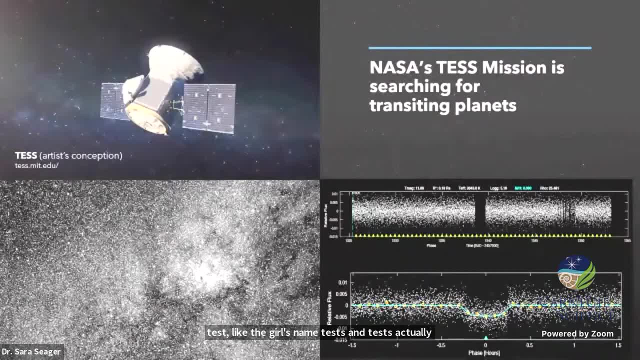 And TESS actually orbits Earth in a very highly elliptical, highly inclined orbit And it steers at one giant strip of the sky for a month. The strip is. for people who know what this means it's like. imagine the conversation. It's like I'm going to go to the moon, I'm going to go to the. 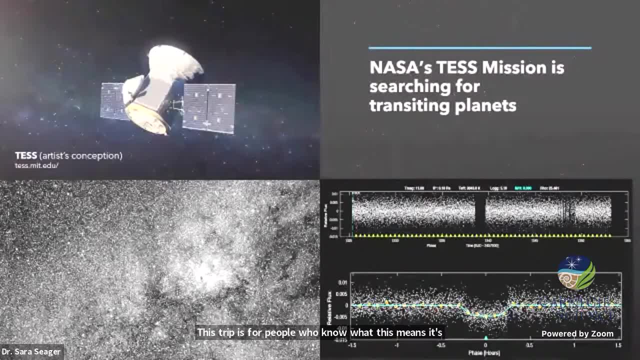 stars and see which one of the stars will be the largest star, and then in a month I bring out a whole entire million star. that's basically essentially three in one, petits involving millions of stars. So here's two of these stars and one is a half moon at night. Yeah, more or less. And what does TESS mean to you? You're going to go to the moon, Okay. So what it actually does is what we're asking to do, which is, when you look at stars, you're going to. 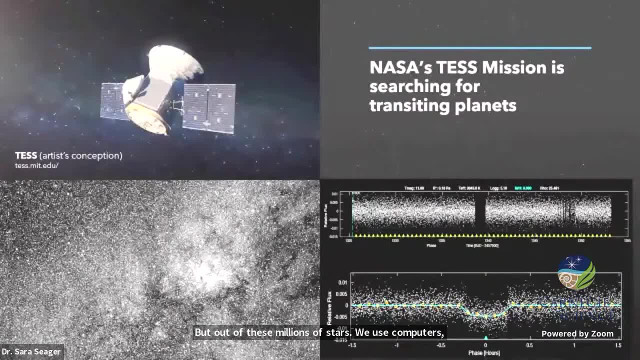 computers, big computer programs developed by NASA. Some of them are developed by the MIT team and others, And what these programs do is they figure out where each star is and then they look in a catalog, if the star is known already, and to find you know position for the star. And then 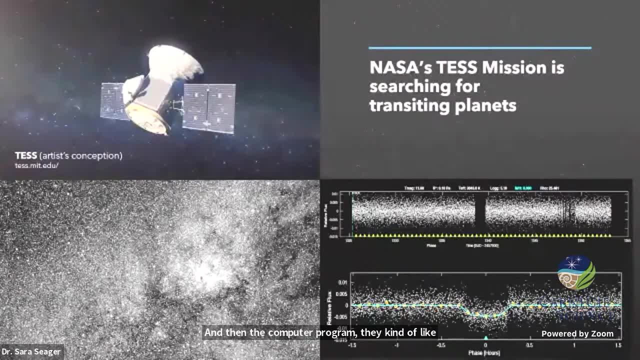 the computer program. they kind of like plunk down a circle around each star- Sometimes it's a different shape- And then they measure, they count the brightness of each star And the programs do this frame by frame until they can construct a time series And what you're seeing on the bottom, 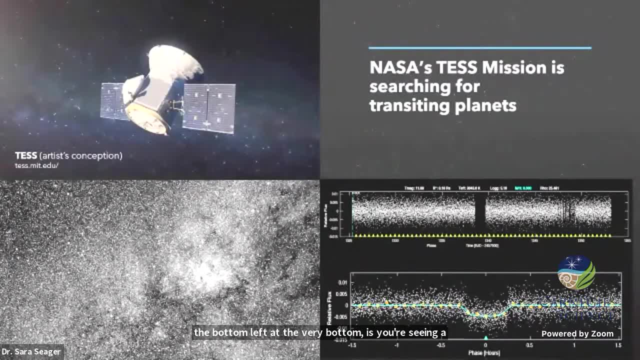 left, at the very bottom, is you're seeing a transit light curve. It's real data from the test mission And you can see the dots, all the dots. the little dots are points of brightness that the computer program has extracted, And then the program searches these millions of star light. 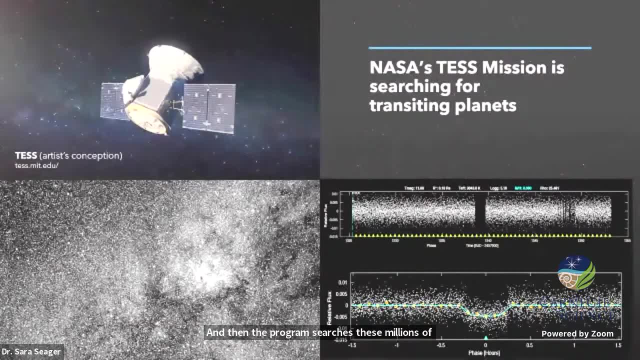 curves, looking for a drop in brightness. that's a very characteristic shape And after all that hard work, we're left with a bunch of planet candidates that, believed or not, a human team works through. a human team ends up looking at like what the 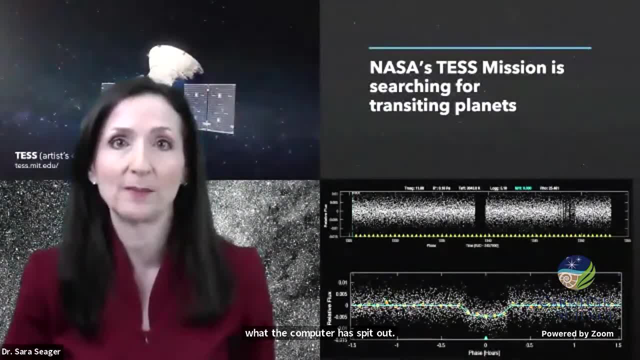 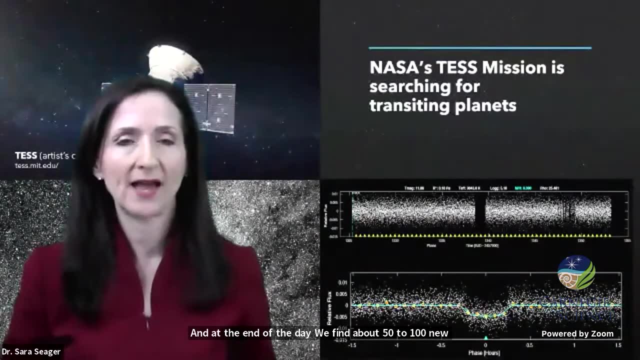 computer has spit out, typically searching a few hundred objects every month And at the end of the day we find about 50 to a hundred new planet candidates each month. And these planet candidates go out to the community for extensive follow-up observations to confirm whether or not they are. 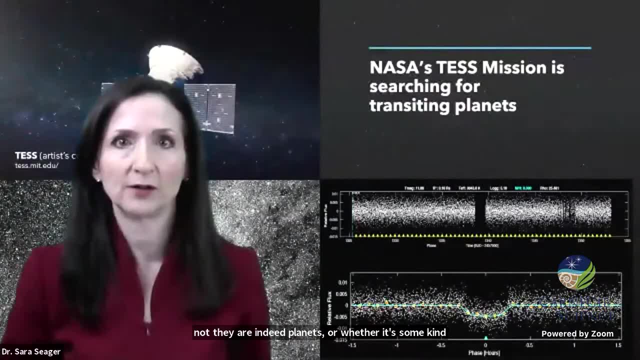 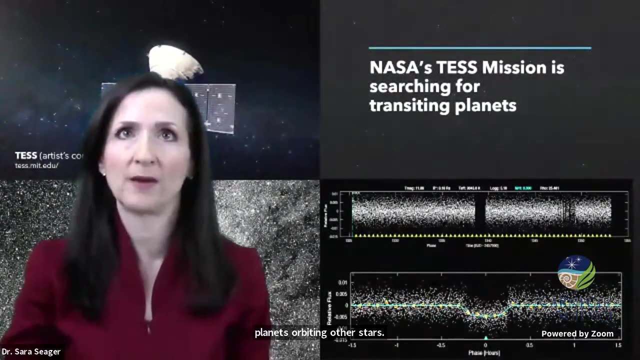 indeed planets, or whether it's some kind of false positive signal. So in the search for another earth, the transit method is really right out there in front to finding small planets orbiting other stars. But in exoplanets, you know, there's a big push to make. 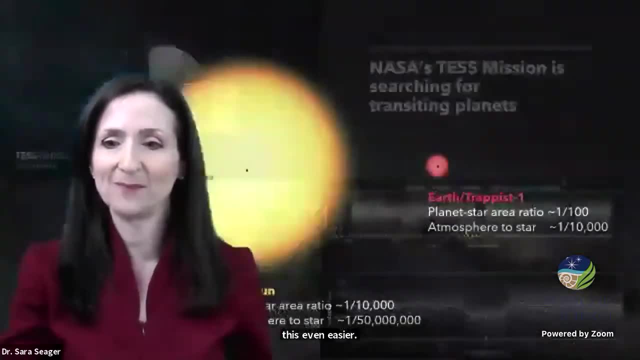 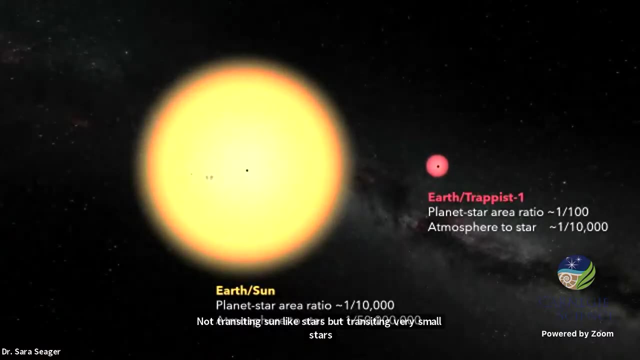 this even easier, And that is by looking at planets not transiting sun-like stars, but transiting very small stars. Here you can see, I'm showing you a real image of our sun And hopefully you can see this little dot here, this fake planet. 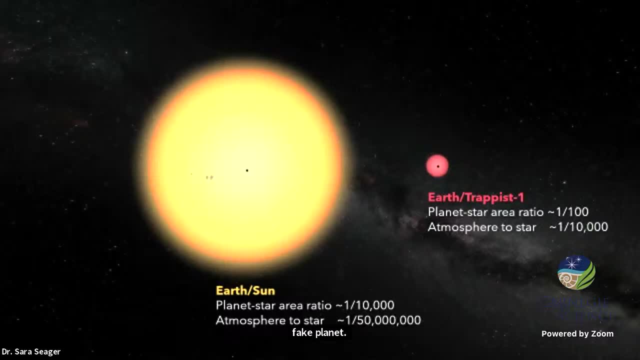 Just put my cursor on it And that's our sun and the planet to star area ratio which creates the drop in brightness. for an earth sun is one part in 10,000.. I said our earth is a hundred times smaller, but remember, pi r squared, we have to square that the radius. 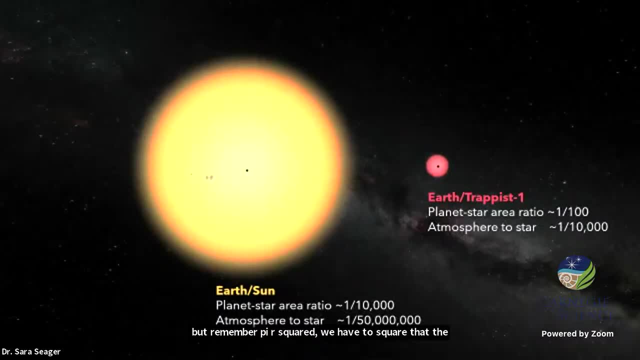 ratio. So it's actually the drop in brightness is one part in 10,000.. Well, we have very small red dwarf stars out there are incredibly common, And here's a fake image of a very small red dwarf star. it's only one 10th the size of our sun And in this case I put the same fake planet on it And 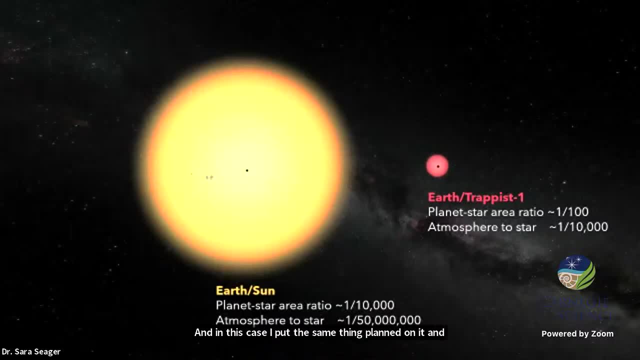 you can see right by eye that the planet is taking out much more area of the small star than of the big star, And so that drop in brightness is only one part in a hundred. as compared to our sun, it's would be one part in 10,000. So it's much, much easier to find small planets transiting. 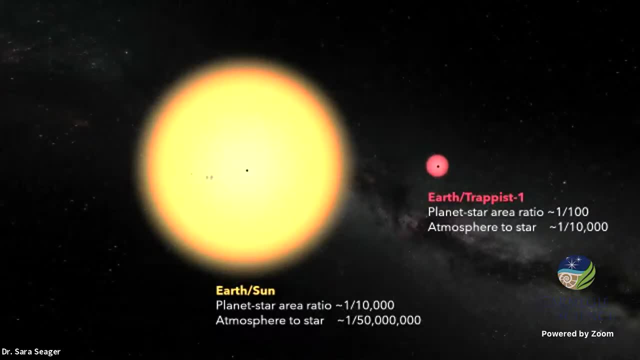 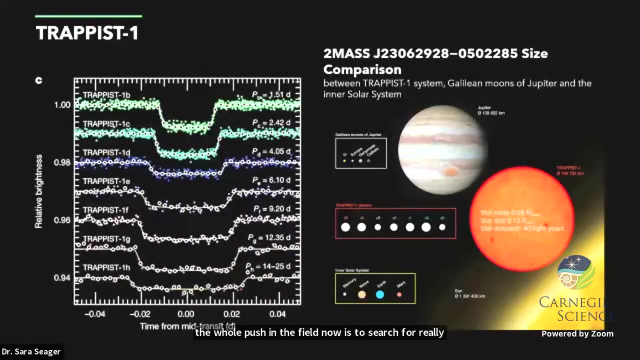 small stars than it is finding small planets transiting sun-like stars. So the whole push in the field now is to search for really small planets transiting small stars. By the way, there's a favorite small red dwarf star out there. Some of you might've heard of this. 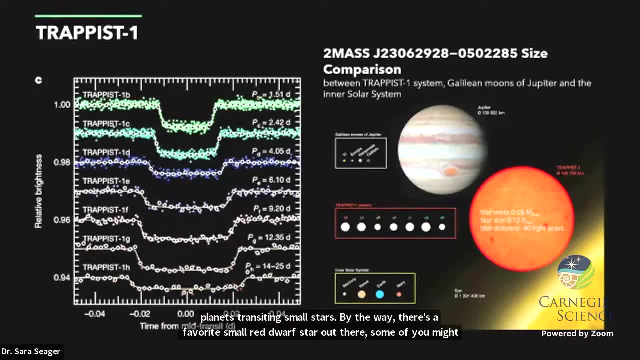 It's called Trappist-1.. And, by the way, some of these stars they just get named after their telescope survey because they don't have. they weren't stars that had previously been cataloged. And this star is amazing. On the right it's showing you the star, this orange blob. 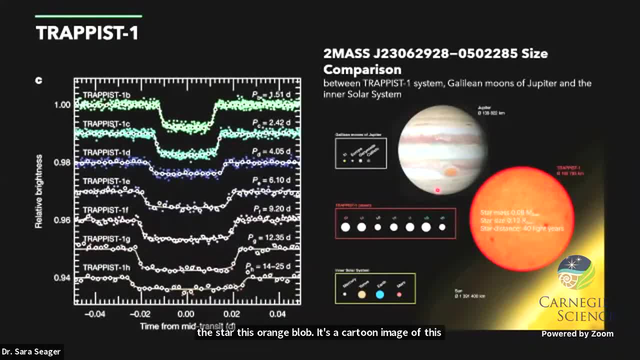 it's a cartoon image of the star compared to a real image of Jupiter. So the star is quite close in size to Jupiter, In fact any smaller and colder, and this object would not be able to have fusion on the inside. By very definition it wouldn't be generating energy. 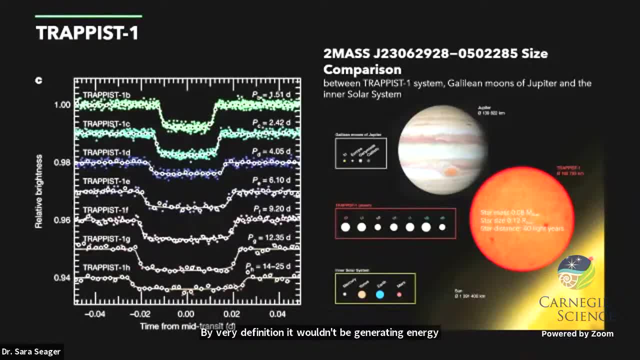 it wouldn't be a star. And on the bottom right you can see a little slice of our sun, just for comparison for how small the star is On the left. it's just some real data showing you seven, seven transiting planets transiting Trappist-1.. And some of these planets actually 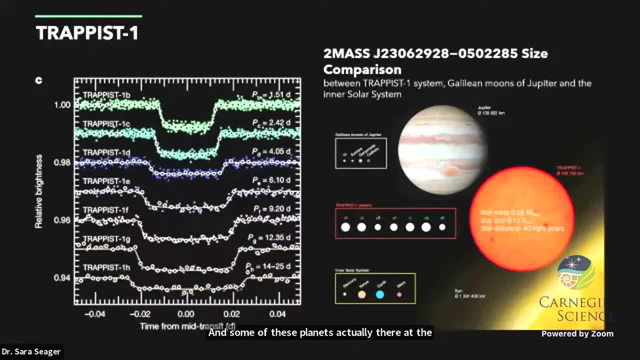 they're at the right distance from the star, So they're as heated by the star. They're not too hot, not too cold, but just right for life. So to explain these planets transiting small red dwarf stars a little better, let me take you on a very short but very virtual trip. 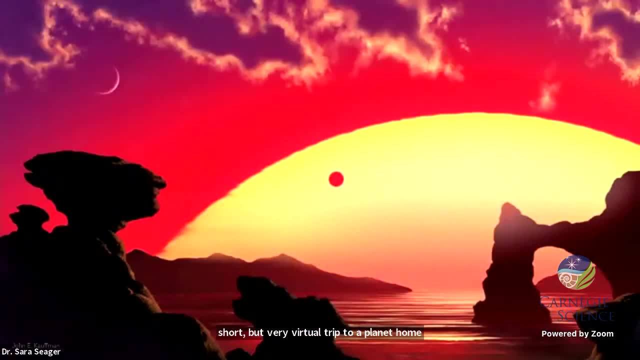 to a planet transiting a small red dwarf star. First of all, this is an artist's conception and it might be, depending on the star and the planet orbit, that the star might be very, very big in the sky, And this is because the red dwarf stars give off very little energy. 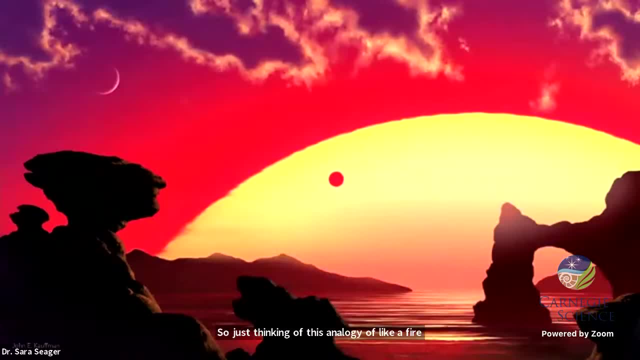 So just thinking of this analogy of, like a fire, an outdoor fire, if this fire is very small, you have to stand quite close to the fire to get warm. So the planets will be relatively close to the star actually, and the star might be big in the sky. 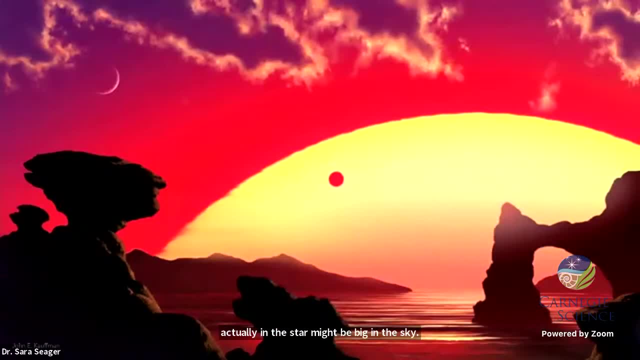 Here, the artist took an artist's license to make the sky red and the clouds purple, and they're showing you a couple of other planets in the same system. But these planets that are so close to the star tidal interactions over even just millions of years. 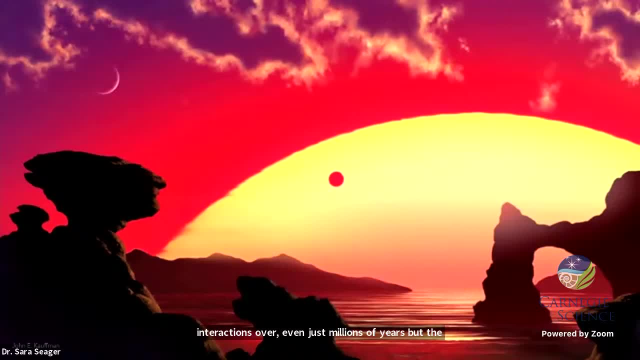 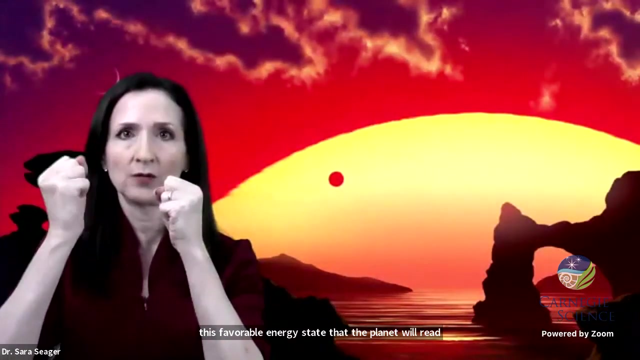 but the systems will be billions of years old. tidal interactions have made the planet have a special type of rotation and orbit, And we actually call it tidally locked Over time. it's this favorable energy state that the planet will rotate one time for every time it orbits. 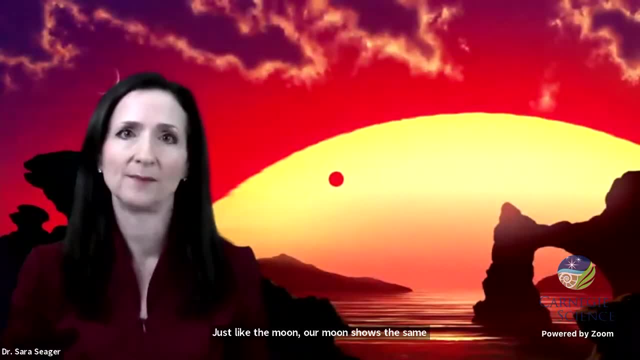 Just like the moon, our moon shows the same phase to Earth at all times. this planet will show the same face to the star at all times. and what this means for us, if we could visit this planet. it means that the one side, it means that we could that once, well one. side of the planet is always in daylight and one side is always in darkness. so imagine going to this planet and you could choose where to go. would you choose to go where it's always day, or would you choose? if you're an astronomer, surely you choose to go where it's always night? or i would really love to go where the sun is always setting. imagine having a nearly permanent sunset and we could look for there's this amazing phenomena: when the sun sets, if it's a clear horizon and like a large distance, you can see a green flash. so actually it would be amazing to go. 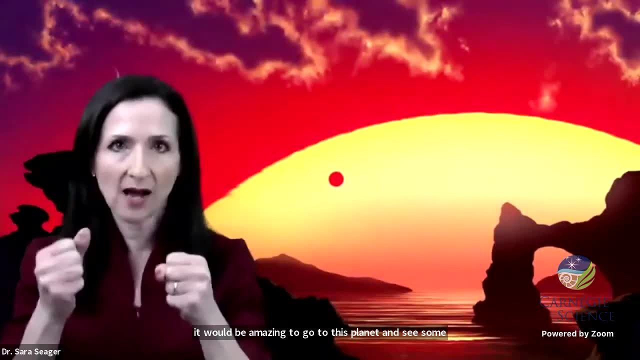 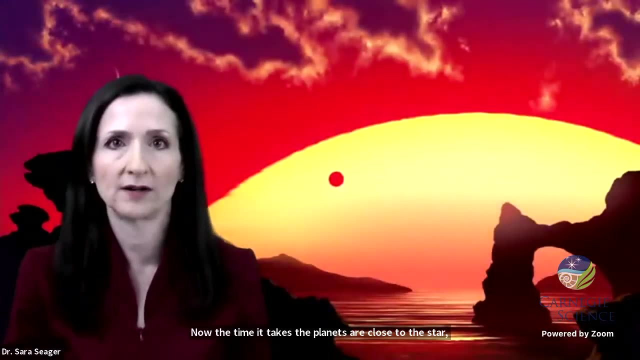 to this planet and see some really really cool phenomena. now the time it takes, the planets are close to the star, so by kepler's third law, the planet's year is really relatively short. you can see that the sun is always setting and the planets are close to the star. 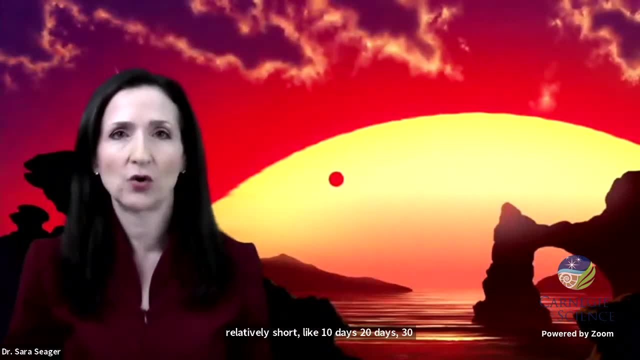 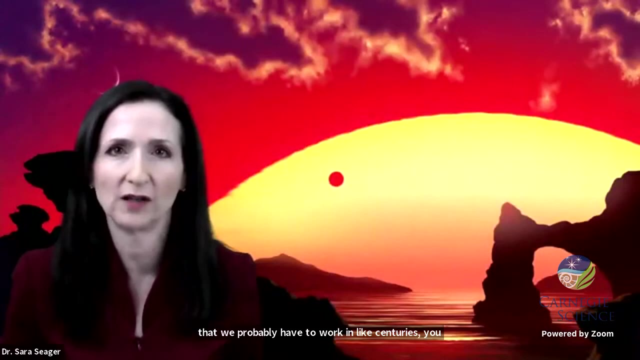 like 10 days, 20 days, 30 days, and so a year on this planet would only be that long, like 10 or 20 days. so that would be pretty tricky for accounting and all that we'd probably have to work in like centuries, you know, or every decade or every century, because 10 days isn't really long. 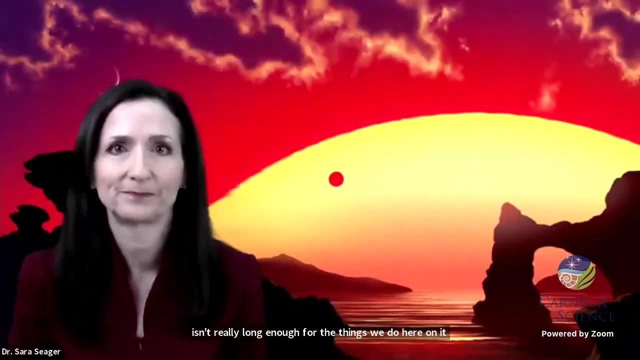 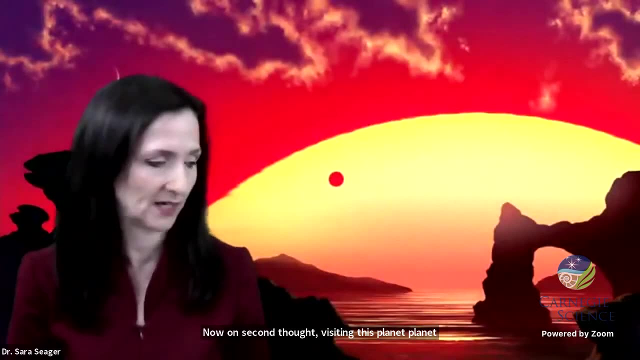 enough for the things we do here on an annual basis. now, on second thought, visiting this planet, a planet orbiting a red dwarf star, might actually be a terrible idea. we wouldn't be able to flip out and be glued. flip out and be glued to our phones. 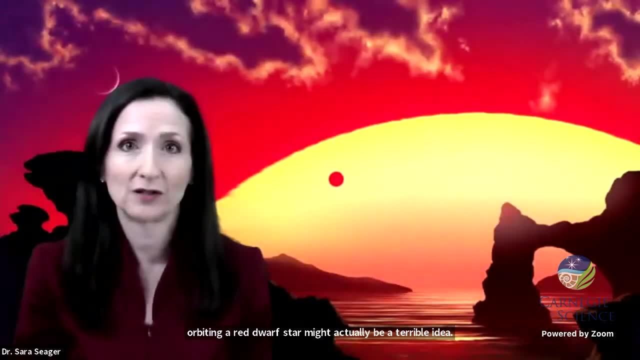 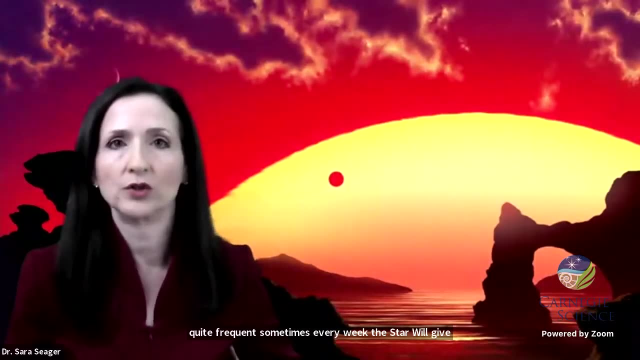 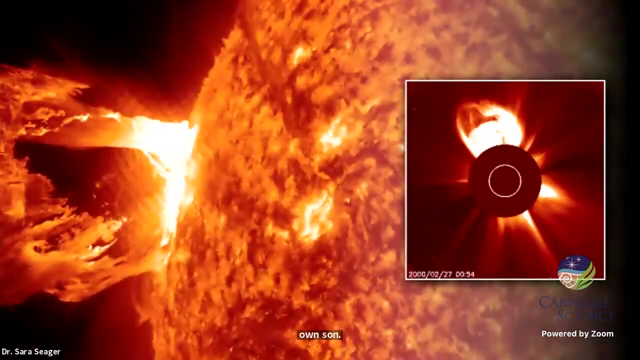 because these stars have high energy flares, sometimes quite frequent, sometimes every week. the star will give off a high energy flare where these particles would destroy electronics in the phone. it's like, um, what kind of sunscreen would you bring? it's really really rough actually, and we know that our our own sun um had a very crazy flare event uh, about 150 years ago this. 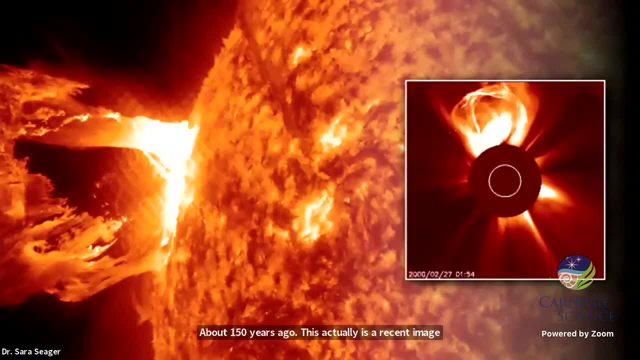 actually is a recent image from a satellite and it's showing you a very mild version of a flare, and this satellite image is taking out a very narrow wavelength. it's got a special filter that makes the sun look all modeled. this event was called the carrington event and our sun actually. 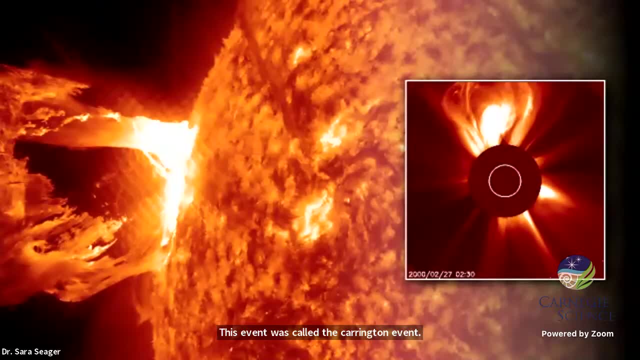 gave off a big flare and a part of our sun, called a coronal mass ejection, came hurtling towards earth and embedded in that part of the sun was a magnetic field which interacted with our magnetic field and induced a current, and it's one of my favorite images of the sun. 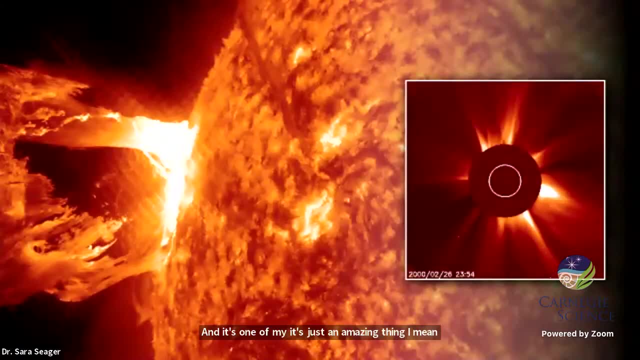 it's just an amazing thing. i mean, i'm not going to say wish we were there, but our earth became electrified and people could see northern and southern lights, almost down to the equator, if you're, you know, in the northeast, you know. here, apparently, we could have stepped outside. 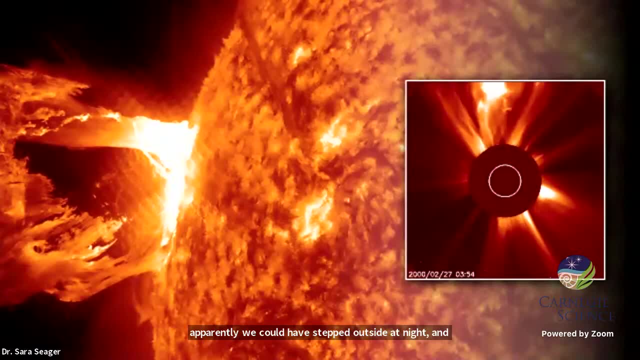 at night and it was so bright from the northern lights we could read a book by it. and the telegraph operators, their telegraph lines, caught fire and wow, it was just a crazy. no, no life got hurt, and i don't think this would preclude life or anything, but i was just trying to give 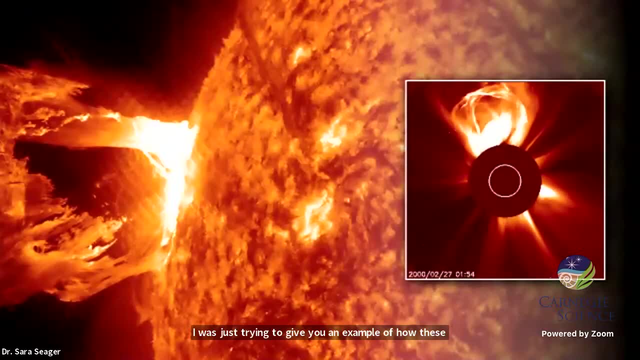 you an example of a fire. that was a big fire and i was just trying to give you an example of a fire, of how these planets orbiting red dwarf stars- they're not like Earth. actually We don't know what they're like. It's sort of one of the mysteries. 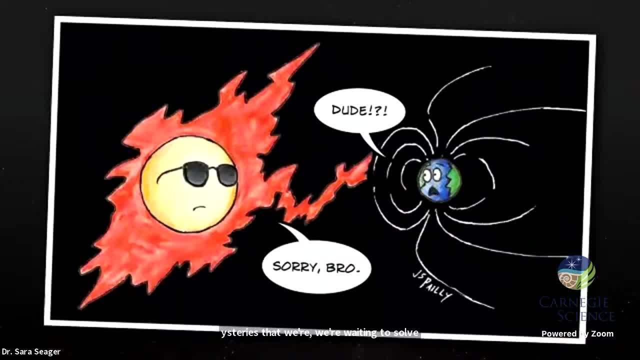 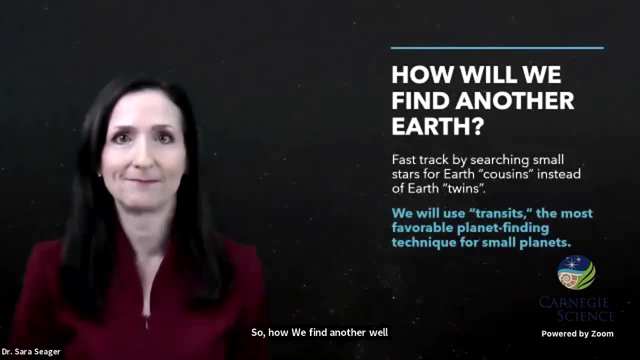 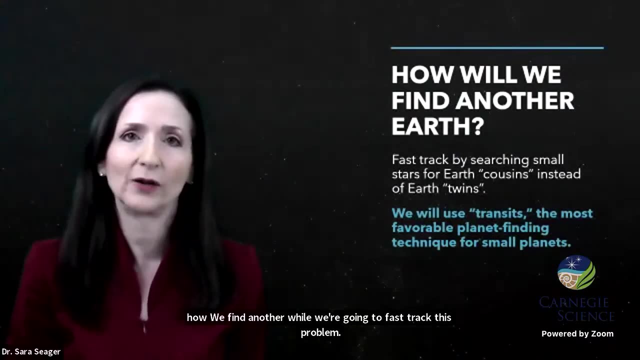 that we're waiting to solve with upcoming telescopes. So how will we find another Earth? Well, we're gonna fast track this problem, And a large part of the exoplanet community is behind searching small stars for what I like to call an Earth cousin. 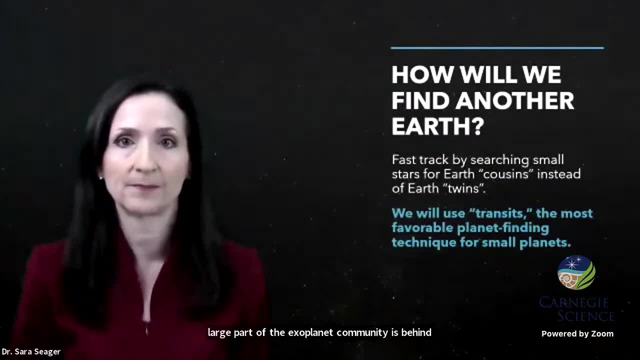 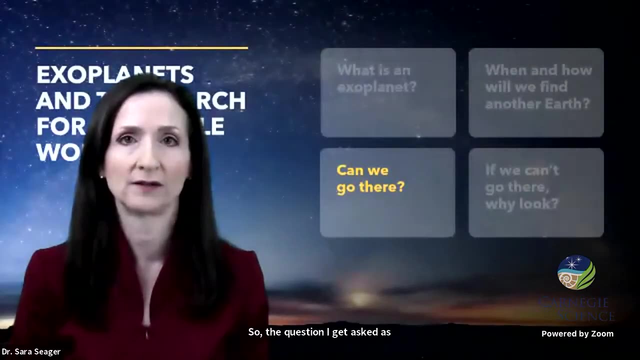 rather than an Earth twin. So we're going to use transits, the most favorable planet finding technique for small planets right now, And that's how we'll find our first other Earth. So the question I get asked- actually the one I get asked most often- 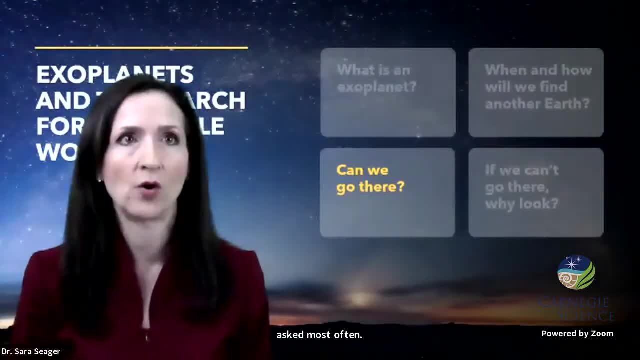 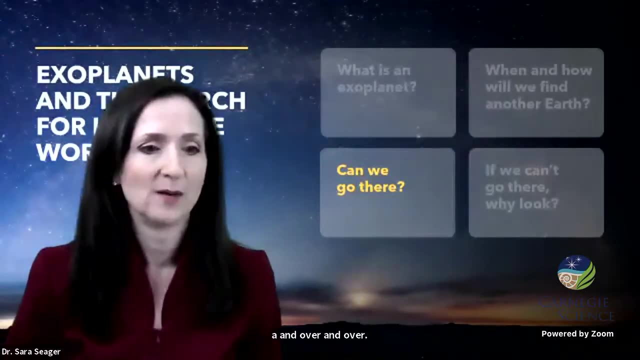 and I'll get asked this question and then explain it And then you know I'll get asked it again in the Q&A and over and over. And that question is: can we go there? Because people really love the idea of? 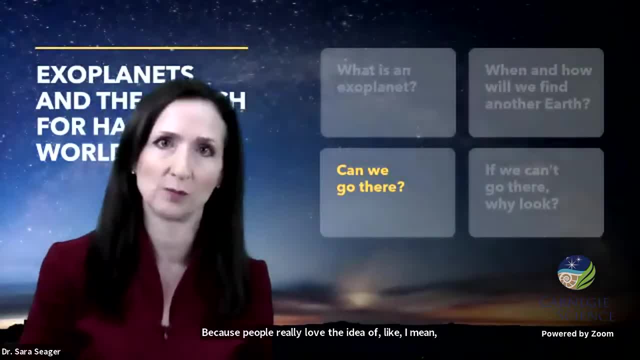 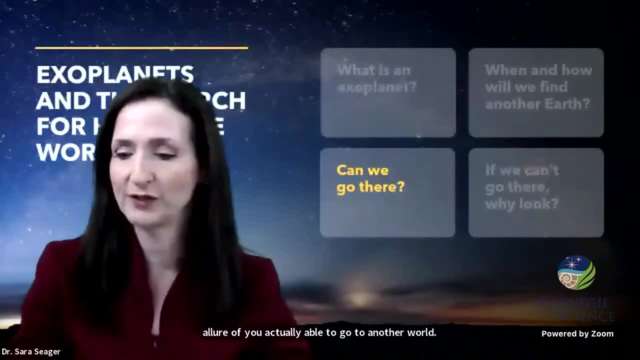 like. I mean, it's like the movies you know, science fiction, science fiction books, science fiction movies, the sort of allure of being actually able to go to another world. Well, this is really tough And I think a lot of you might already know the answer. 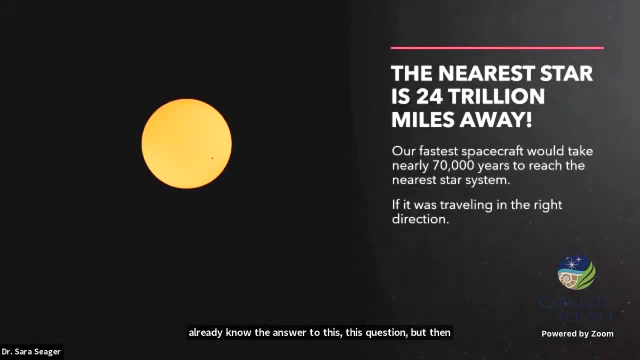 to this question. but the nearest star is so far away. It's four light years away, It's like trillions and trillions of miles away, And right now our fastest spacecraft would take nearly 70,000 years to reach the nearest star. 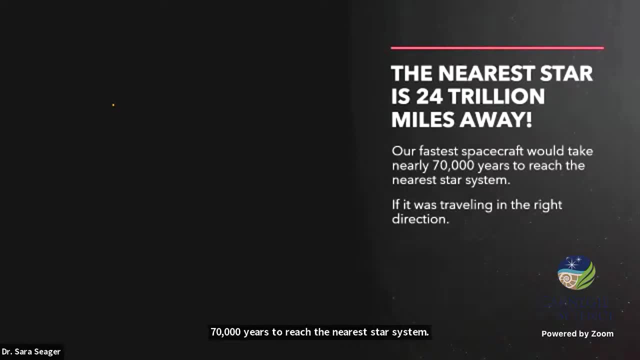 would take nearly 70,000 years to reach the nearest star. would take nearly 70,000 years to reach the nearest star. These are the Voyager spacecraft. by the way, They've already exited our own solar system And they're billions of. 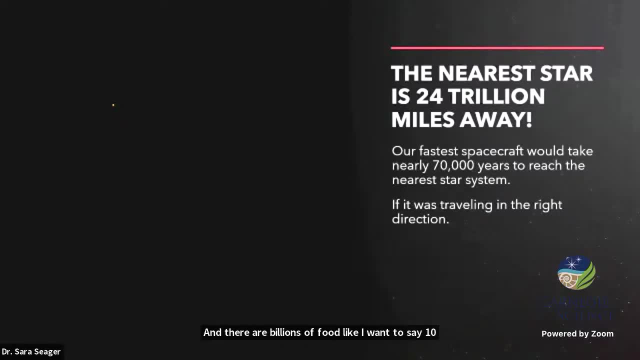 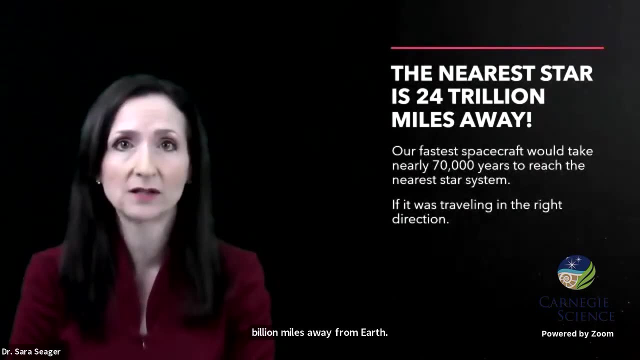 something like I want to say 10 billion miles away from Earth right now, But that's not, and it seems like a long time right. The Voyager spacecraft, launched in the late 1970s, left our solar system several billions of miles away. 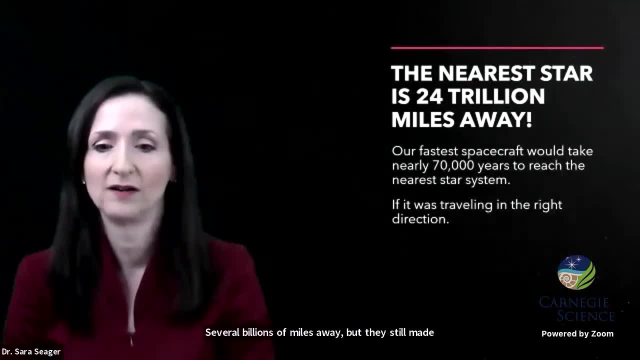 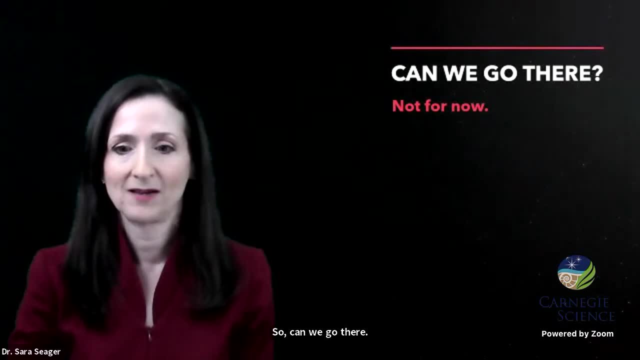 but they still made almost no progress towards the nearest star. So can we go there? The answer is not for now, And I think a lot of you knew that answer already. but the reason I'm telling you this is because in exoplanets, 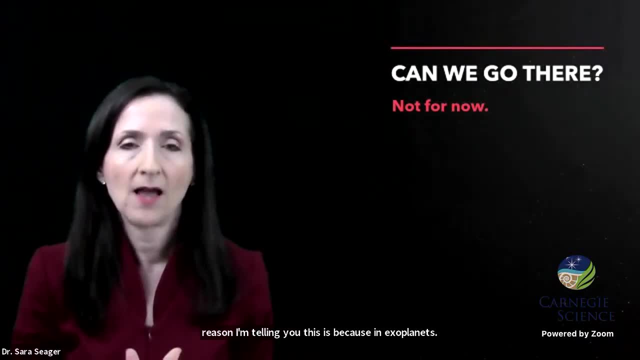 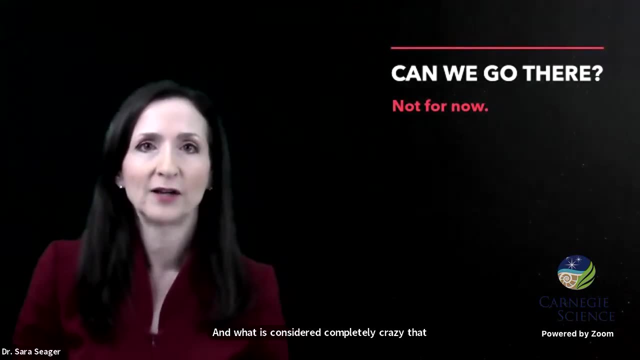 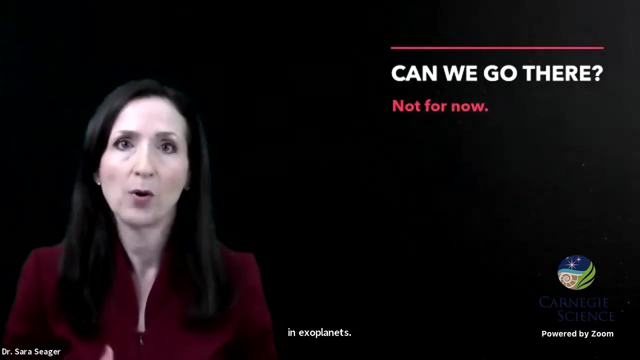 the line between what is considered mainstream and what is considered completely crazy. that line is constantly shifting And I'd like to just tell you about when I got my start in exoplanets: When I finished graduate school and I finished I was actually a postdoctoral fellow working. 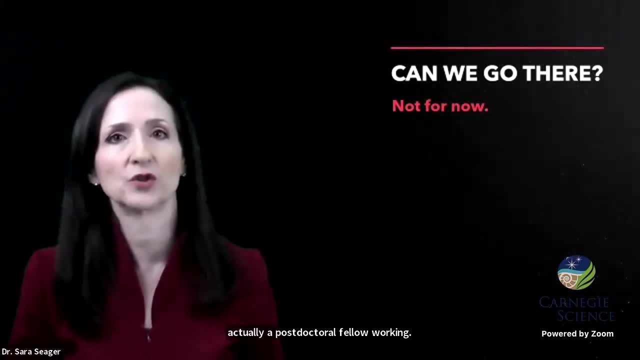 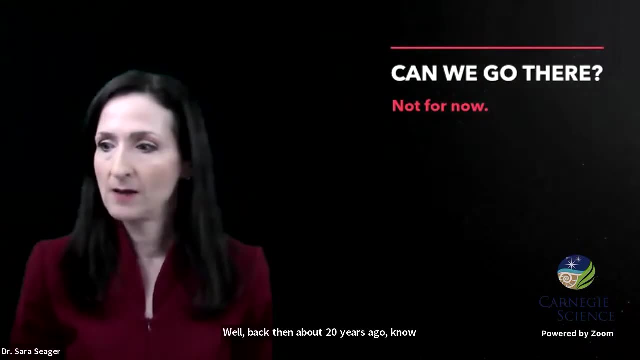 And I started to apply for faculty jobs where I would hope to continue research for the rest of my career. Well, back then, about 20 years ago, no one was hiring in exoplanets. People would get really nervous about it. I would give talks and go. 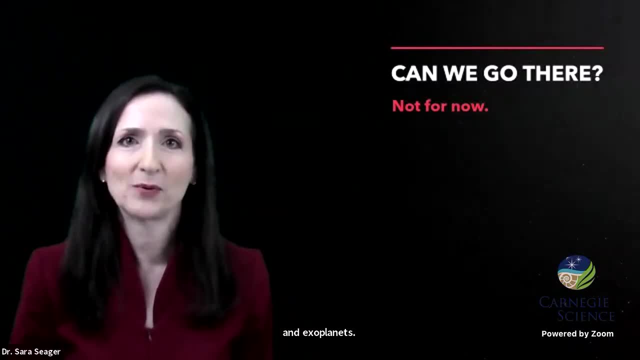 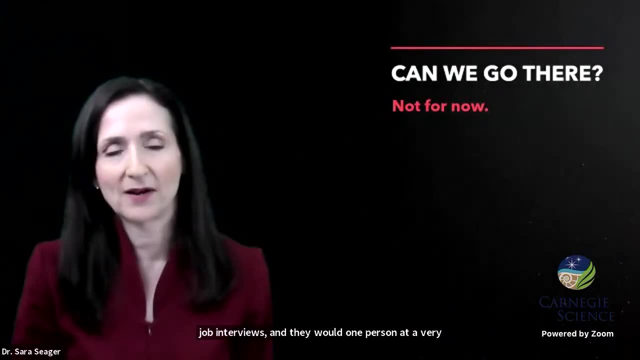 I would actually did get in job interviews and they would- one person at a very high ranking institution like- had the nerve to say: I don't think there's going to be very many transiting planets. At the time we had one transiting planet. 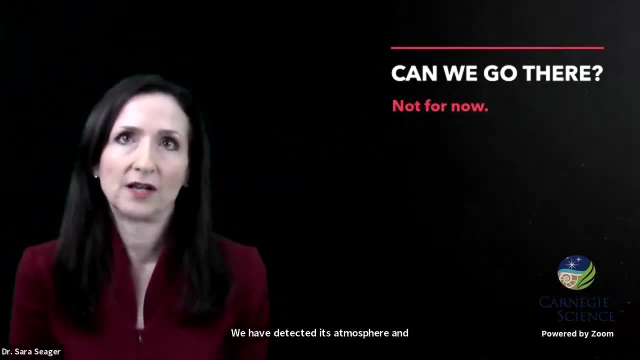 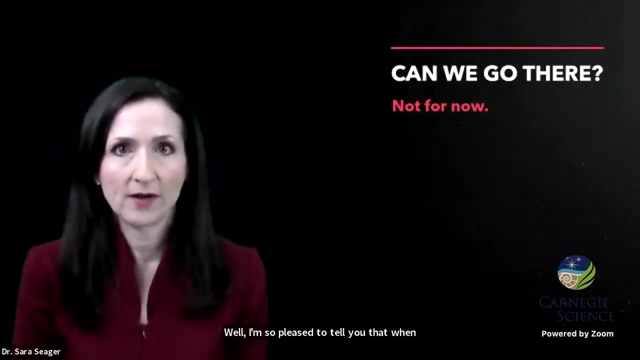 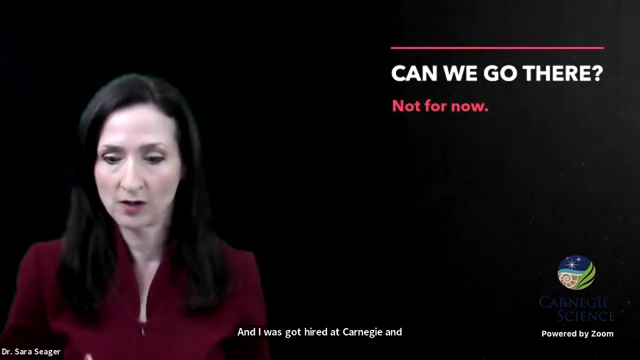 we had detected its atmosphere and people just were nervous. They just didn't think the field would go anywhere. Well, I'm so pleased to tell you that one major exception is and was Carnegie. And I was got hired at Carnegie and Carnegie the Department of Terrestrial Magnetism. 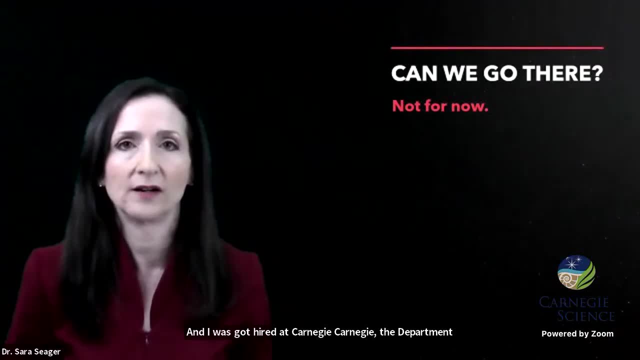 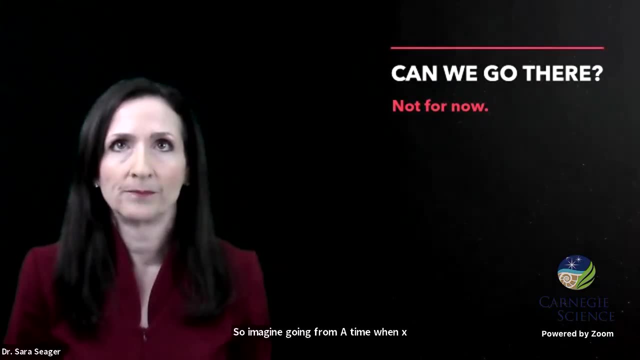 as it was called. we hired three people in this field and we had two already there, and we had a great group working in this. So imagine going from a time when exoplanets were. they were hardly any of them and people weren't sure if they were really planets. 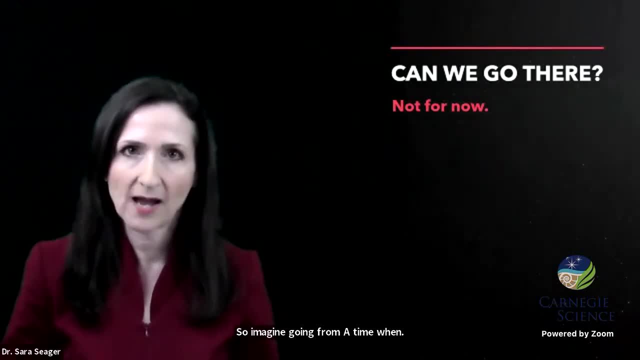 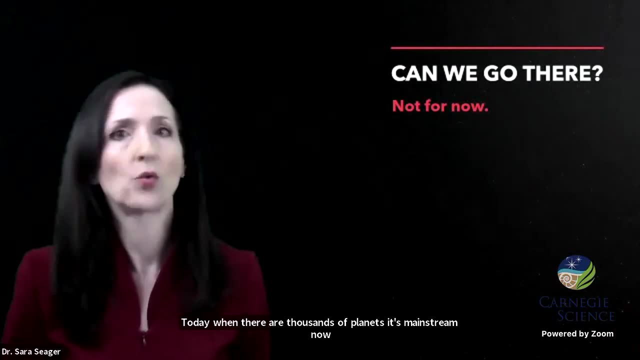 or perhaps they were false positives or events happening in the start itself to today, when there are thousands of planets. It's mainstream now to work on exoplanets. So I'm telling you all this as an answer to the question: can we go there? 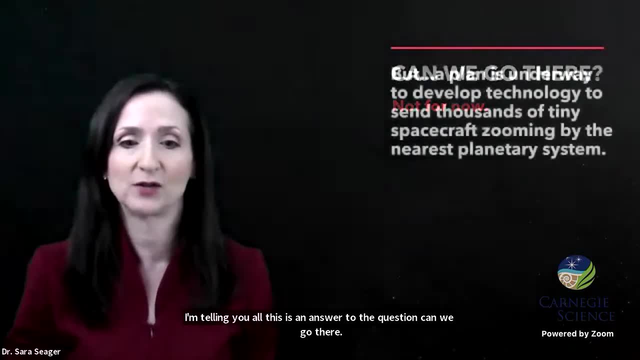 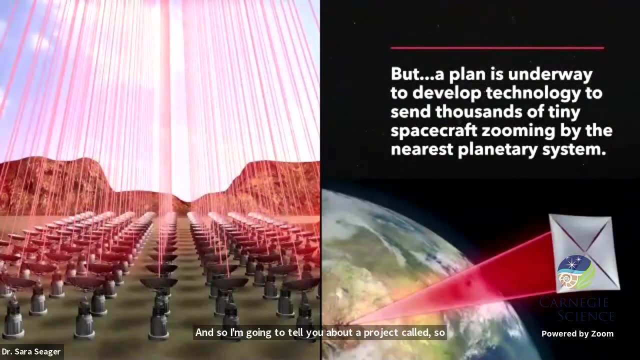 It sounds pretty crazy, but people are working on this and taking this question seriously, And so I'm going to tell you about a project called StarShot. I'm not personally involved this project, but I am a big fan of it, And Starshot is the idea that actually has it has. 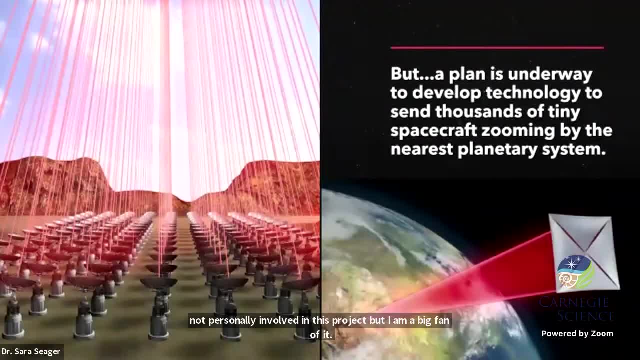 $100 million of private money to behind it. And that's actually- believe it or not- not enough to make it work, but it's enough to get it started. It's enough to shift that line between what is crazy and what might someday be mainstream. Now, this concept involves sending up thousands of 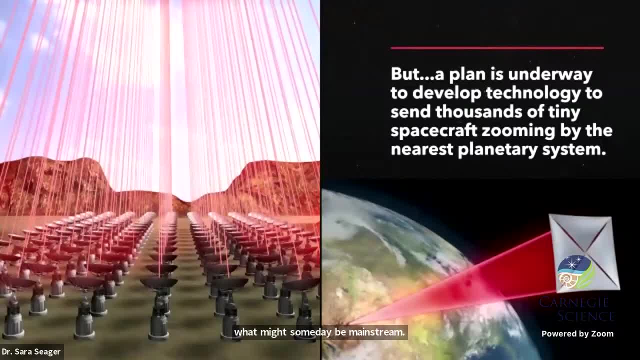 little tiny space chips- They call them space chips instead of spaceship- And each of these chips would deploy a sail of about one or two meters in diameter And just after they deployed a giant bank of lasers on earth, here on earth that would take like a hundred, like it would. 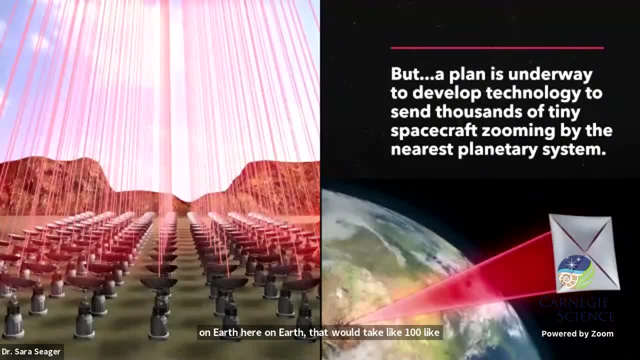 take about a square kilometer. It would have about a hundred gigawatts of power. That's like having a hundred watt light bulbs but a billion of them, And they would accelerate. they would light up these sails and by photon pressure they would actually accelerate the sails without. destroying them. And they would actually, they would actually, they would actually. they would accelerate the sails without destroying them. And out of these thousands of tiny spacecraft, we're not expecting all of them to make it, but they would get accelerated to about 20% the speed. 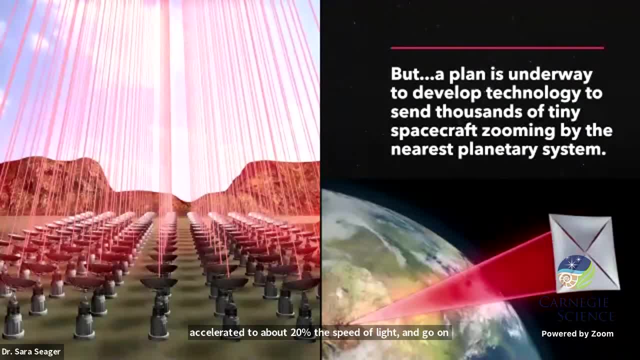 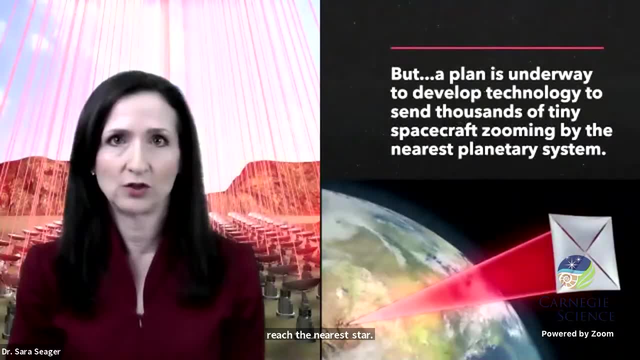 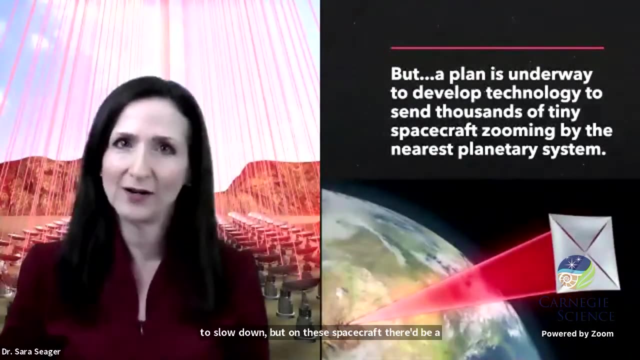 of light and go on a long journey that would take something like 20 years to reach the nearest star, actually the Alpha Centauri star system, And they would zoom by because they don't have any way to slow down. But on these spacecraft there'd be a camera and they'd be able to radio. 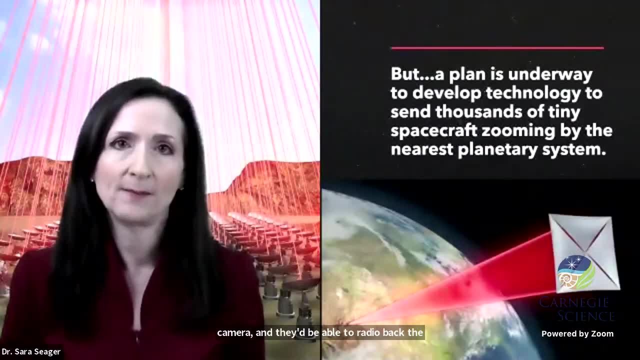 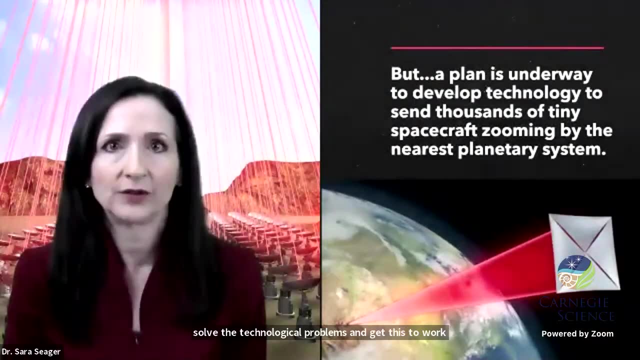 back the information, which would take a few years. So you know, we may be if this can work and if we can solve the technological problems and get this to work. you know it would take a while to get this to work. Maybe, I don't know, 20 years and then 20. 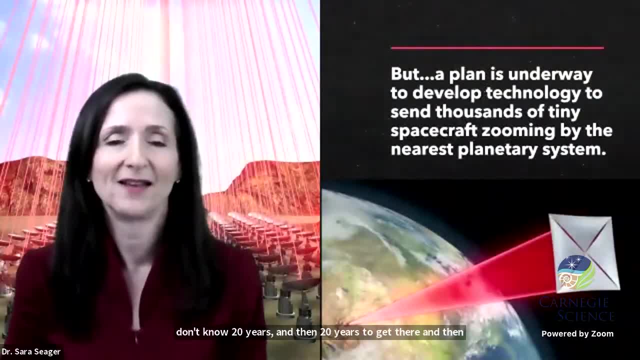 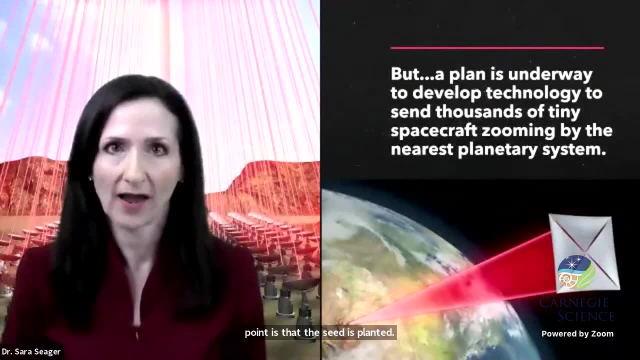 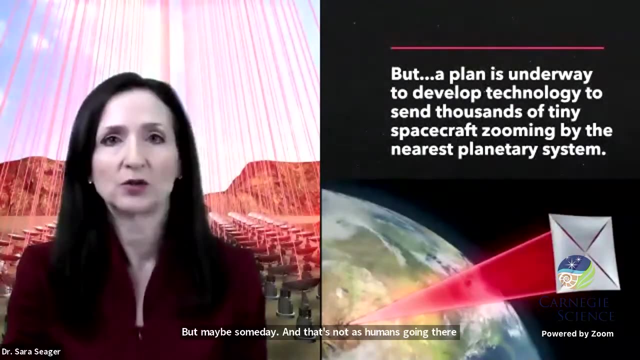 years to get there And then a few years to send the information back. So the point is that the seed is now planted And so, to answer this question, can we go there? Not for now, but maybe someday. And that's not us humans going there, but it is sending these spacecraft to send information. 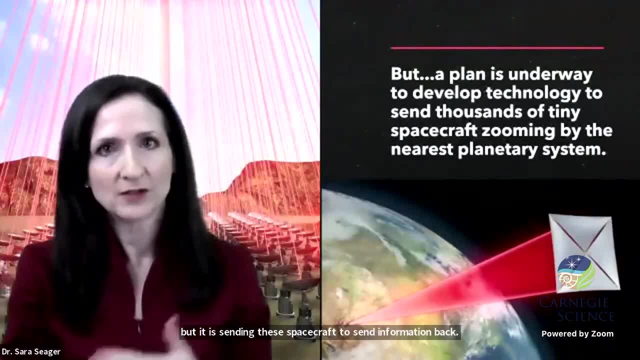 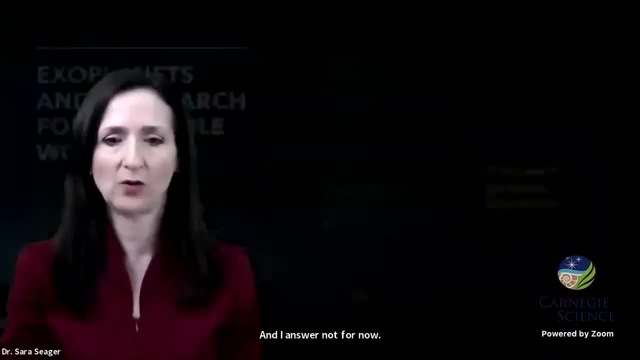 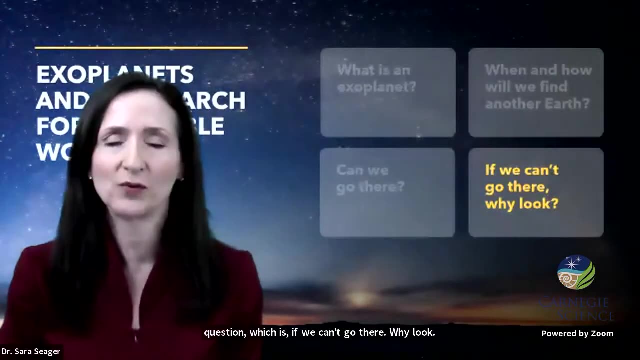 back. So in this series of questions, when people ask can we go there, And I answer not for now, There actually tends to be this immediate follow-up question which is: if we can't go there, why look? And the reason we're well, we, we, the reason we were looking, is because we can study. 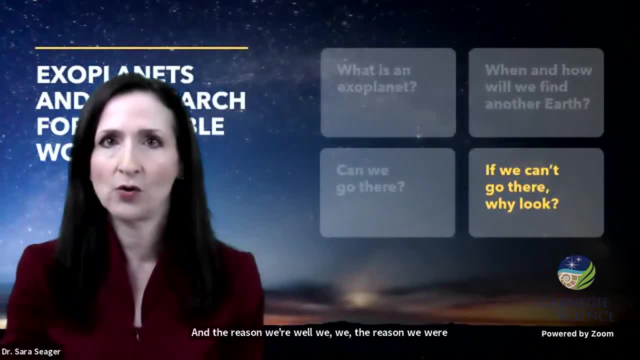 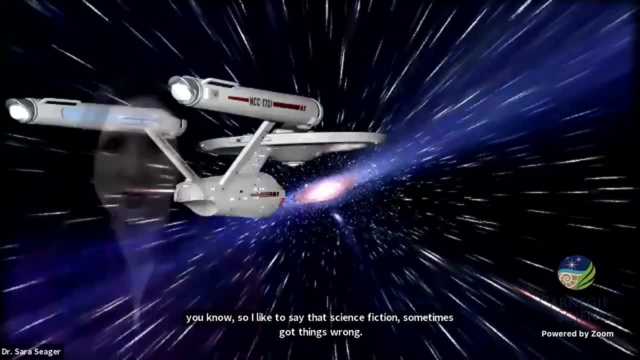 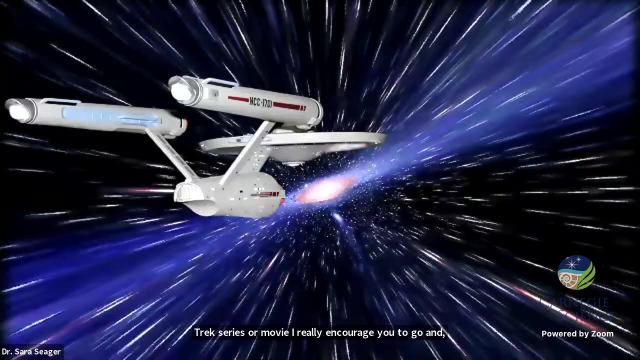 planets with the tools we have, And you know I like to say that science fiction sometimes got things wrong. So if you aren't a Star Trek fan or haven't seen a Star Trek series or movie, I really encourage you to go and and watch some of the shows. It's really 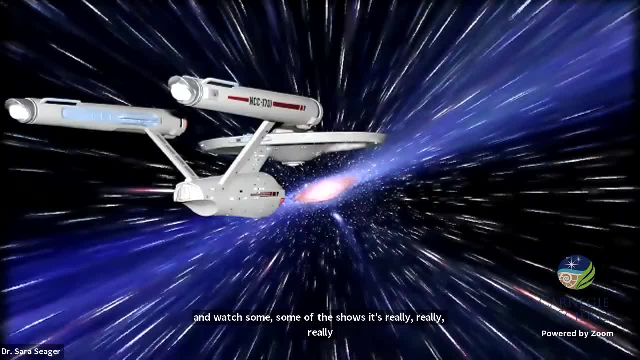 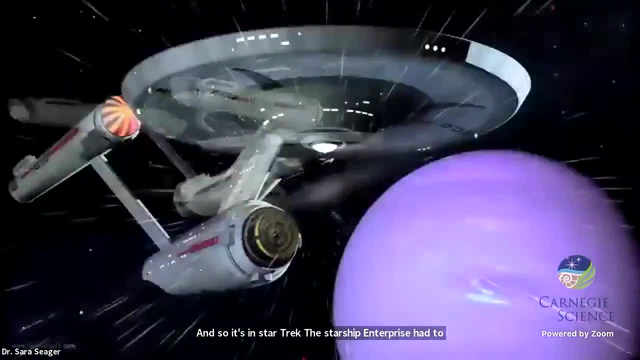 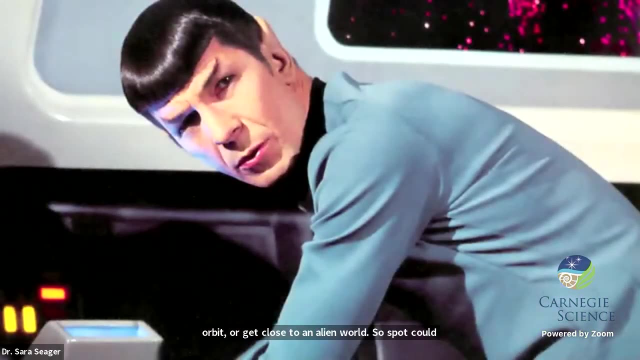 really, really fun. And so in in Star Trek, the Starship Enterprise had to travel incredible speeds, to travel vast distances, to orbit or get close to an alien world. So Spock could analyze if the atmosphere was habitable and if there were life forms on the. 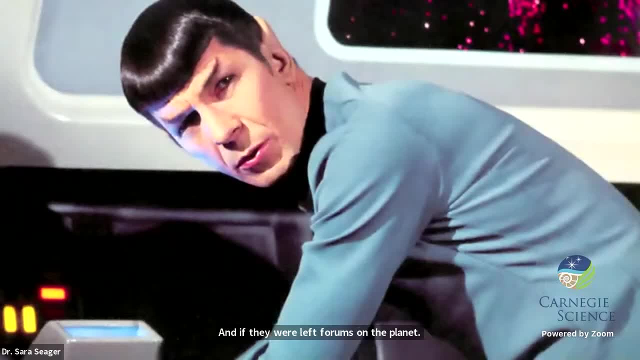 planet. So you know- I hate to disappoint some of you- We don't need warp speed to to study exoplanets And, in fact, if you wanted to make a TV series about astronomers searching for planets and studying their atmospheres, it would literally be incredibly. 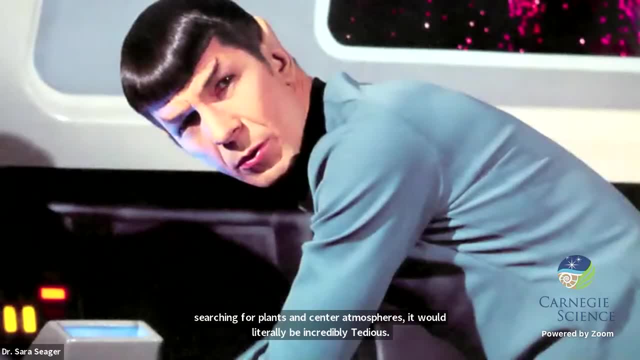 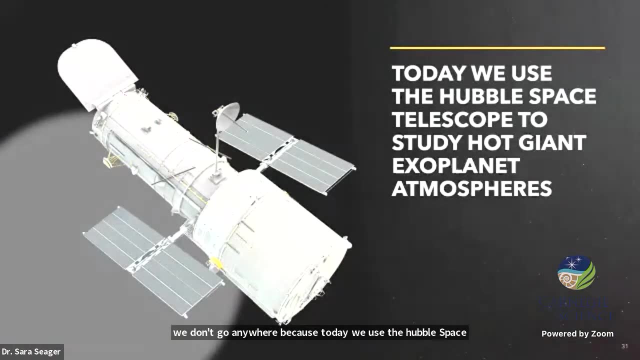 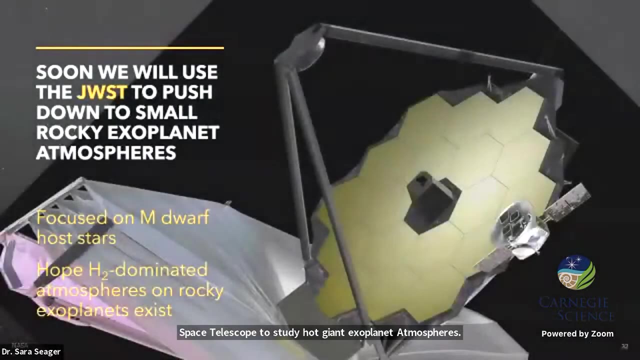 tedious because we we just work on our computers, just like a lot of you do. We analyze data, we crunch numbers, but here we don't go anywhere. because today we use the Hubble Space Telescope to study hot, giant exoplanet atmospheres And soon we will be using a new telescope. 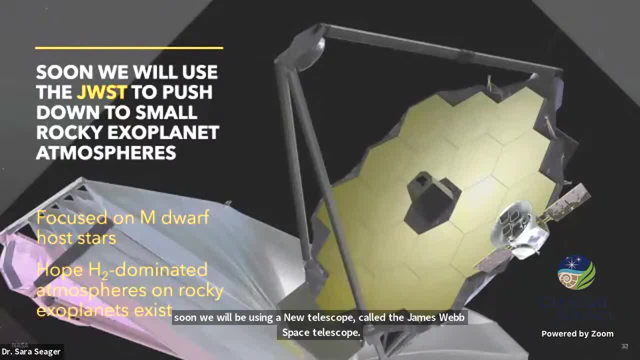 called the James Webb Space Telescope And it's going to be a really, really, really to push down to small rocky exoplanet atmospheres. This is an artist's conception of the James Webb Space Telescope, showing you this huge mirror. It's actually about six and a half meters in diameter. 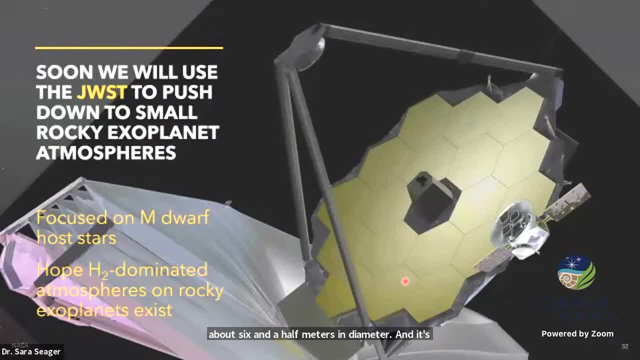 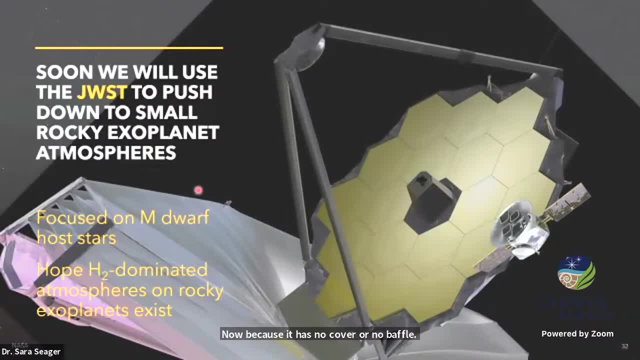 the James Webb Space Telescope has this giant tennis court sized sun shield which blocks light from the sun from entering the telescope and also blocks heat And actually there's five layers and they all have a different woven pattern, So it has one layer absorbs the radiation it gets sent out. 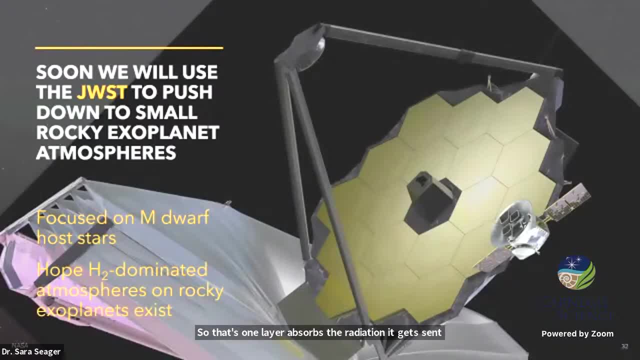 and absorbed by the next layer, but that it won't pass through layer. It's more likely to be sent off to the sides. Now, on this picture you can see TESS. TESS will not be flying together with the James Webb. It's here a bit of like a joke in that if you ever use a telescope- a somewhat big- 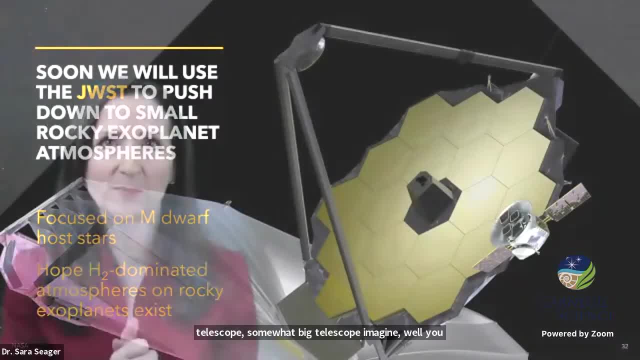 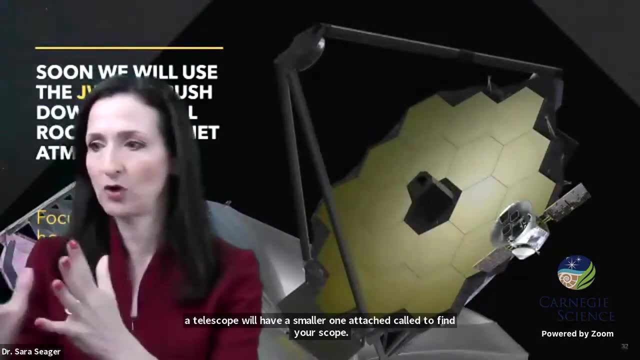 telescope imagine. well, you probably don't have one in your backyard, but typically a telescope will have a smaller one attached called a finder scope, And you use your finder scope to navigate and figure out where you want to point your telescope, And then the bigger telescope can. 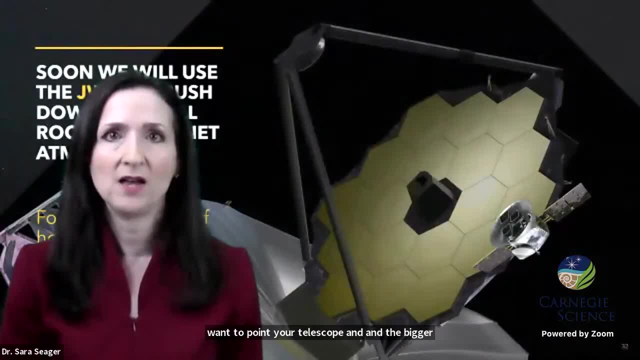 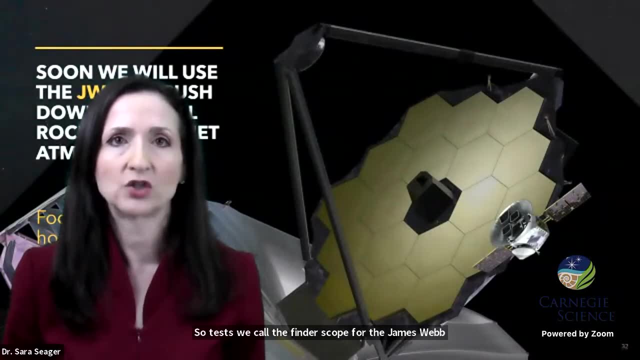 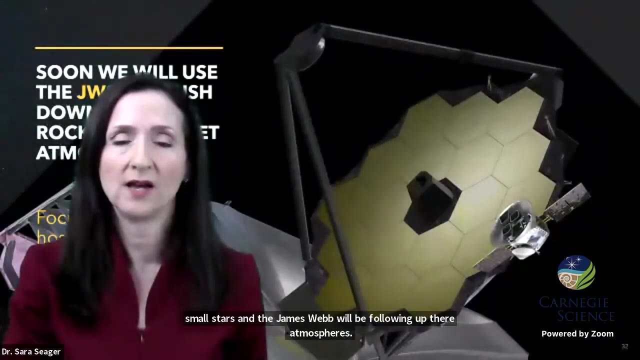 magnify or see objects more powerfully. So TESS we call the finder scope for the James Webb, because TESS is finding these sun shields, Small planets transiting small stars, and the James Webb will be following up their atmospheres And I wanted to explain to you how we, how we study planet atmospheres And this, this slide. 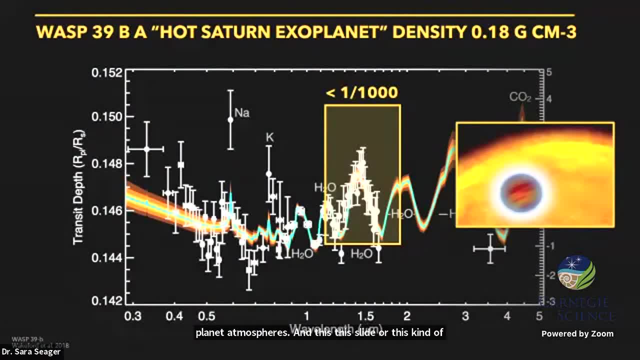 or this kind of moment is actually a little technical, So you don't have to understand this to understand the rest of the talk. but I wanted you to get a takeaway so that when you hear about, you may hear about in a few years, the first sign of life on an exoplanet and that you'll know. 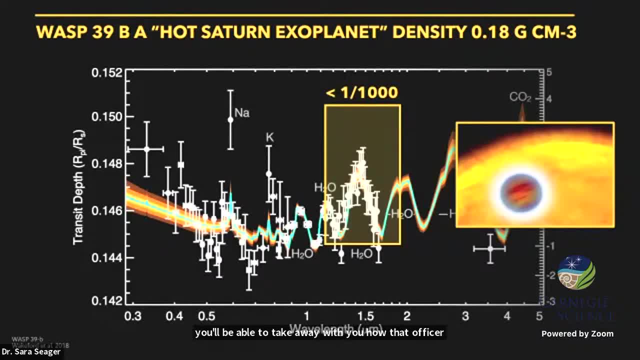 you'll be able to take away with you how that observation is made. What you're seeing in this, in this artist's conception of a planet in front of a star. on the right here for a transiting planet, you're seeing the atmosphere glowing as backlit by the star. 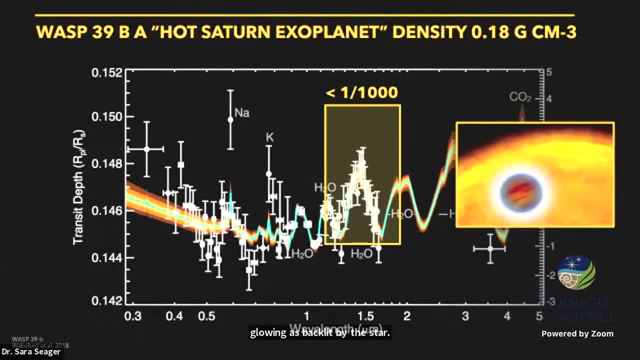 And here you're. what you're supposed to think about is when the planet goes in front of the star, some of the starlight shines through the atmosphere, And think about this like shining a flashlight through a fog. You know, some light makes it through, some doesn't. And here's the tricky part that I want you to try to get your head around. 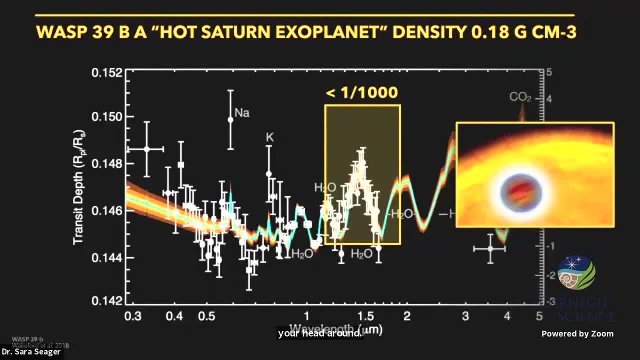 I want you to imagine observing the planet at a wavelength, at a like a color or wavelength, where the planet atmosphere is transparent, It is not absorbing, It doesn't have a gas that absorbs. at one specific wavelength, Then the planet size is the, the diameter of the planet or the area is. you know, it's this black, this dark brown planet that the artist has has colored it dark brown. 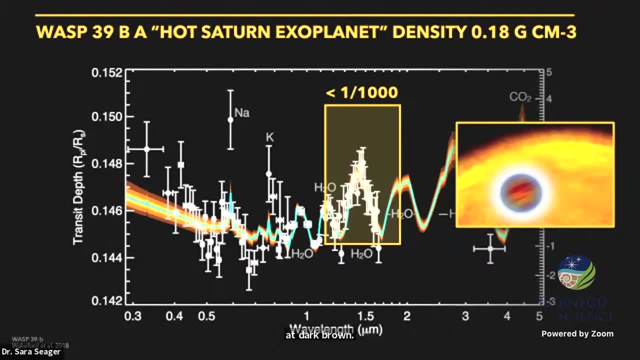 Now I want you to imagine observing the planet with a telescope at an adjacent wavelength, a wavelength where the atmosphere is transparent, The atmosphere is opaque, where it's highly absorbing. All of a sudden now the planet looks a little bigger, because now the diameter of the planet extends from the edge of this blue, glowing atmosphere to the other edge of it. 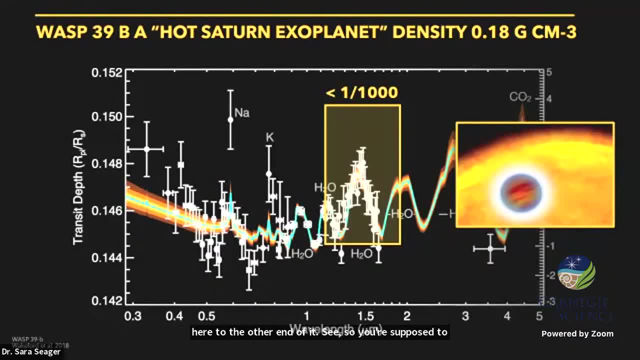 See. so you're supposed to see that the planet is bigger when the atmosphere comes into play and it's smaller when the atmosphere is not important. So, effectively, we're looking for a change in planet size as a function of wavelength, And that's how we study exoplanet atmospheres. 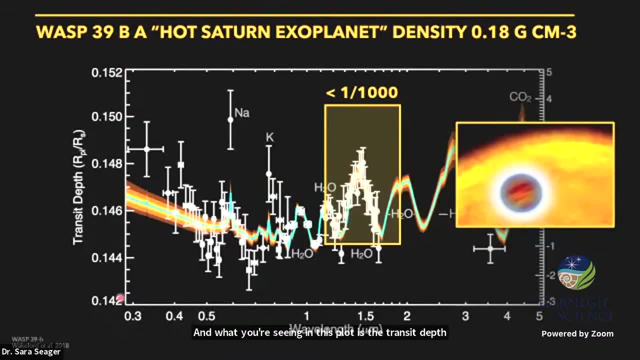 And what you're seeing in this plot is the transit depth. So this is the drop in brightness of a planet as a function of wavelength, where on the left side it's visible wavelengths And on the going past one micron it's infrared wavelengths. 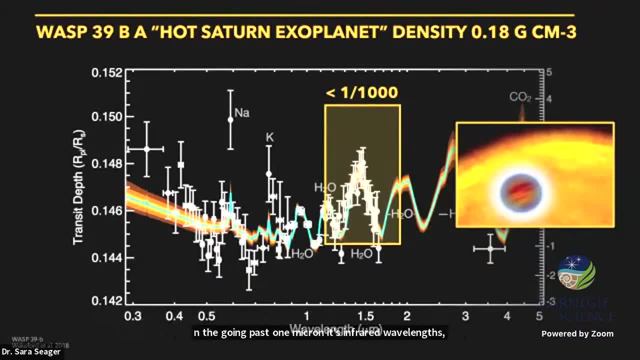 And the white points are data from the Hubble Space Telescope And the curves are models. They're models that model atmospheres, And what you're supposed to do is look at this plot and agree with it, And agree with me that the white points are different from a straight horizontal line. 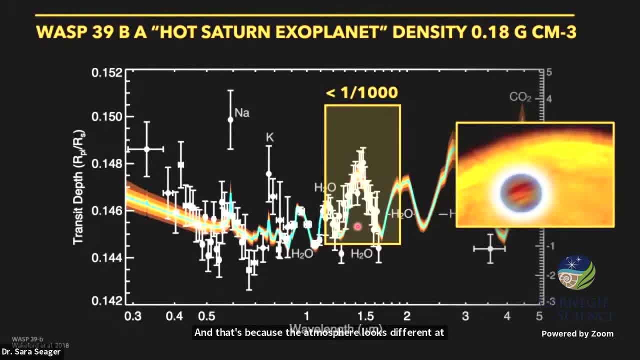 And that's because the atmosphere looks different at different wavelengths, looks a tiny bit bigger at wavelengths, actually looks one part in a thousand bigger at wavelengths where water vapor is known to be strongly absorbing. And so, if you agree with what I've said, this is different from a straight line and the model matches the data, at least here in this orange box. this is a discovery of water vapor on a hot, giant exoplanet. 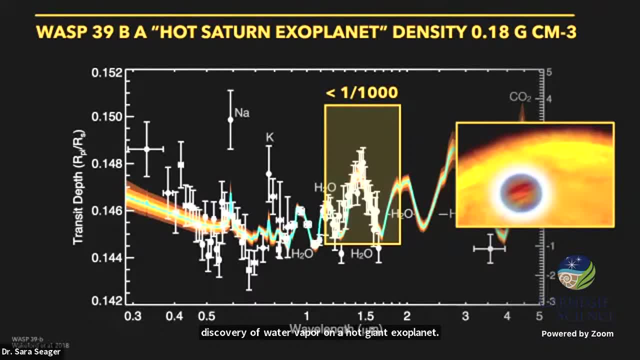 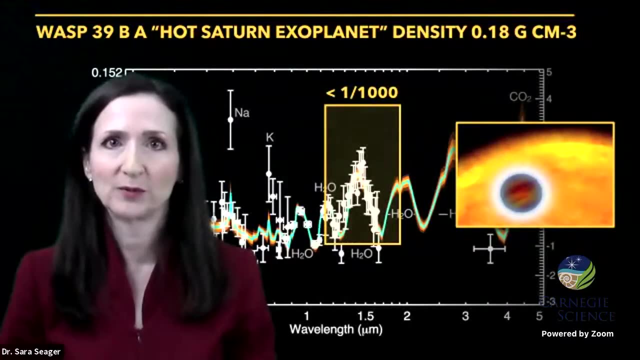 And this is data is taken with Hubble and that's we're all excited about the James Webb Space Telescope and and actually today the James Webb Science Office announced proposals, that competitive proposals, that that now we know which exoplanets are going to be observed. 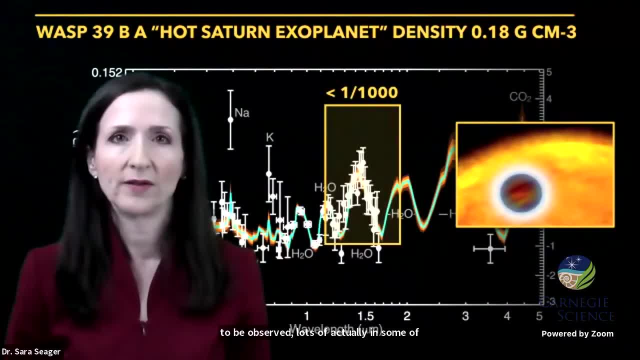 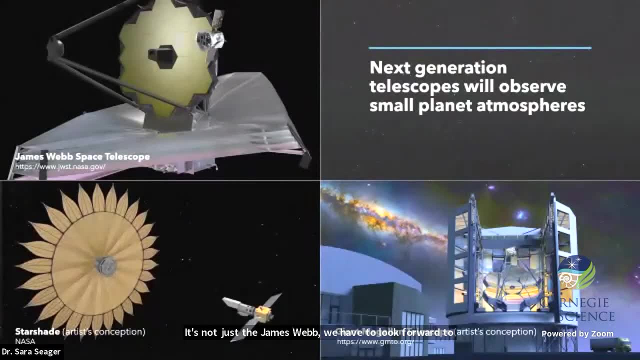 Lots of them actually, and some of them are small. What we think are small rocky worlds. It's not just the James Webb we have to look forward to. There's other telescopes I didn't have time to talk about, I was just 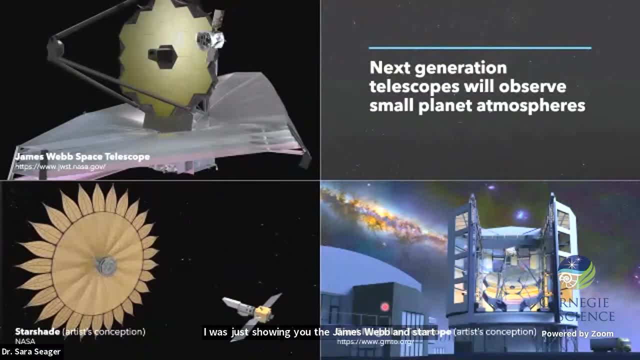 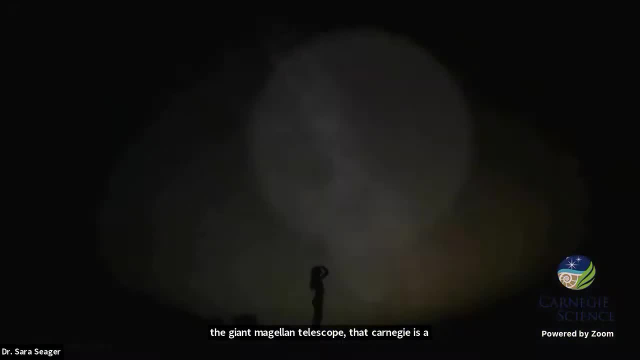 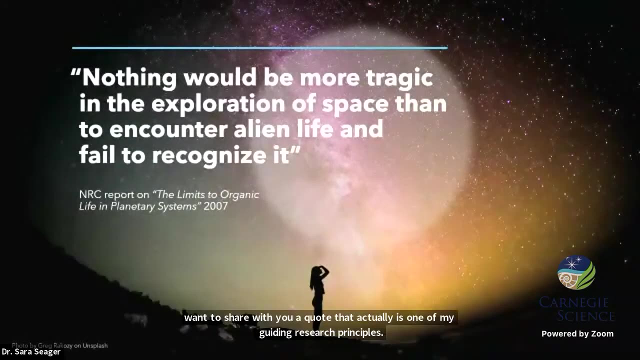 Showing you the James Webb and starshade and the giant Magellan telescope that Carnegie is a leading player in. So just in the last few minutes here, I want to share with you a quote that actually is one of my guiding research principles, And this quote came out of a National Academy of Sciences report. 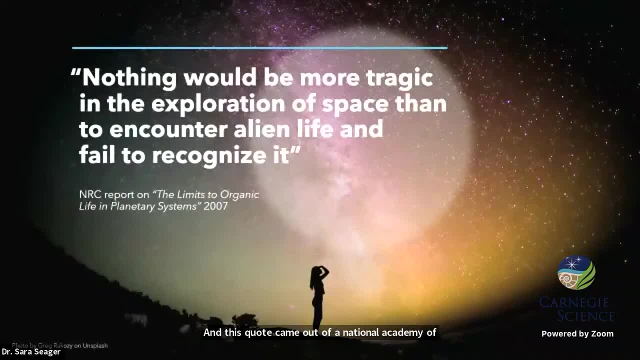 It was actually about our solar system. It was actually about finding life in our solar system, on planets and moons. here This quote says: nothing would be more tragic in the exploration of space Than to encounter alien life and fail to recognize it. So the reason why this stays with me is because our Earth only had significant atmospheric oxygen for the past billion years. 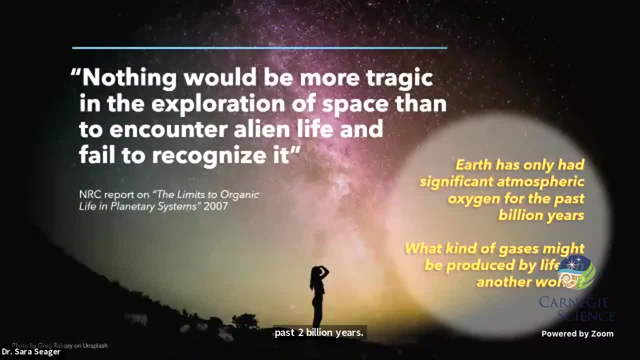 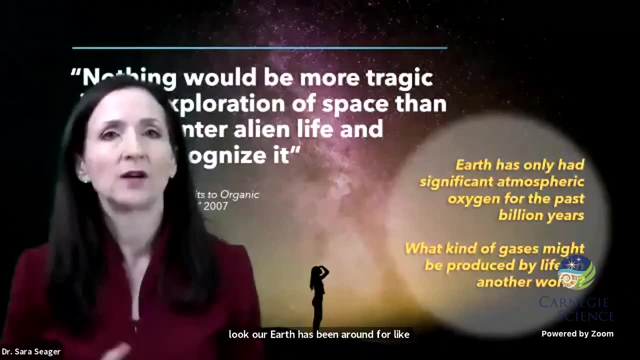 And you know, billion years seems like a long time, But look, our Earth has been around for Like over four and a half billion years. So we think of oxygen as a wonderful biosignature gas. where we define a biosignature gas, 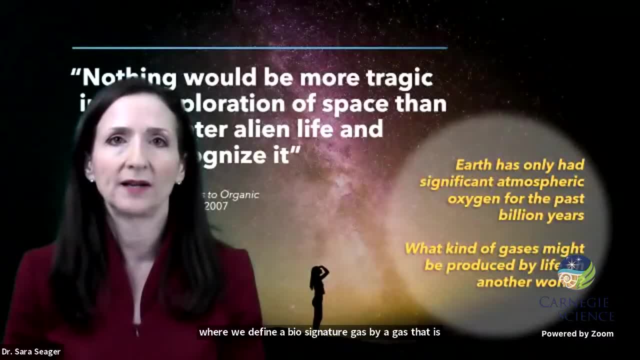 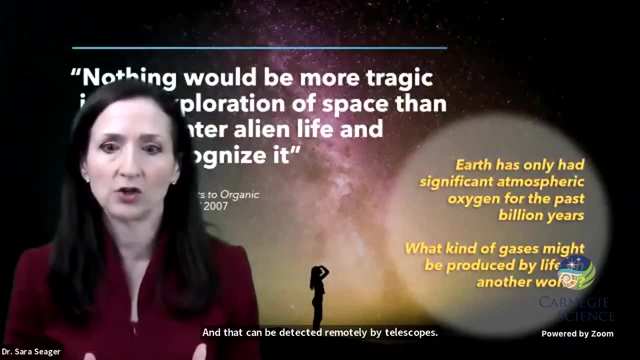 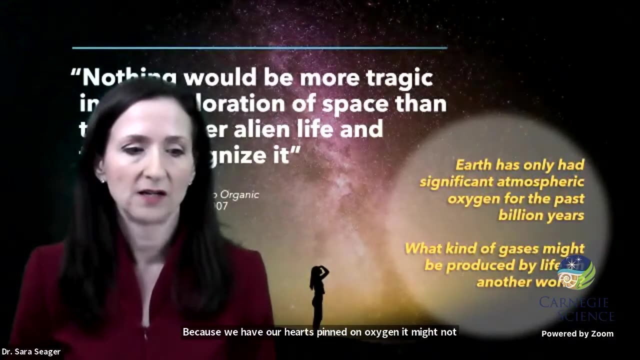 By a gas that is made by life, that can accumulate in the atmosphere and that can be detected remotely by telescopes. But oxygen is not the only one Right. And it shouldn't be, because if we have our hearts pinned on oxygen, it might not even be in another planet if the atmosphere hasn't yet saturated. 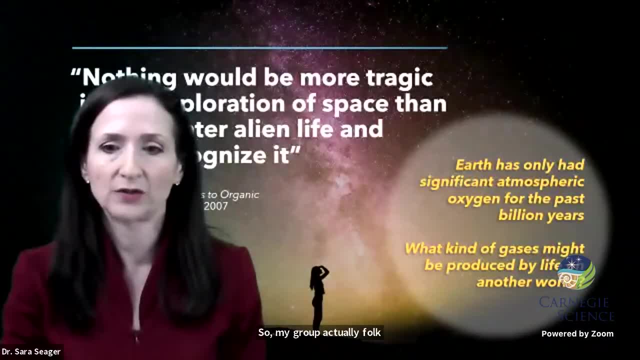 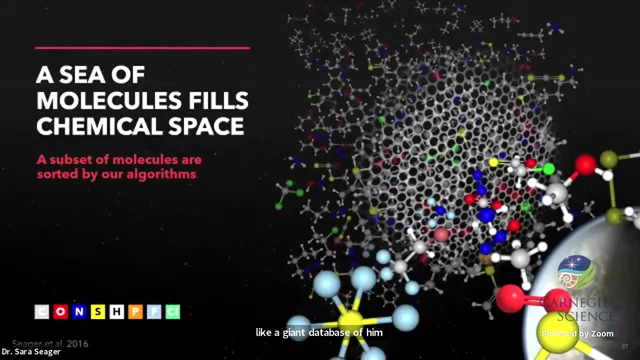 So my group actually focuses on the search for biosignature gases And, believe it or not, we constructed like a giant database of molecules. Of every molecule that could be in gas form, It could be a potential biosignature gas, And life on Earth in fact produces thousands of gases. 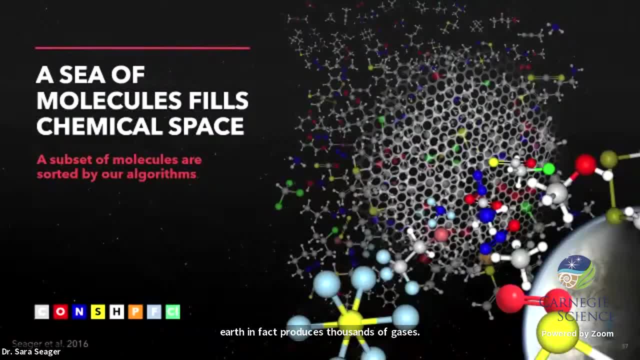 Thousands of gases, And it may be that each one of these- like it's not true that each one- could be a biosignature. Some of them are made in very, very small quantities, But I can address some of these in the Q&A if you have more questions. 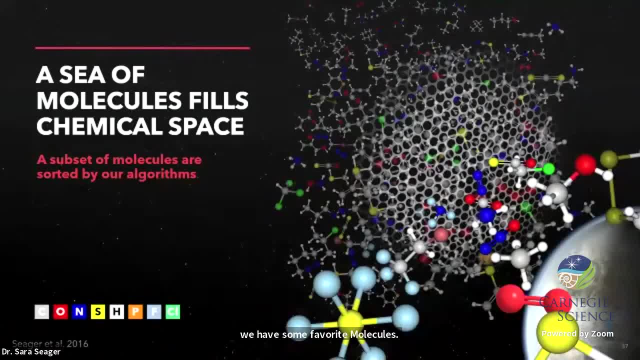 Let's just say we have some favorite molecules, Some of our molecules like methane or nitrous oxide Or hydrogen Or hydrogen sulfide- Those are tricky because they're also produced by mid-ocean ridges and volcanoes and other things- Photochemistry. 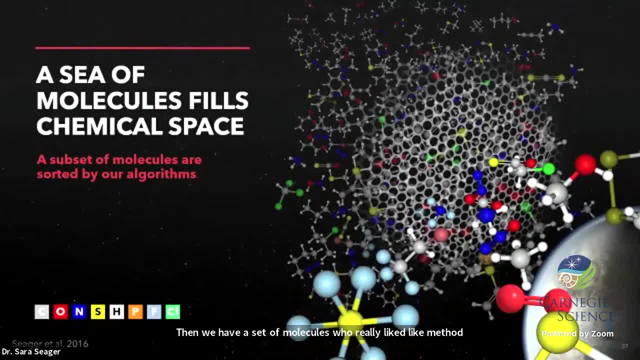 Then we have a set of molecules we really like, Like methyl chloride, Dimethyl sulfide, That are more complicated molecules, Less likely to be made by volcanoes, But they tend to exist in very small quantities. So we're still kind of working through this. 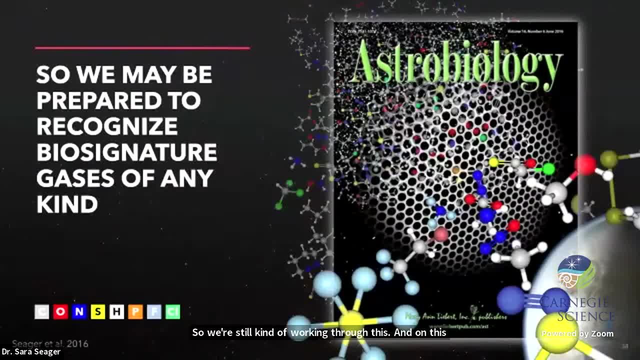 And on this chart you see a sea of molecules fills what we call chemical space in the background, And they're sorted by this shaker filter, Which represents my team's computer algorithms, And they're sorted into different streams, Some of which go by a planet. 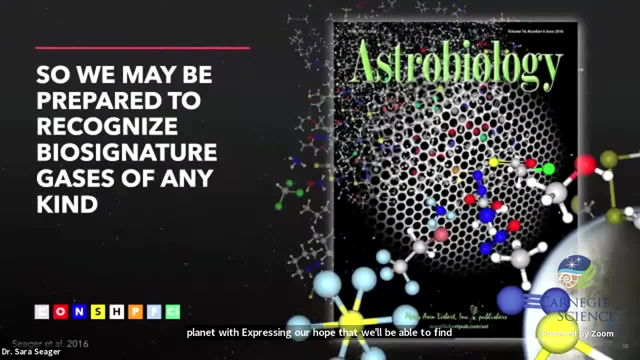 With expressing our hope that we'll be able to find and identify molecules that don't belong in context with the rest of the atmosphere And that can be attributed to life. So, to summarize this last question: If we can't go there, why look? 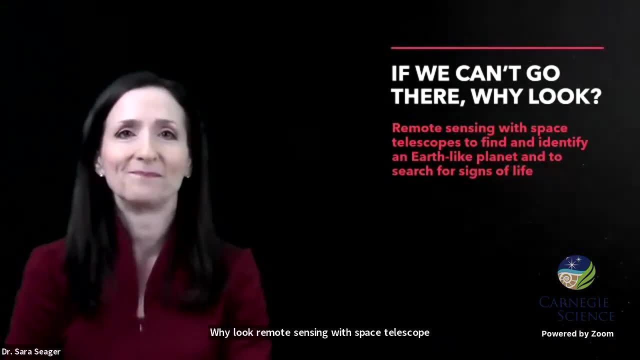 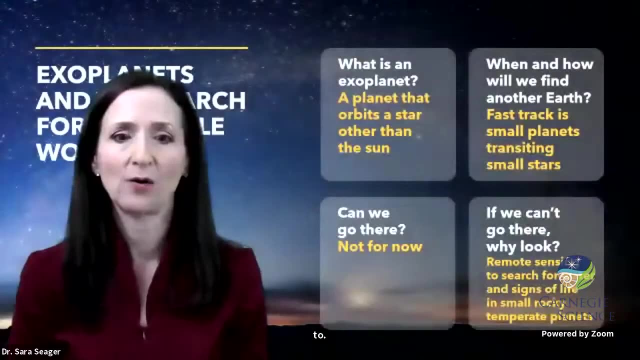 Remote sensing, with space telescopes to look at atmospheres And to understand them, And to search for signs of them, And to understand them, And to understand them. Now I'm going to summarize What is an exoplanet. It's a planet that orbits a star other than the sun. 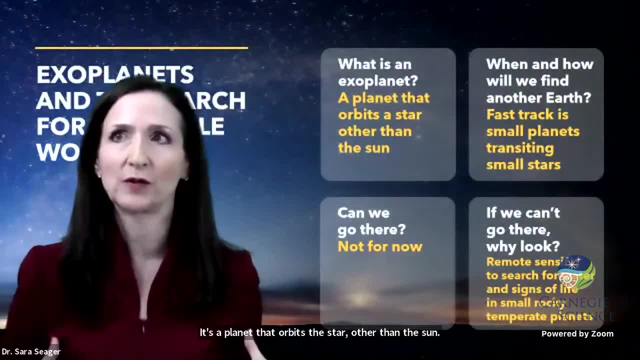 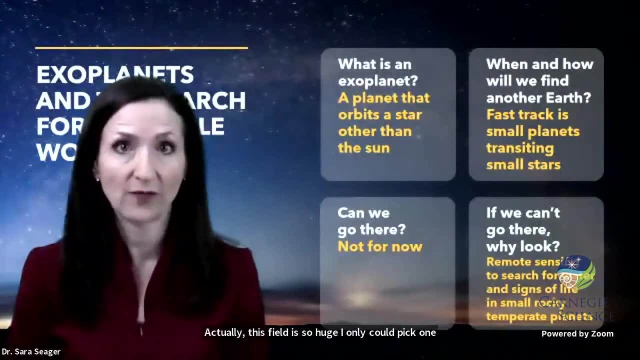 When and how will we find another earth? Actually, this field is so huge I only could pick one thing, And I picked the sort of nearest term way that we're going to find another earth. We're going to fast track By searching for and studying small planets transiting small stars. 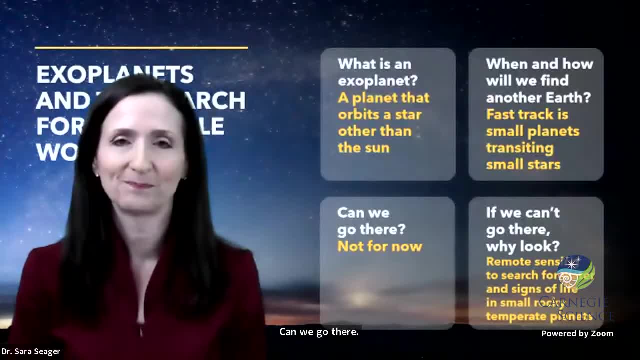 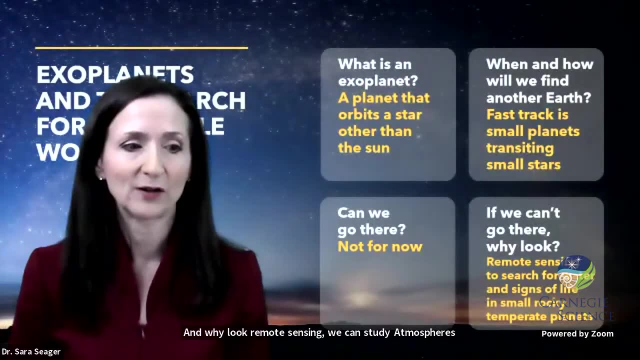 Can we go there? Not for now. And why look Remote sensing? We can study atmospheres from afar And search for signs of life. Well, that concludes my talk And thank you so much for your attention. Thank you, Sarah. 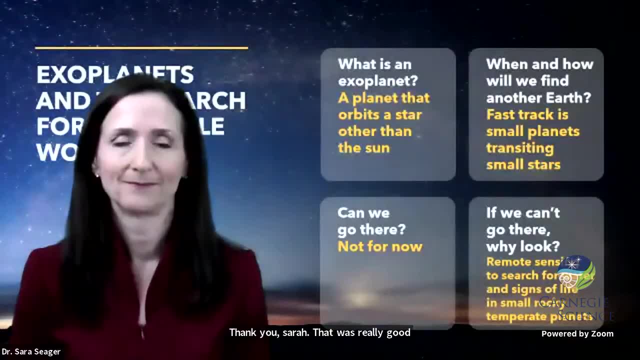 That was really, really terrific. That was fantastic. That was a lot of stuff And I think we've got a lot of great questions, So why don't we just dive right in? I'll try to address as many questions I can. 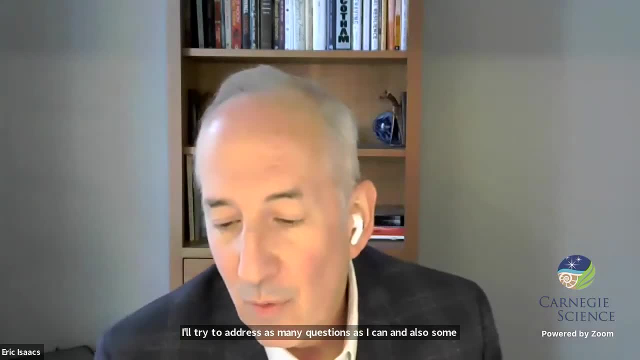 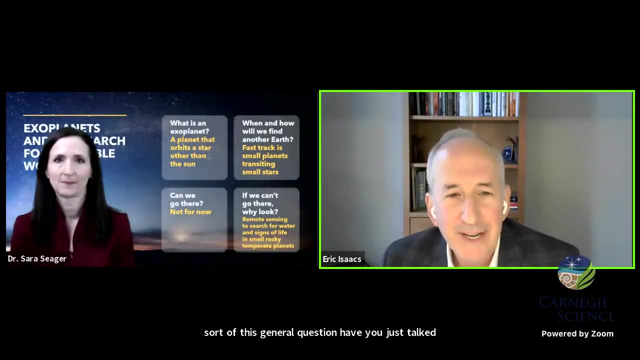 And also summarize some of them as we go through these. One is sort of this general question that you just talked about, Which is one of your areas of expertise, which is biosignatures. So maybe one way to ask this is if you were sitting on Trappist-1.. 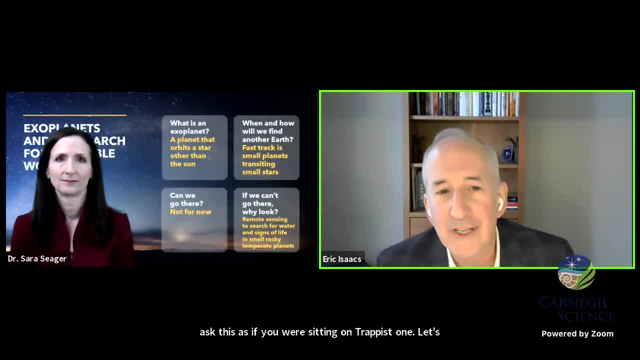 Let's assume that you could sit on Trappist-1 and looking back at earth. What would you see in our own atmosphere, Since we can measure that pretty much? What would you see that would help convince you as a planetary hunter, and a hunter for? 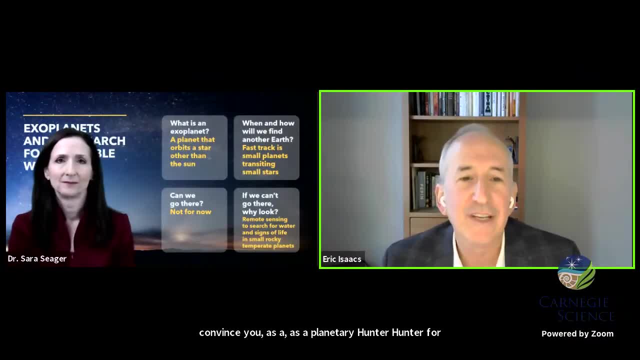 life on other planets, that there is life on earth, without actually getting to come here Because you just told us it's going to be hard to do it. So what would you see that would convince you? Well, first I'm going to answer a slightly different question. 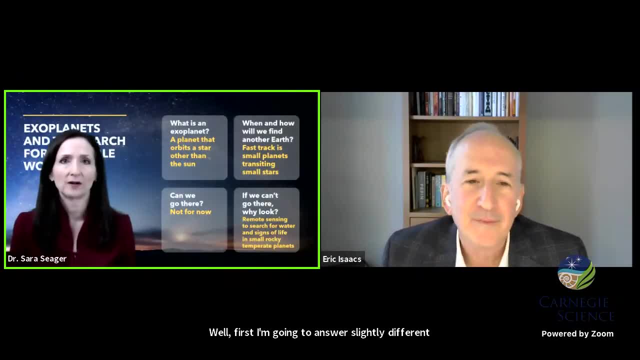 Okay, The main thing we'd see, believe it or not- is water vapor, And we'd see carbon dioxide. But water vapor is so important because on a small rocky planet it means there's a liquid water ocean, And that's important because we need a solvent for life. 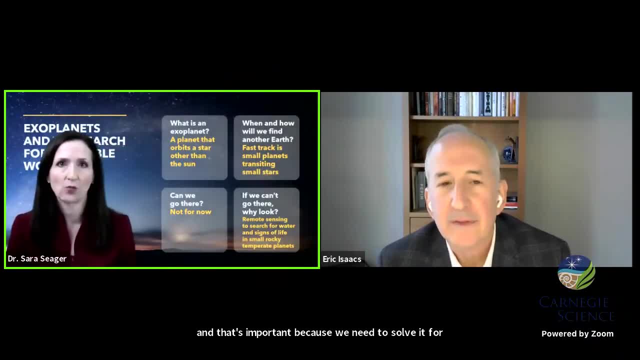 And water is the best one we know of anyway. So just even seeing water vapor we'd be excited Because we know we have what we call a habitable planet. For me personally, it's oxygen would be a huge tip-off And that's sort of. 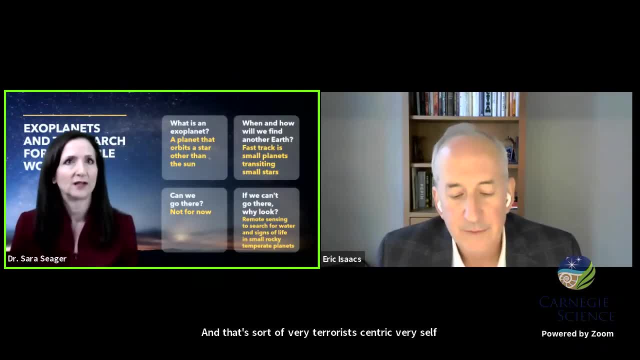 Very Terra-centric, Very self-centered, But really it's really a tough question Because with the tools, our wonderful next-generation telescopes, that's what we can see: Water vapor, oxygen, carbon dioxide And maybe a few other things. 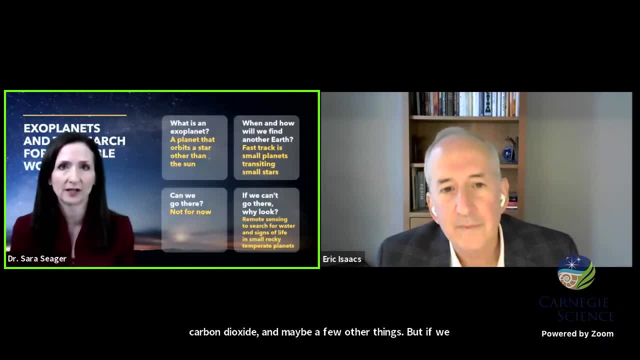 But if we could go further in the future, honestly it would probably be a pollutant like a chlorofluorocarbon, something so complicated and so energetically costly to make that we think it would have to be made by life. 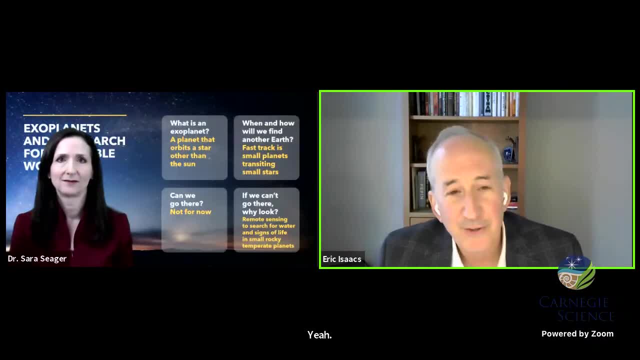 Yeah. So let me get a little more speculative here, because you did too. You talked a little about science fiction at the beginning and ended a little with science fiction, And the question has come up in a number of different ways, which is: we're looking, as you just said, we're looking for life like our own. 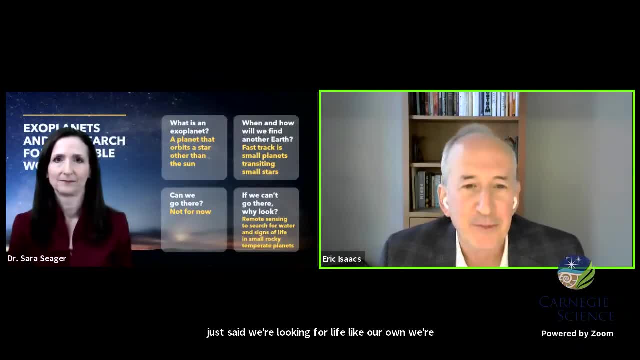 We're looking for carbon-based life that aspirates, that breathes, There's oxygen, there's carbon, there's carbon dioxide, carbon monoxide, photosynthesis, which creates it all. Is it even fair to start speculating that there might be an entirely different life? 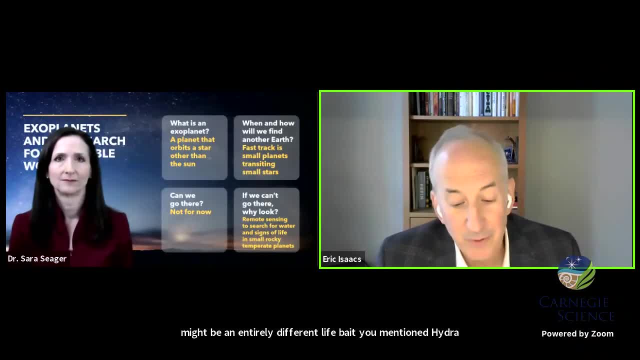 But you mentioned hydrogen and sulfur, These other types of things. I guess one way to ask it is: was George Lucas right in any way? He said he was right about multiple stellar systems. Could he have been right about some of the creatures he created? 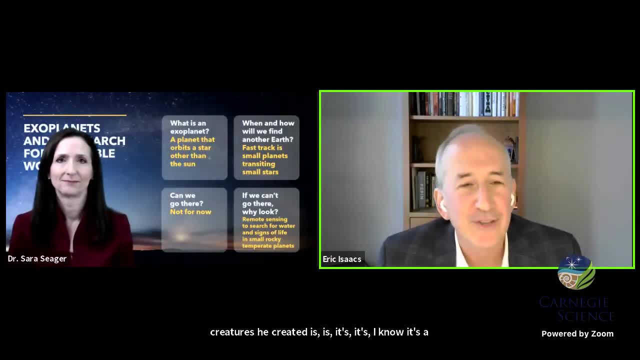 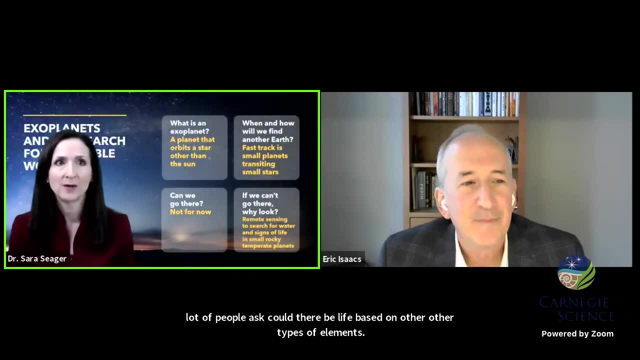 I know it's a speculation, but is there any sense in trying to do that? A lot of people asked: could there be life based on other types of elements? You know there might be And people haven't, you know. it's kind of beyond us to work out like a biochemistry. 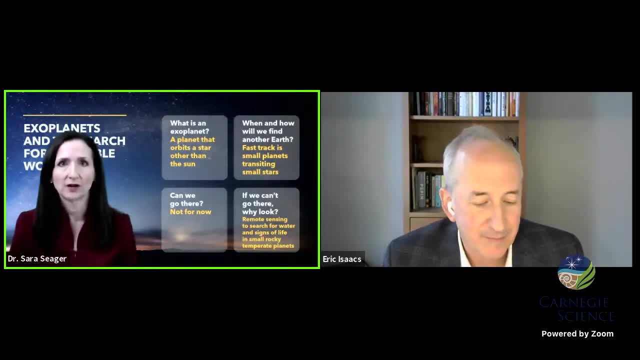 for different solvents or for life forms that are not based on carbon. So we're not really sure And in fact it may be kind of limiting. but you know, we are making the assumption that life uses chemistry like we do. 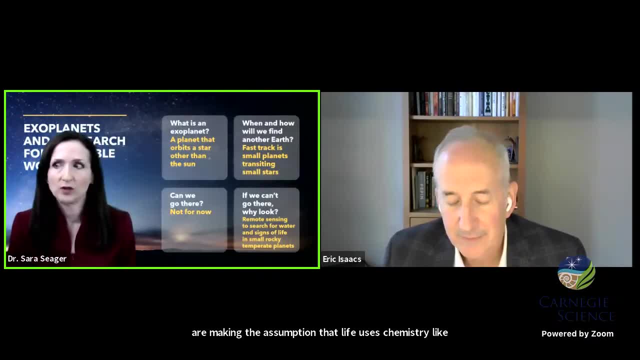 And all we can find are these gases that don't belong, And we don't know if we could ever trace that back to a life form of a certain kind. that's very different. So you know, we're quite limited just to find gases that don't belong. 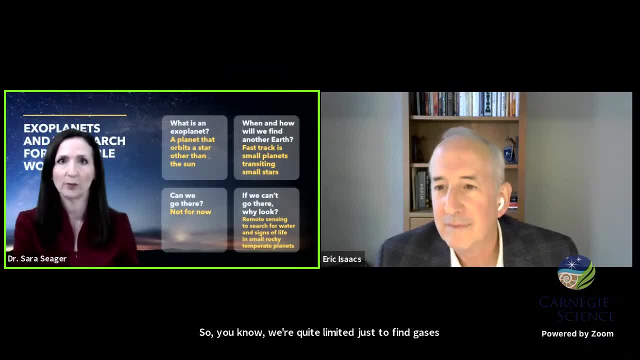 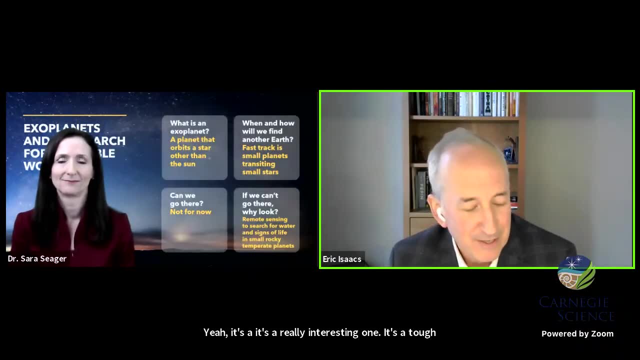 And if we find those, maybe it'll inspire people to think through these harder problems. Yeah, it's a really interesting one. It's a tough one, I guess, because it's a very complicated mix. Maybe a little bit more about the formation of planets. 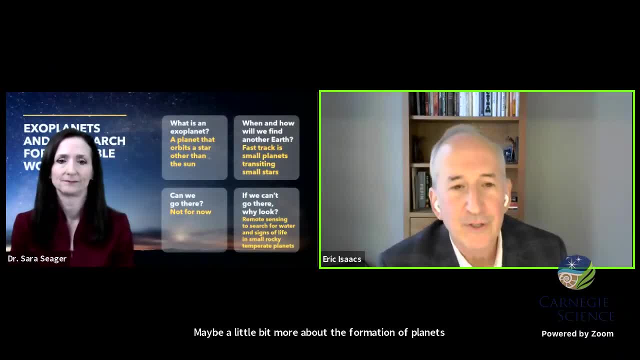 There were some people who noticed in your chart, your early chart, which showed the distribution of planets in various planetary systems, exoplanetary systems, that when you look, when you put the various solar system planets on that chart, they kind of look like outliers. 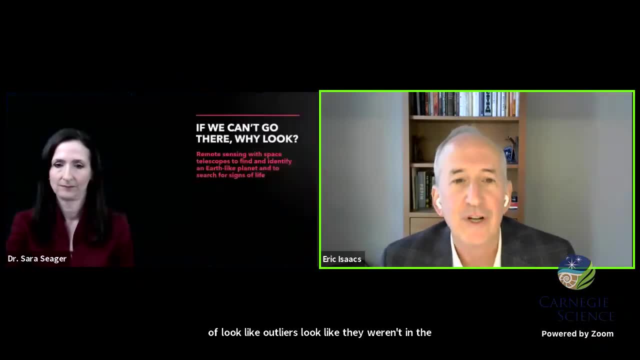 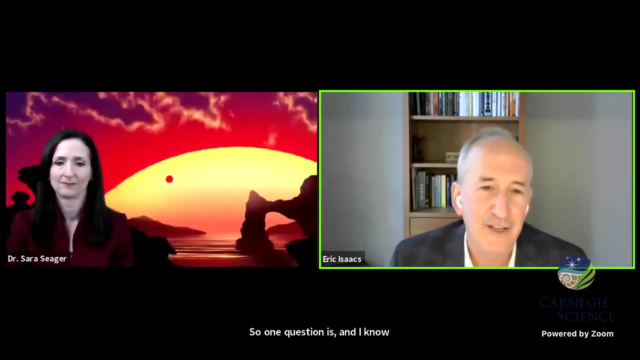 It looked like they weren't in the center of things. They weren't looking like the average architecture. So one question is- and I know you've thought about this- is: you know how unique is Earth's architecture? Are there other places? 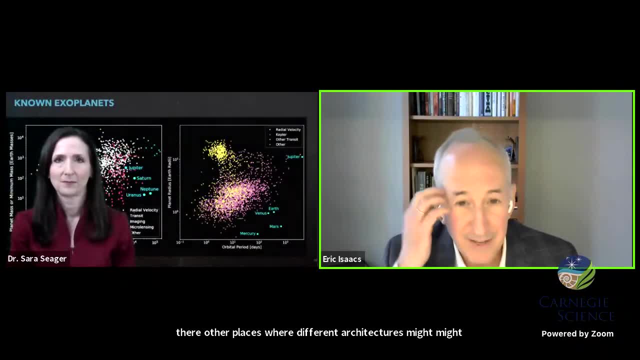 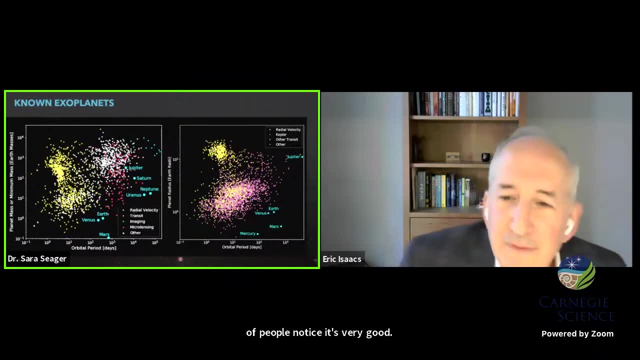 Where different architectures might sustain life. Yeah, this was the example, So it was a lot of people noticed. I'm glad they noticed it. Let's look at this plot on the right here. This is planet size versus orbital period And, wow, our planets are just not. they're all alone out there. 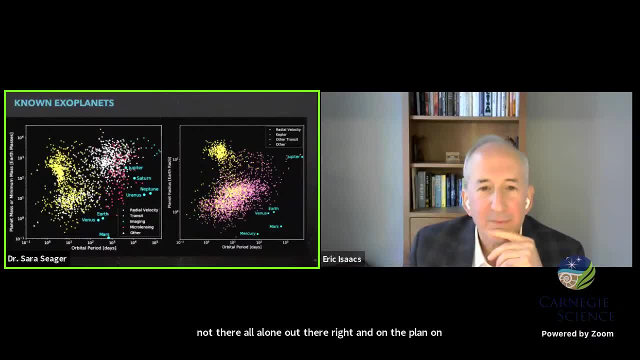 And on the planet on the left as well, And these are what we call log-log plots, So they're actually really compressed. So if we undid the logarithm, they'd be even more. Our solar system planets would be even more in the dark. 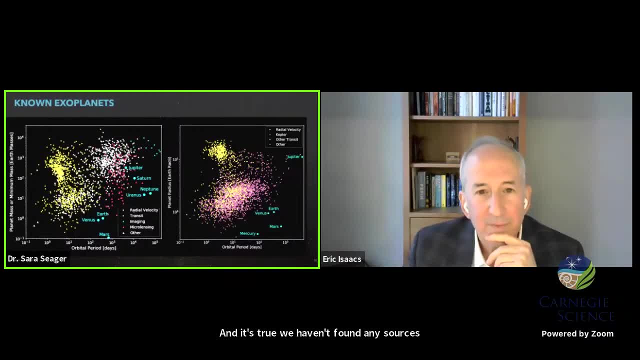 And it's true, We haven't found any solar system copies. You can see Jupiter on the left here. It's not totally alone. But wow, it turns out that, you know, our solar system is very hard to find. All of our techniques to find planets, they're all really quite weak in finding solar system. 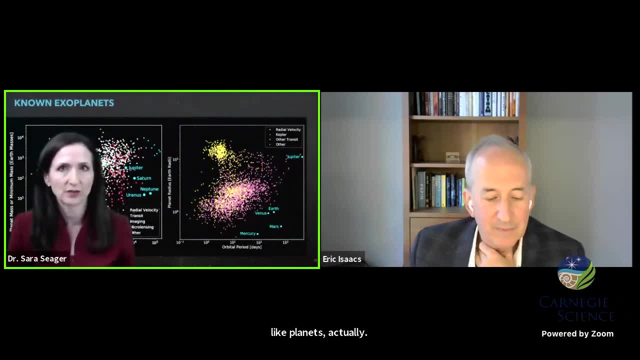 like planets actually. So we don't know how rare our solar system is. It could be as common as 5%, or a few to 5%, of stars have a solar system like ours, But it's not a very big number. 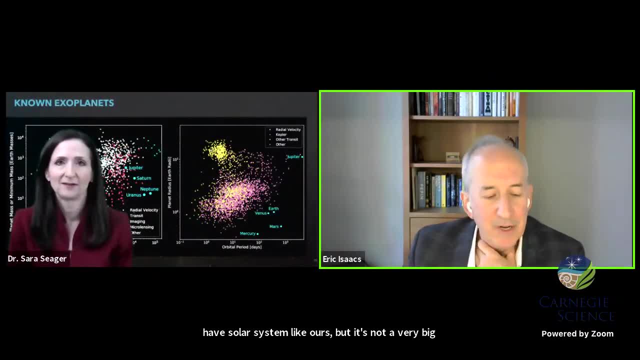 So it's very astute Of the person who asked that question. Yeah, I mean, could we? I mean the other other, some of the other things that have come up. are there biases in the way we're looking at things? 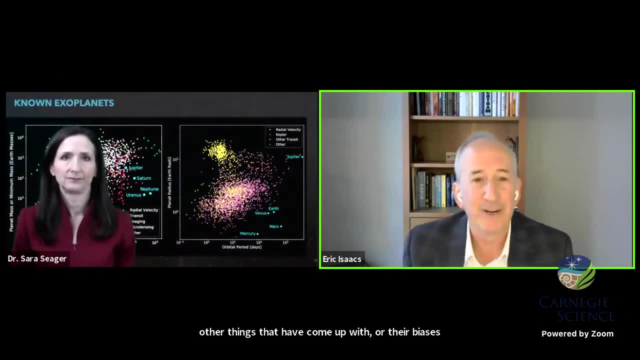 I mean, obviously you've already said right, You need the best thing is a small star and a big planet, And so that sort of does bias you right away in order to see whether it's, you know, radial velocity method or the transient method that you talked about. 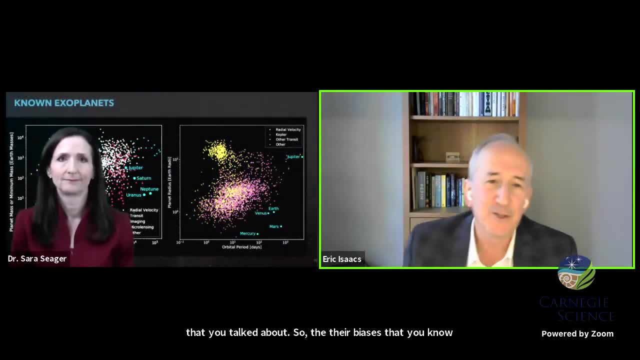 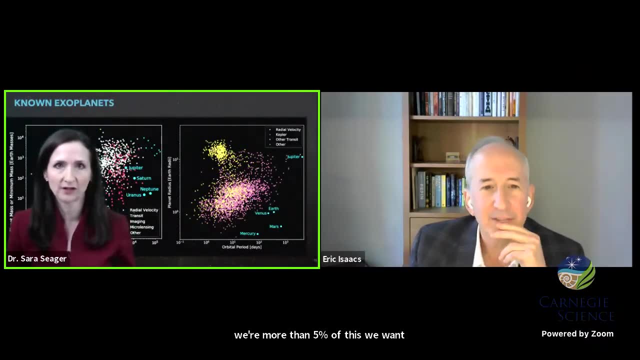 So are there biases that you know you can correct this chart with and say: oh yeah, we're more than 5% if you want to get this like that? In fact, this chart is extremely biased. There's no correction here. 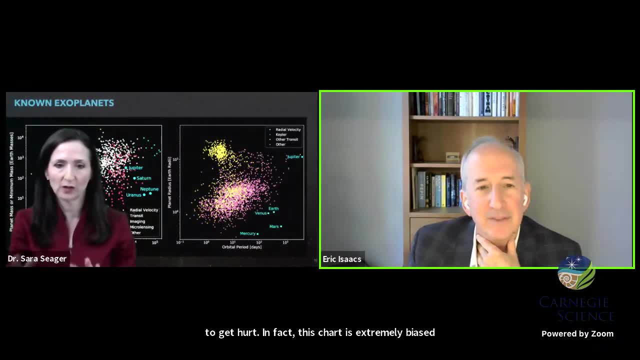 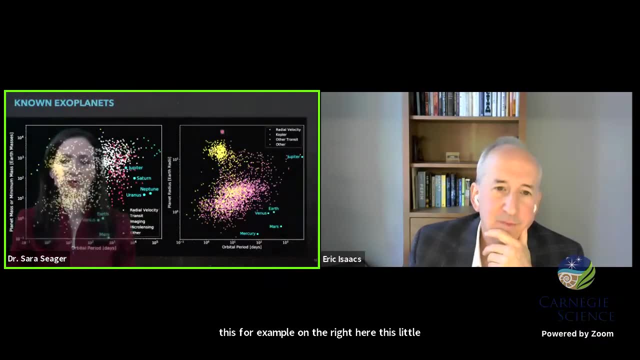 Yeah, For the bias and the technique. So if you want to look at the different clumps you know, don't do that because we haven't unbiased this- for example, on the right here, this little clump at the top, it's due to the 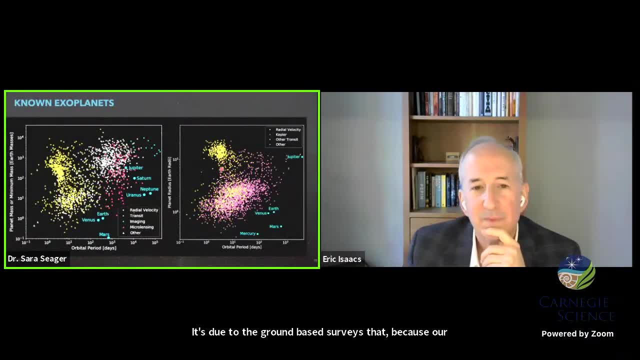 ground-based surveys. that because our atmosphere really kind of ruins our ability to make precise measurements in technique to find planets by planet size. So yeah, that's an artifact. We have so many biases. honestly, it's a great question, but I I couldn't even begin to. 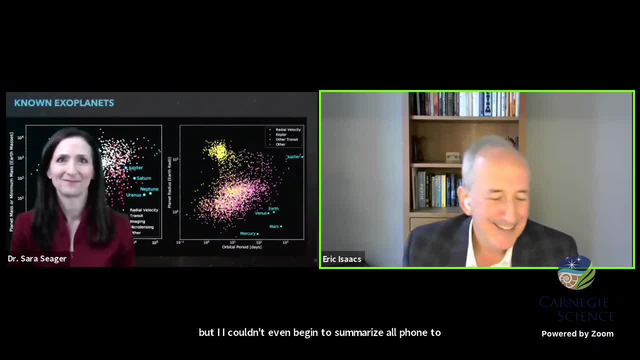 summarize all of them. Yeah, To undo the biases. Yeah, Yeah, I mean another. another thing that comes up is thinking about the habitable zone. So there's the zone- and you sort of talked a little bit about this- that it's preferred. 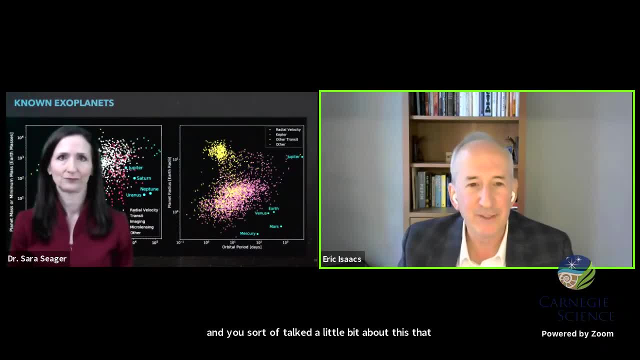 when we're looking for planets, that they exist within the right region, sort of the you know the snow line Right And and that they they because they need enough. you know life needs heat, means enough warmth. It needs energy. 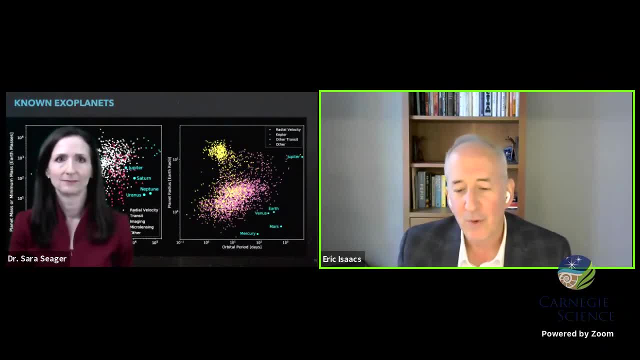 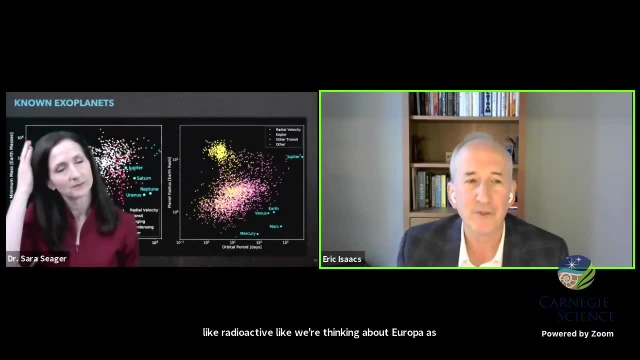 Ultimately, all of life on earth comes from the sun. So one question: are there other sources of heat, like like radioactive, like we're thinking about Europa as a possible place where there's life? are there other possible sources of heat that might trump the idea of having to be exactly in that habitable zone and maybe provide 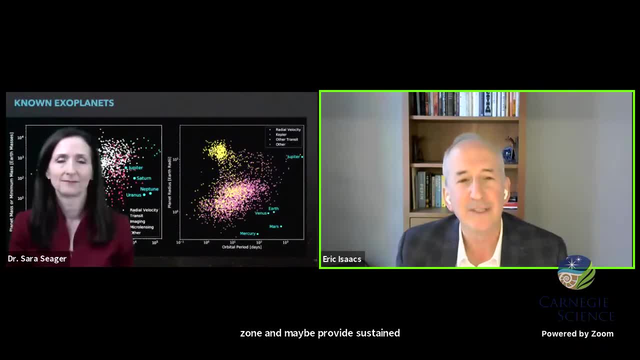 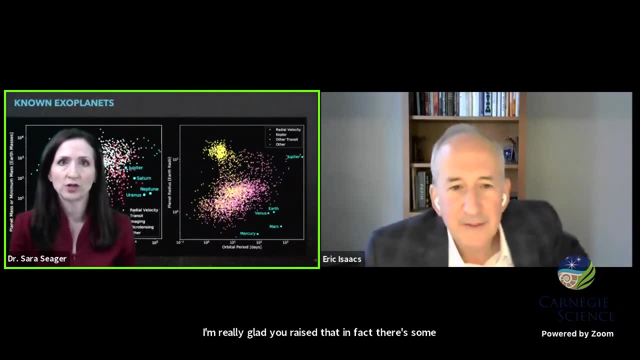 sustainability and for energy elsewhere in a in a system. Yeah, I'm really glad you raised that. In fact, there's some life on earth that doesn't use sunlight. There's life that lives at the bottom of the ocean, your hydrothermal vents. There's life on earth that exploits chemical potential, energy gradients, right? Imagine you have a ball on the top of a hill and you nudge it and it rolls down. They do that same thing by catalyzing Chemical reactions and they get energy. 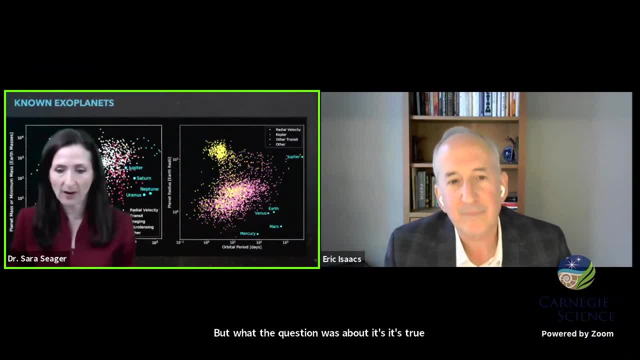 But what the question was about. it's, it's true We're here's another bias, because we're only looking for planets where life lives on the surface and is generating a lot of gases for an icy world Like like the example is in one of Jupiter's icy moons, scaled up as an exoplanet. No, we wouldn't be able to find signs of life there, because any life beneath these icy surface wouldn't gases, won't make it up. There's no atmosphere on the well, there's no atmosphere in those moons. So yeah, you know, we're really not. you know, imagine that there's life that doesn't use. 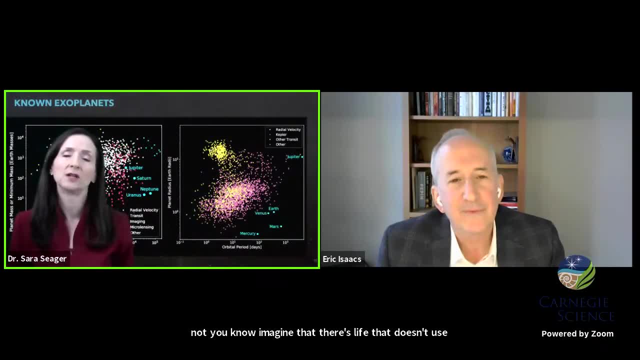 chemistry. perhaps there's mechanical life out there like our windmills, and perhaps they don't use chemistry to store energy And we couldn't find that kind of life at all. And one more thread on this is that I know that at Carnegie there's climate science and 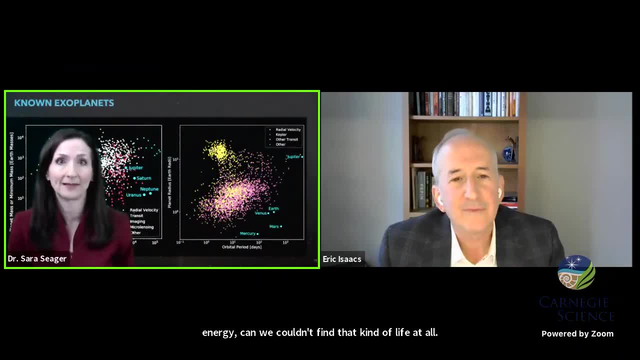 you know we're worried about a hundred. we're worried about like parts per million of carbon dioxide being added to our atmosphere. So now imagine another earth that has double the carbon dioxide you know just naturally, or 10 times more. 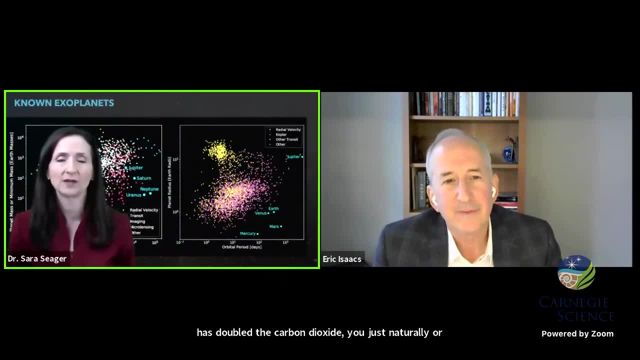 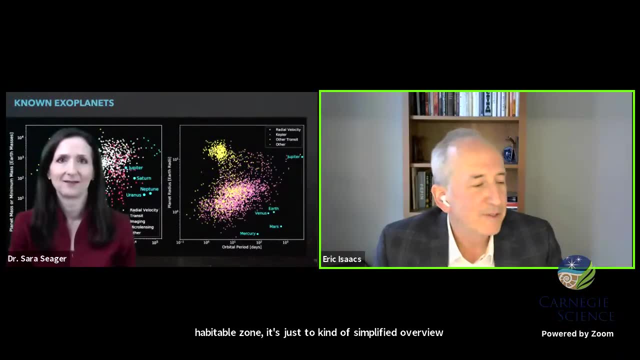 Yeah, So you know that atmosphere greenhouse effect really matters, And so it's true. the habitable zone, it's just a kind of simplified overview. Habitability is really planet specific. Yeah, That's really interesting. You know, one of the issues that comes up and I think we mentioned this before your 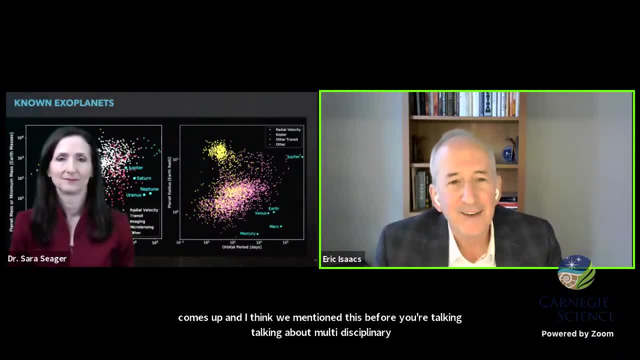 talk, talking about multidisciplinarity of this whole field, and you know what you're talking about. you, just in your talk, you know I think you probably whizzed through a bunch of different science sort of disciplines, from chemistry to biology, to you know the. 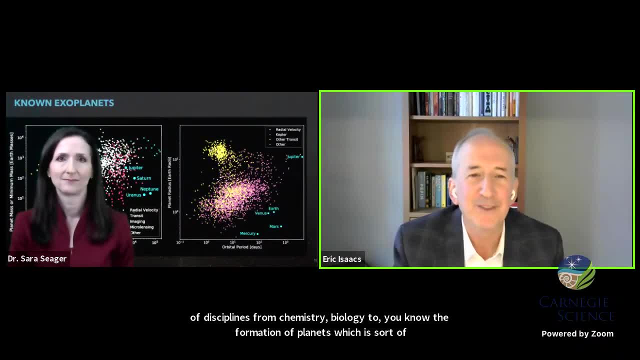 formation of plants, Which is sort of geoscience to astronomy by you know, using these techniques. Can you say a little bit about how you personally have trained to you know sort of stretch your mind into so many different areas that you have to combine just to do this kind of? 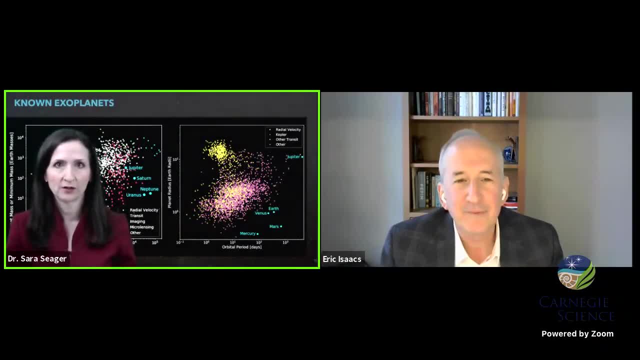 work Well, I love being on the frontier and I get bored easily, So those things helped me personally. but what also helped was having colleagues willing to talk, Like when I was at Carnegie. you know, the geophysical lab is right next door and I bugged. 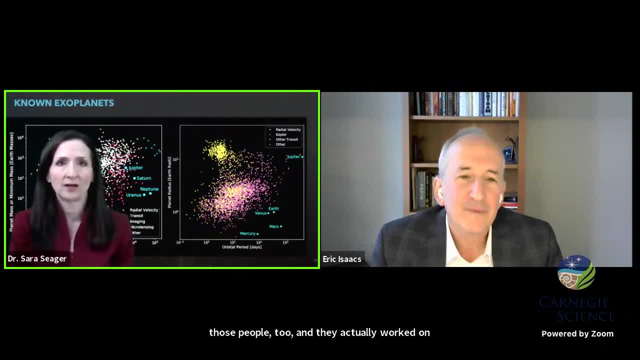 those people too, And they actually worked on asteroids. So I talked to one of the postdocs worked in biology. It took us like six months before we could actually have a conversation because we spoke a different language in our different sciences. And then I worked with the high pressure geophysics. 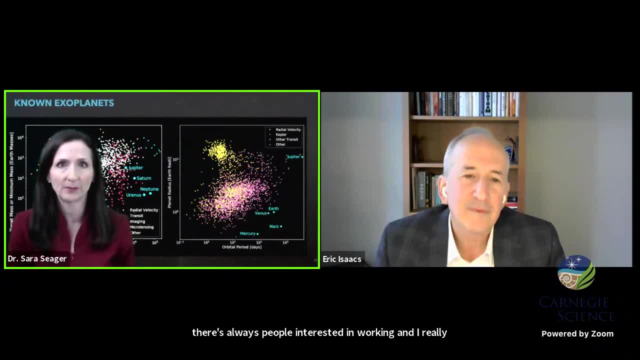 So there's always people interested in working and I really learned a lot from those people And then other things I do. I'm still working hard on chemistry and I have to go back and relearn, Like think about Eric for you, like what you learned in undergrad. 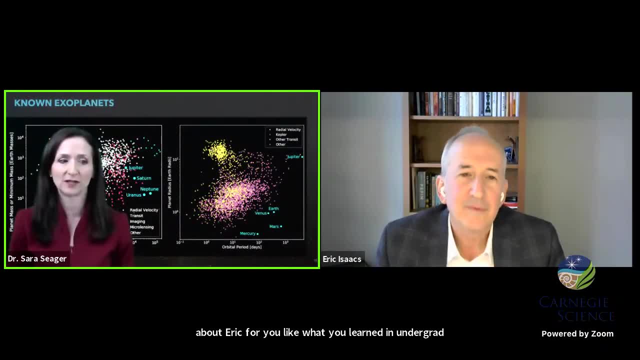 Like it's crazy, right? Maybe you took chemistry. I know you trained as a physicist, But if you took chemistry, you're going to be like, I'm going to be like, I'm going to be like- well then, I have to go back and review all of that and learn. 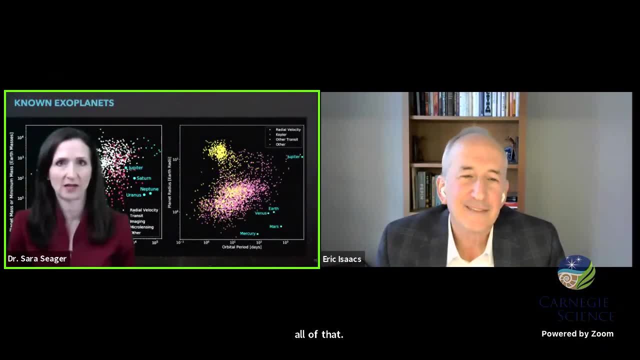 Like, I took organic chemistry as an undergraduate and it made zero sense. I don't even know how I passed. but now I actually understand parts of it because I, you know, put in the effort and the investment. So it's a mix of all those different things. 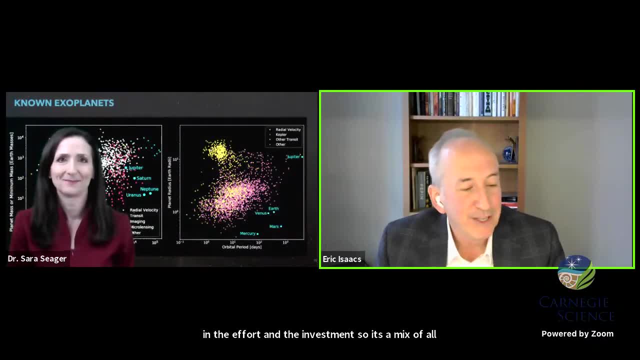 Yeah, Which makes it a lot of fun, I guess. So you know, so you must put all this together. So I guess one of the most important things you do is is you know you're trying to predict where to look. 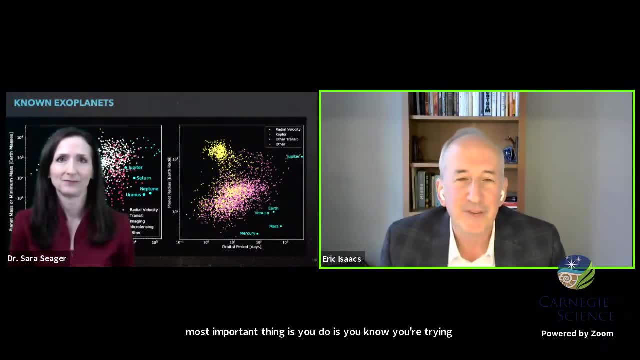 So how do you think about where to tell observationalists and yourself? I mean, when you think about you know? you mentioned James Webb, which is an incredibly exciting new development And, as you say they had just announced, in fact, Carnegie won three awards in this today. 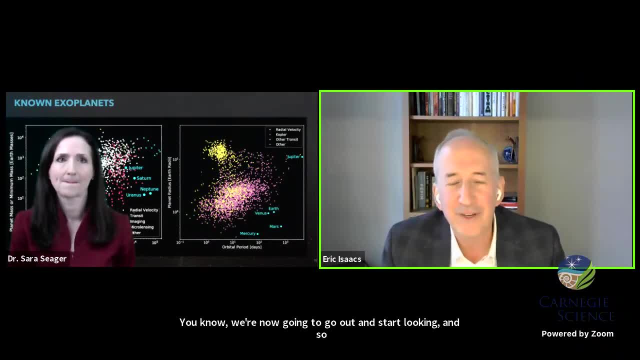 You know we're now going to go out and start looking, And so what would you say to an observationalist who has some time on the JWST? Where should they go Look? how would you even start to even think about that? 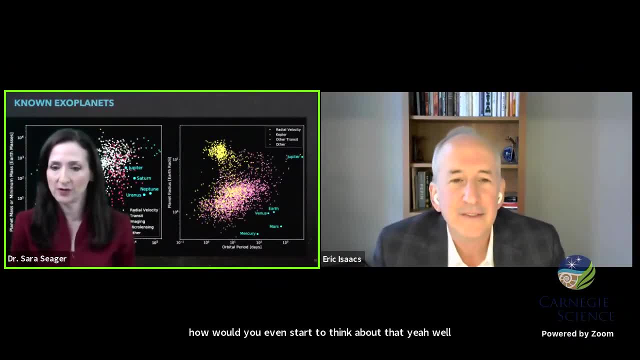 Yeah Well, you know it depends on the planet, and there's two ways to do this. One is look for this exact thing, And the other one is more like we call a fishing expedition, where you get observations, You have a reason, a motivation to get them, but you may find things that you 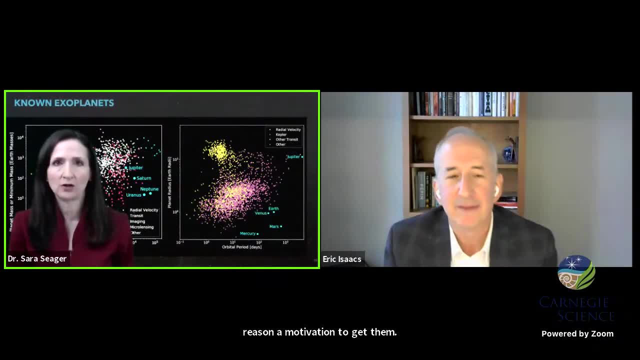 weren't looking for. So right now you know, it's really molecules strongly absorb in the near infrared where James Webb operates. I honestly, I mean I would just say like I don't think you can go wrong with any observation with the James Webb. 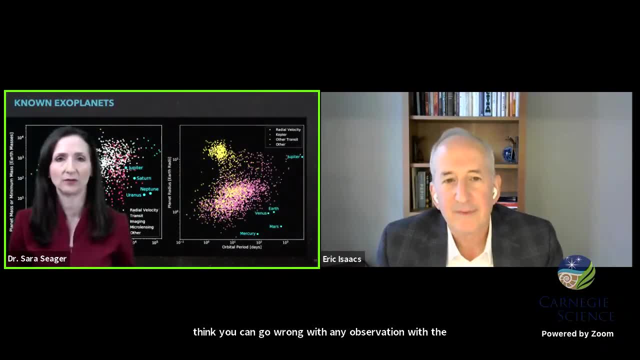 I mean, your proposal won't be selected in a competitive environment if you don't have a really good reason for motivating it. But I think it's just going to open up like a huge, huge discovery space. But there are specific things, like you know: the carbon bearing molecules, methane, carbon. 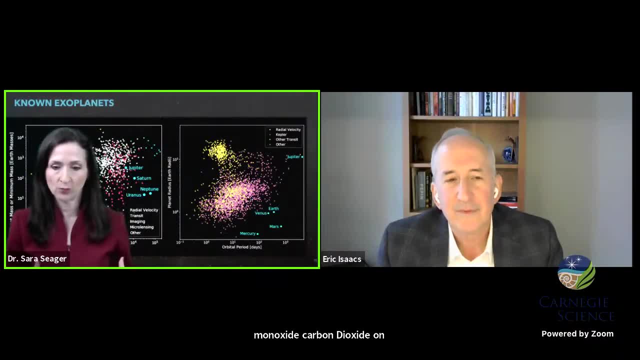 monoxide, carbon dioxide, On exoplanet- Yeah, Exoplanets on. We don't know exactly how those carbon will be distributed among those three. We think there's going to be some real clues as to atmospheric processes or atmospheric interiors and what they're releasing. 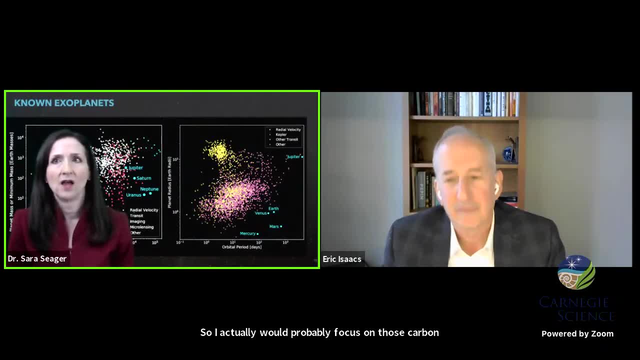 So I actually would probably focus on those carbon bearing gases. and also ammonia is one of my favorite gases because, yeah, yeah, it can be. and nitrogen, it can be in molecular nitrogen, like our earth has And you know. and two, it's a very strong triple bond or and can be pneumonia. 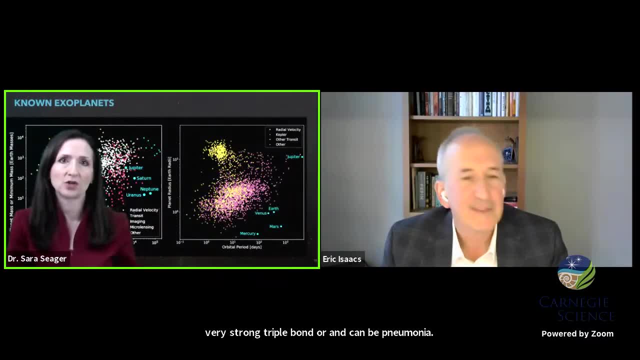 And it actually depends on the conditions whether the planet has an ocean or how much hydrogen it has. So I would tell them to go for those two sets- carbon bearing and nitrogen bearing molecules- because they have a whole lot of keys. We could go all night for this here. 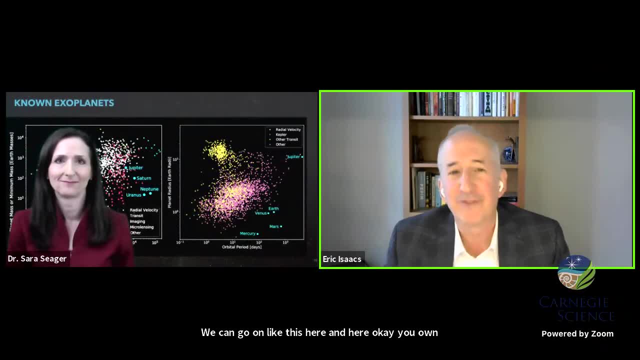 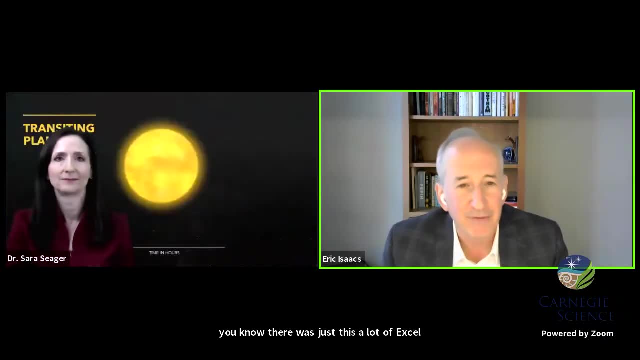 OK, you open the question of gases, So talk to us about phosphine. So you know, there was just this: a lot of excitement, maybe controversy, around the purported discovery of phosphine on Venus. You're involved in some programs there. 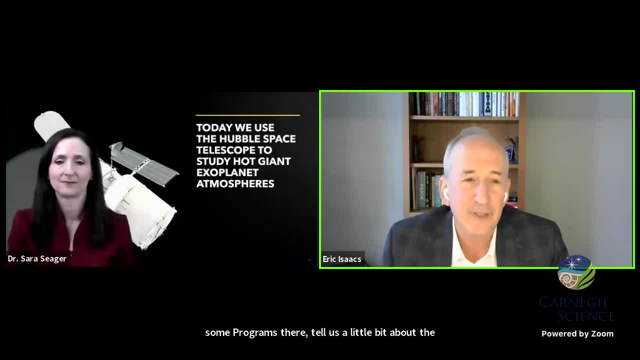 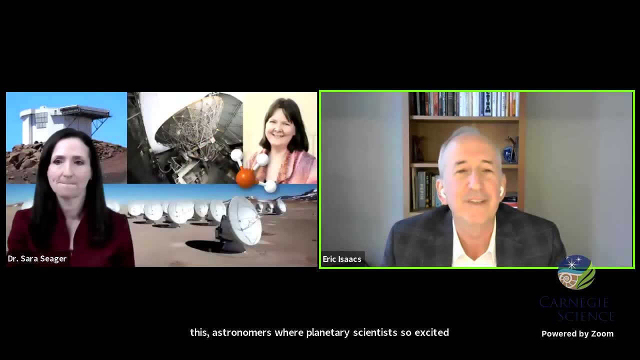 Tell us a little bit about the likelihood Of that being true? And if there is phosphine, what does that even mean? for why is it? why are astronomers or planetary scientists so excited about finding phosphine in Venus? Yeah, I have this little collage here, which which, because since I didn't have time to 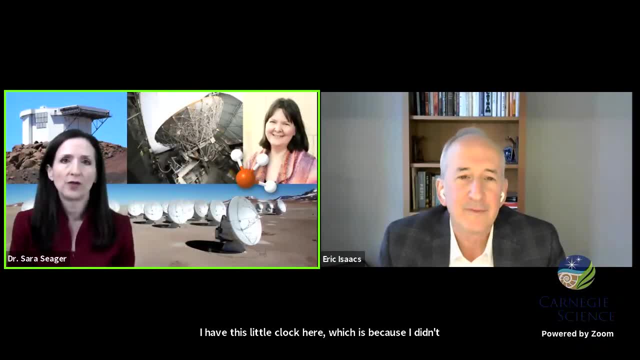 like squeeze this into my talk, but it turns out that on Earth, the gas phosphine, that's a phosphorus atom with three hydrogen atoms- It's actually only associated with life. It's either made by us humans, like as an insecticide kind of thing, or it's made by 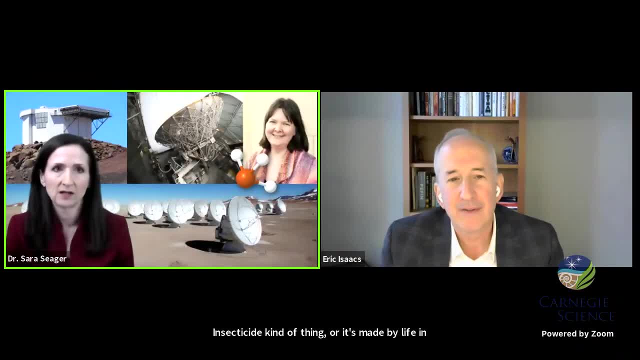 life in oxygen free environments Like wetlands or inside the guts of animals. And the story actually starts with Professor Jane Greaves from the UK, who remember how we were talking about how the line shifts between crazy and mainstream. Well, this idea was definitely on the crazy side because she purposely went out, wanted 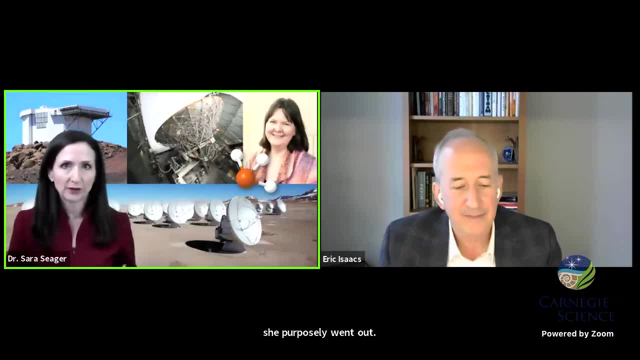 to search for signs of life on Venus, and she looked through the literature and she came across this gas, phosphine- And, by the way, my team had been working on phosphine for exoplanets and someone connected our two teams, So we got invited to join her work. 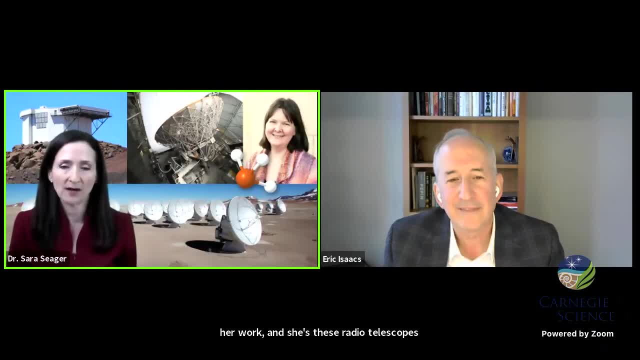 And she used these radio telescopes shown in these picture here: ALMA in Chile and the James Clerk Maxwell Telescope in Hawaii. And yes, she found a signal of phosphine on Venus. Now, Venus is too hot for any kind of life. 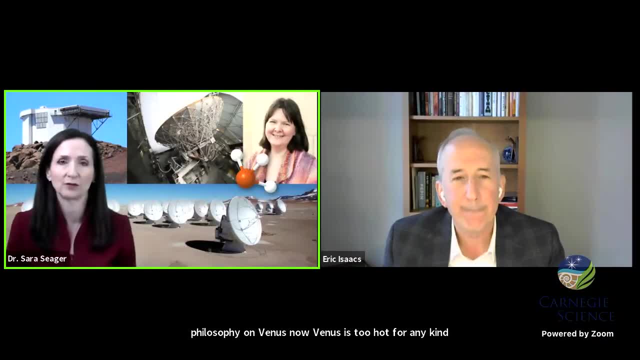 It has a massive greenhouse atmosphere- carbon dioxide greenhouse atmosphere- But up in the clouds of Venus, up away from the surface, it's much, much cooler And it is the right temperature for life actually. So she got her proposal eventually accepted and found a signal. 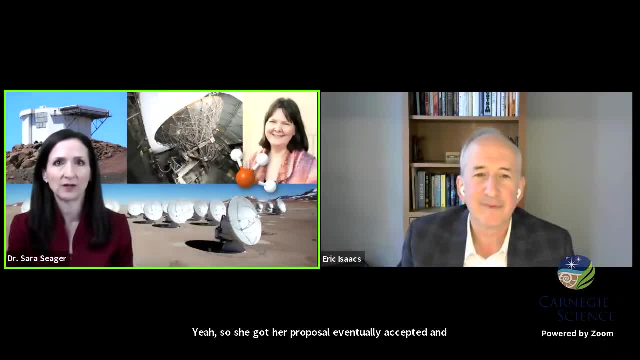 And it's incredible because There shouldn't be phosphine on Venus, Just like on Earth. there's very little hydrogen. The temperatures and pressures just don't favor phosphine. Now I just wanted you to know that this discovery made big waves and some negative 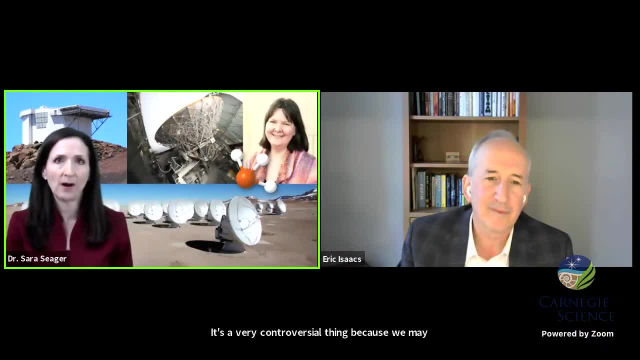 It's a very controversial thing because we make all our data public. It comes from these big shared national or international facilities And some other teams have analyzed the data and have not found a signal. You know other teams have analyzed it and have found a signal. 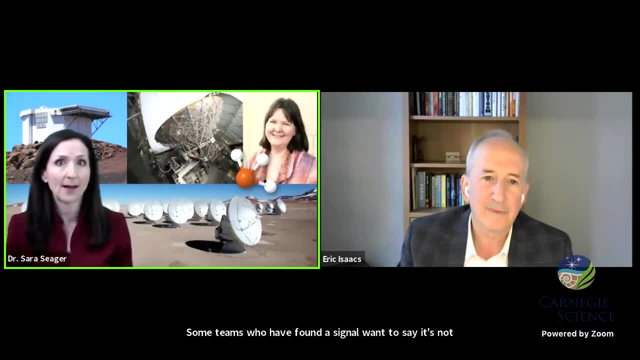 Some teams who have found a signal want to say it's not phosphine, It's a contaminating gas, It's sulfur dioxide, which our team stands by, our our signal, And we find that we need too much sulfur dioxide, like more than has ever been seen on Venus, to match it. 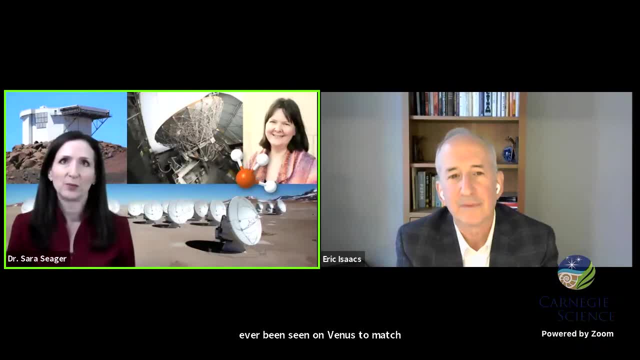 So this is still ongoing And it's kind of a like a beautiful, almost like real, like a- I don't want to say precursor to exoplanets, but kind of like a lesson learned. You know, we're looking for a tiny signal. 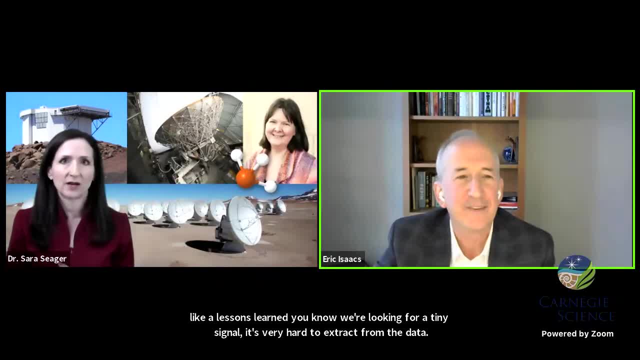 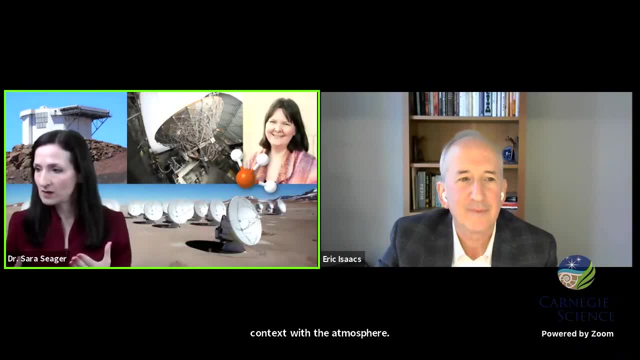 That's very hard, It's very hard to extract from the data. Yeah, we find a gas that really shouldn't be there in context with the atmosphere, And there's always- Yeah, there seems to always be a counter argument. So we'll just have to wait and see how this unfolds for exoplanets. 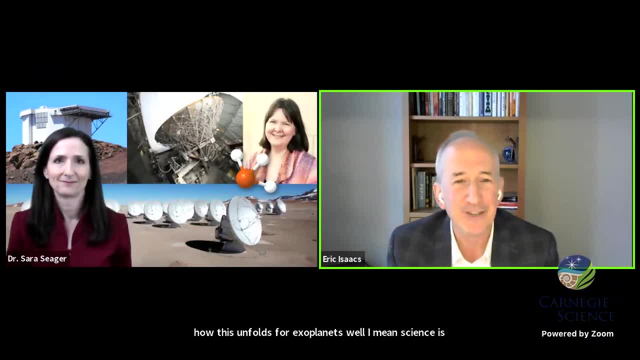 Well, I mean, science is working right. So controversy is good And, you know, challenging controversy is good, So it's a good. it's a good story and exciting. Of course, I was very excited when I saw it, but it's good to hear. 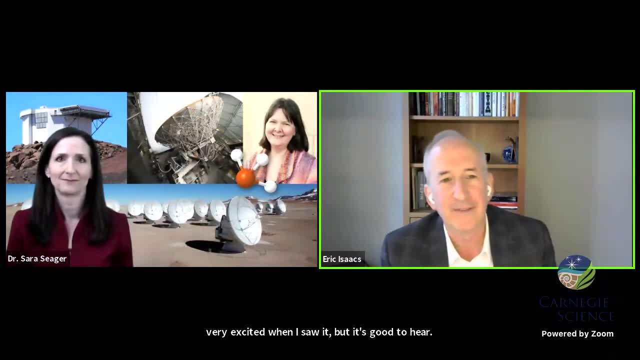 We don't have a lot of time. A few more questions maybe, But let's, let's move back to life, And you know we're going to talk a little bit more about what we're going to talk about, And you know this question of a biogenesis versus biogenesis. 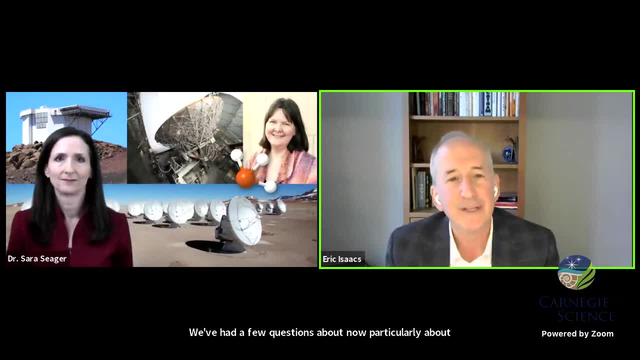 We've had a few questions about- not particularly about which it is, but about maybe this is related to the pandemic. One question starts off with: you know what if we, what if alien life came to Earth and we all got sick and died? 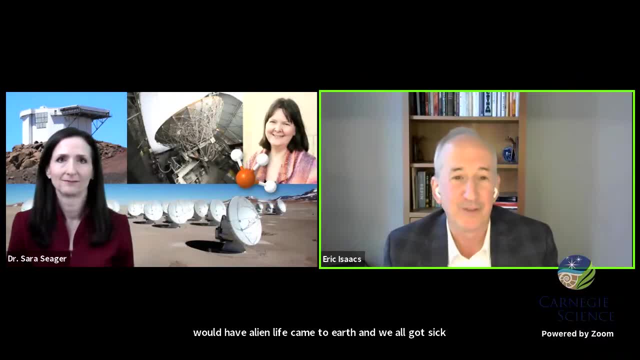 So there's obviously fewer pandemic, But but maybe- and it's an important question because you could imagine contamination. I mean, there are even theories. I've heard that that were actually, you know, some, some aliens landed on Earth, you know, a billion years ago with McDonald's. 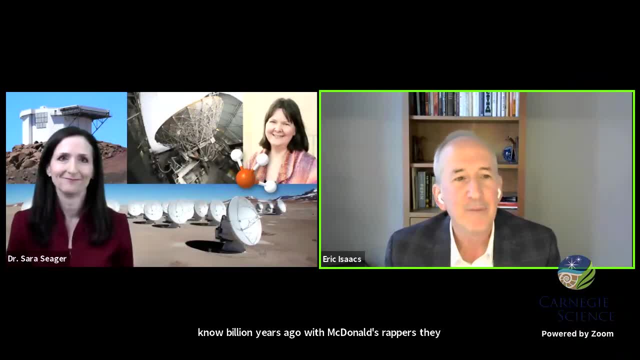 Right, Yeah, And then they were the, the descendants of that, And then we're the descendants of that. But can you say a little bit about your own? I mean, this is also real speculation. We really don't know how life started on Earth. whether you think it might be a biogenesis. 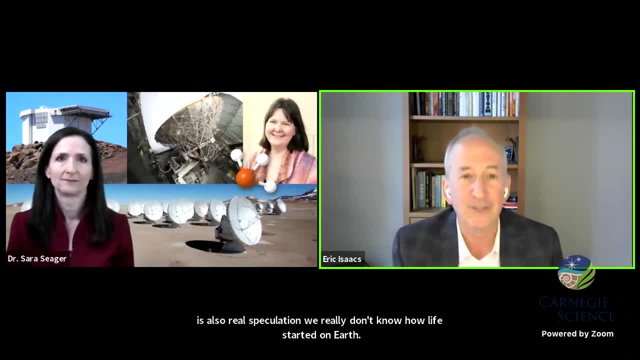 So something that actually started from simple molecules, like you're describing before, into complex lifelike molecules, or whether you think it might have come from somewhere else, which still pushes the question back somewhere else. it had to form Right, But right, right. 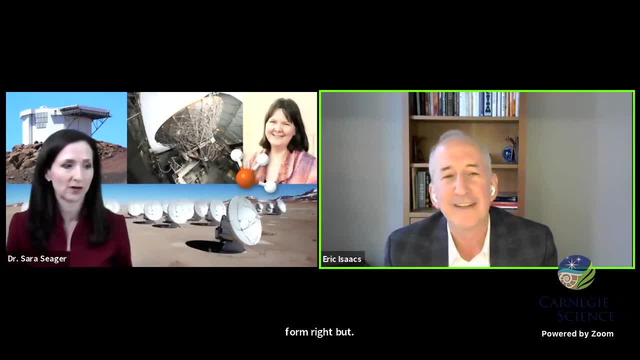 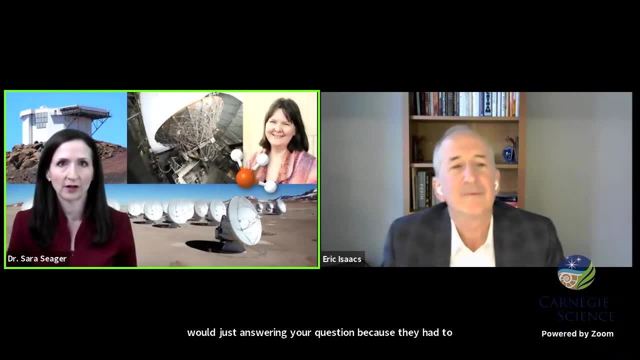 Right? No, I think there is sense. Yeah, I didn't answer it, but I think you've just Just answered the question, because it had to start somewhere. Yeah, And there's really no reason why it couldn't have started here, although we don't know. 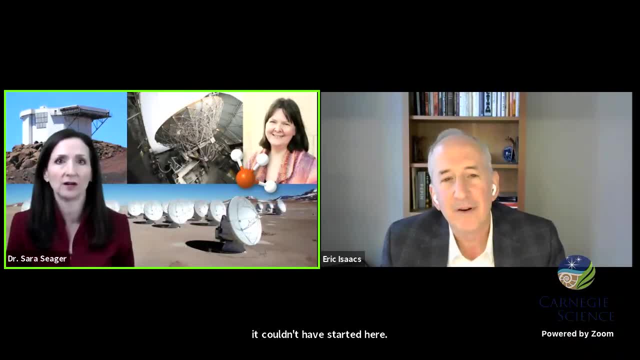 exactly how life originated. You know, we know all the ingredients for life are here, Right, You know we had some people favor that the ultraviolet radiation from our sun- like me, you know- was able to jumpstart some reactions and they have specific pathways that form. 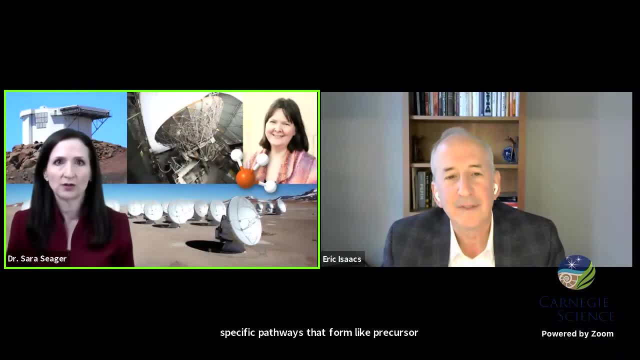 like precursor life molecules, And so there's actually more than one, you know, kind of competing theory about how life originated here. So I don't think we need to, you know, to go with that life came from elsewhere, And I agree with you that even if life did come from somewhere else, it still had to. 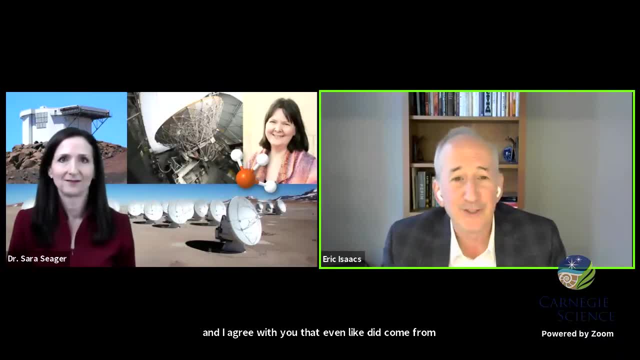 originate somewhere else. I think we probably need more investment in research that looks at a biogenesis. It's a tough problem And I know that a lot of people have been trying to do it for a long time. It's true, Let's see, we are coming to an end. 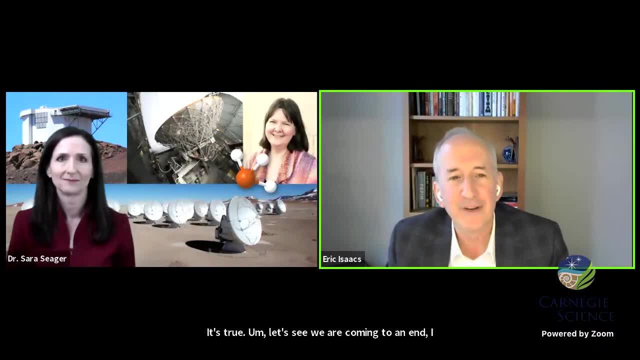 I don't want to keep you later than you have to be kept, but I think I'll end with. there are two things I went in with. One is a comment. We had a very nice note from somebody, and I'm going to give you their name because it's: 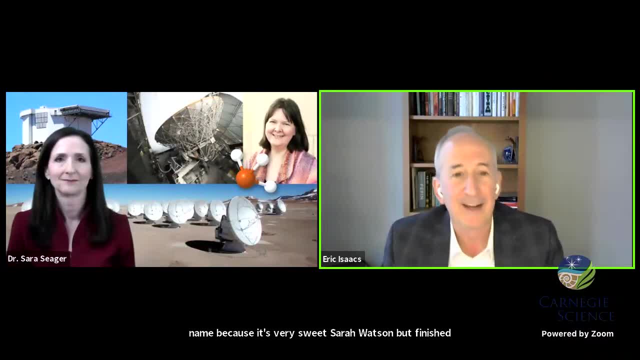 very sweet. Sarah Watson finished your memoir yesterday, Apparently in preparing for your talk today, And she really loved it. She thought it was beautiful and heartfelt. So thank you. Just so that you all know, Sarah Seager published a book, The Smallest Light in the Universe. 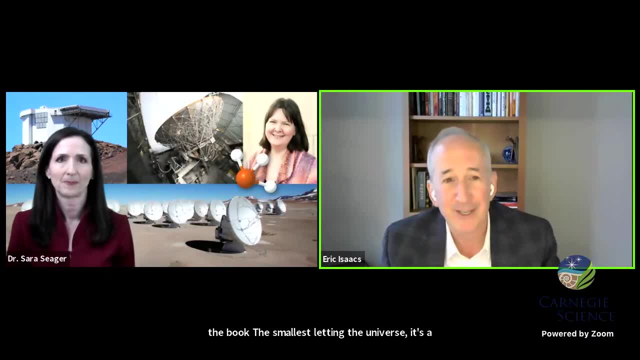 It's a memoir And this is not a book tour. She just gave a science talk but I'm giving her a little promotion here. But one of our- one of our audience members loved it And I just wanted to make sure that you knew that. she thought it was fantastic and really. 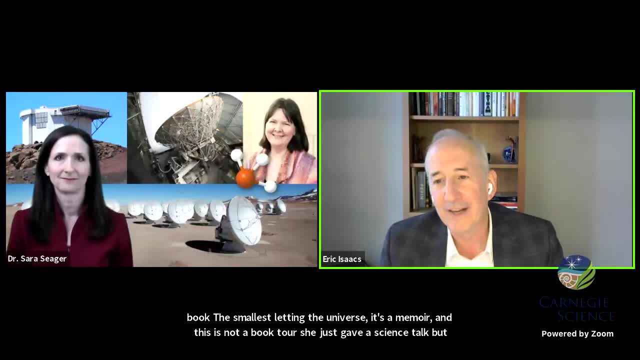 heartfelt. So let me end with what I think a lot of people are really interested in, and it's really totally philosophical. What a question. So what if we find life? What does that mean to us? You said how important it was. 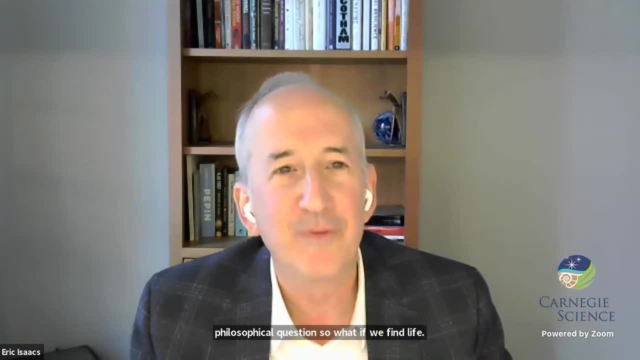 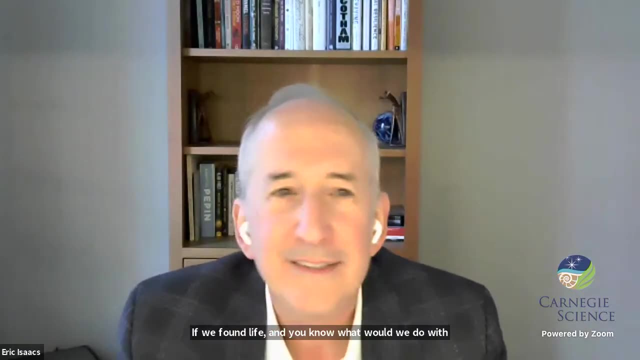 What would it, what would it really mean to us if we found life, And what would we do with that information? How would that affect people on Earth? I think really each person here, each person listening in, has their own answer to that, And I think it's a very, very individualistic question. 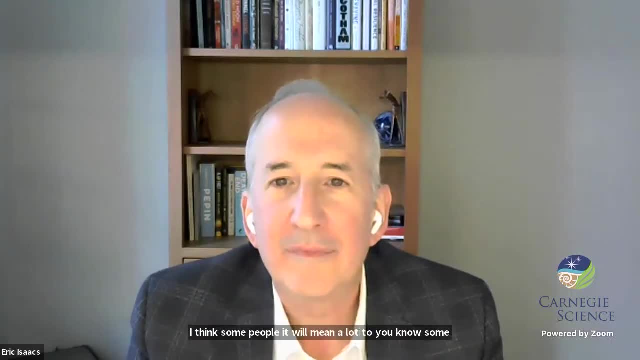 I think some people it'll mean a lot, to some religions There could only be life in one place and that will be really. it will be like a big seismic shift to adjust to that. For other people it won't matter at all really, because you know the everyday life. 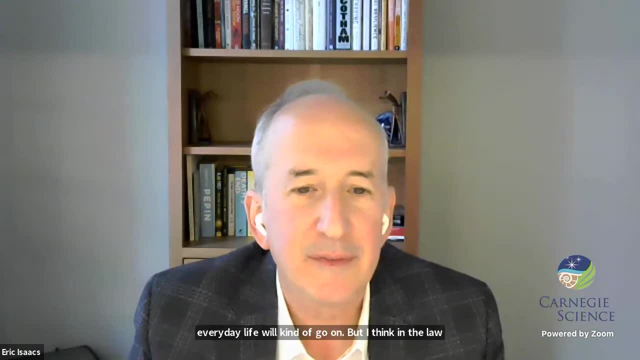 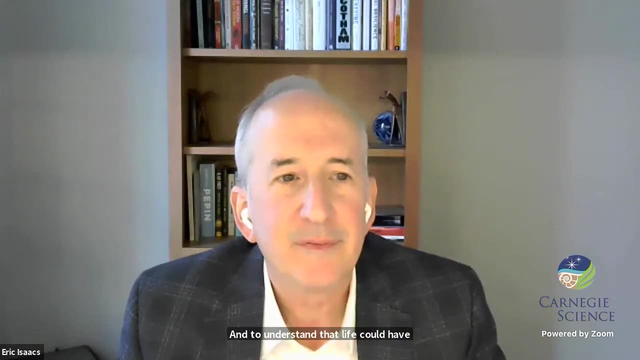 will kind of go on, But I think in the larger context, you know, it would be amazing to know we're not alone and to understand that life could originate elsewhere. It's kind of like, you know, we started out thinking that we, some of us- don't think this. 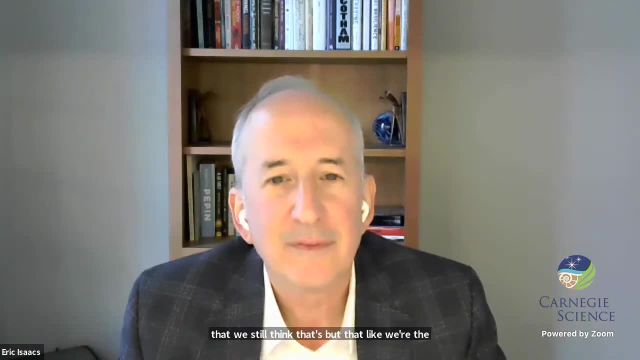 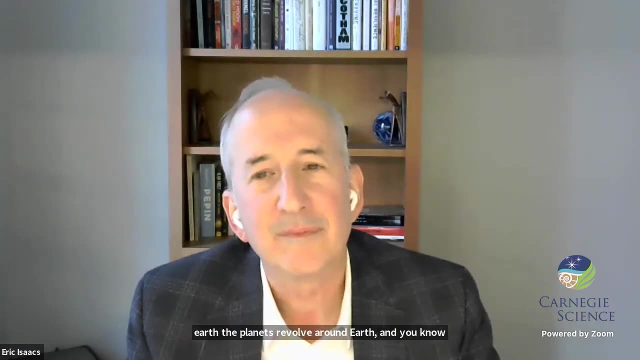 but that, like we're the center of the universe, We thought that, you know, the stars revolved around Earth, the planets revolved around Earth And you know, Copernicus came up with the theory and Galileo helped support it- that no, Our sun. actually everything's orbiting our sun, and later astronomers found that our sun is just but one of millions or billions of stars actually orbiting the center of a galaxy. And we later found that our galaxy is just one of untold numbers of galaxies. 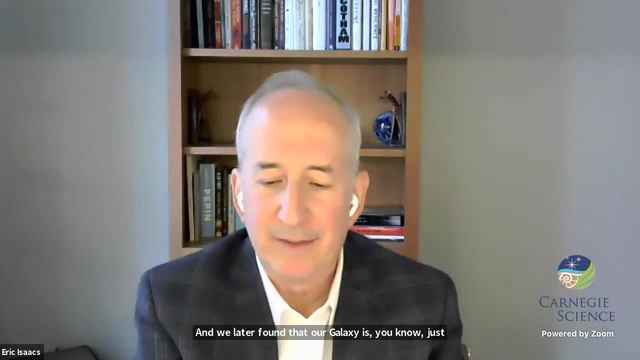 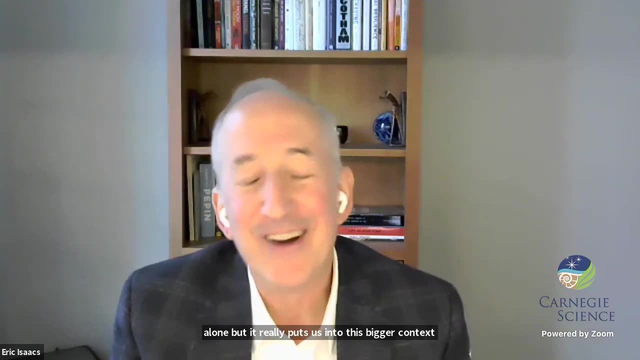 So in some ways, it'd be great to know we're not alone, but it really puts us into this bigger context And we like to call it completing the Copernican evolution. I think that's a great way to to finish up. 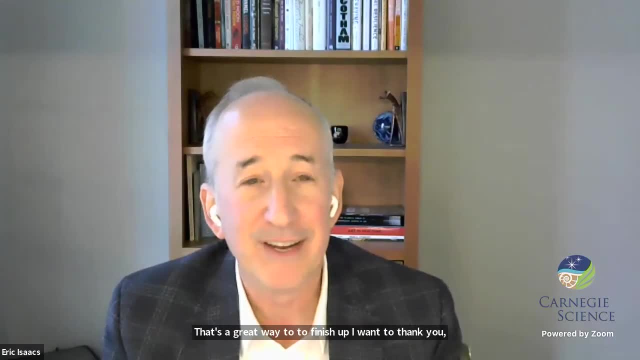 I want to thank you, Sarah, Sarah, for a really wonderful talk. We had a fantastic audience, Great questions. I'm sorry we can only get to a fraction of them. We'll share them all with you, Sarah, So you know what people are asking. 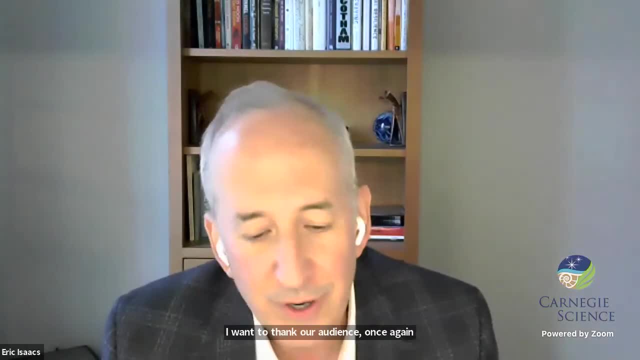 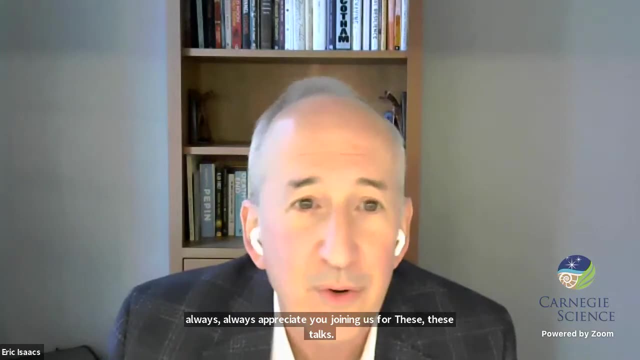 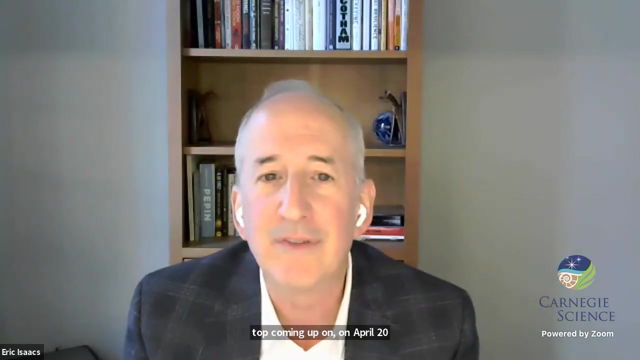 And I want to thank our audience once again for joining us Always, always appreciate you joining us for these, these talks We do have. I just wanted to quickly mention we have a talk coming up on on April 28th, our next Capital Science Evening with Dr.